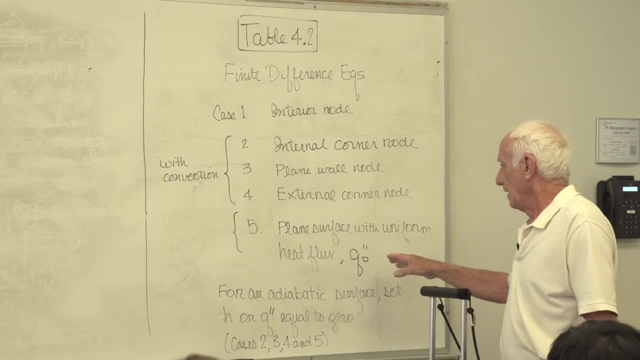 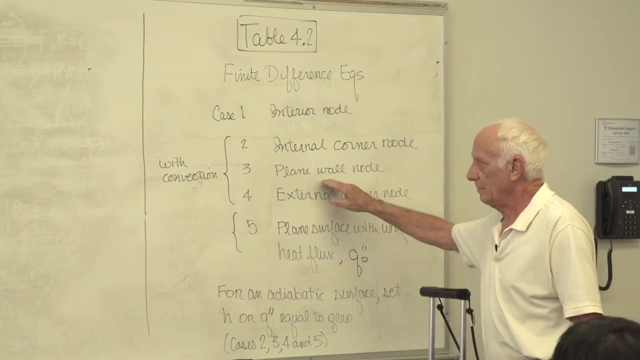 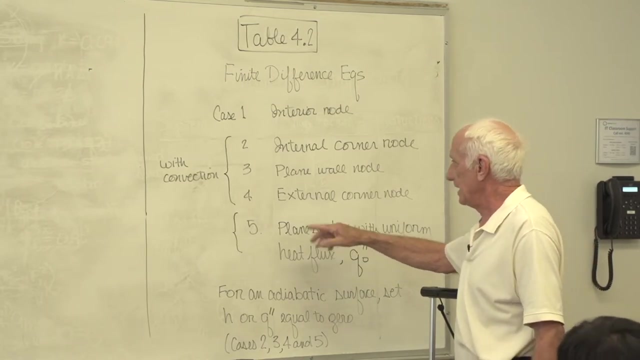 use to set a problem up with finite differences. Now, if this covers heat flux on a wall, convection on a wall, what about the case where it's an adiabatic wall? Okay, What you do there is you set h equal to zero in case 2,. 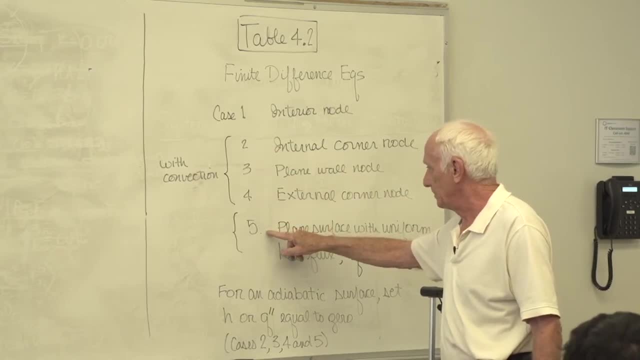 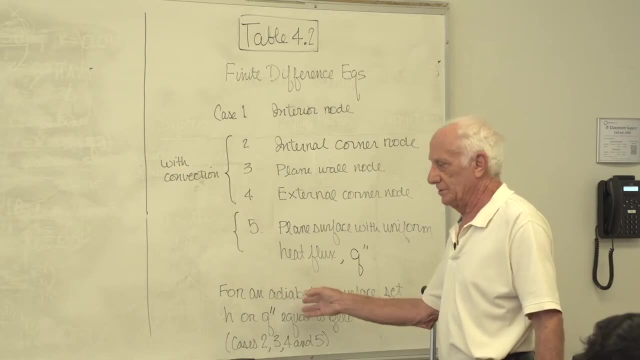 3, and 4, or you set q double prime equal to zero in case 5.. Let's just call that q double prime. We'll do that in just a minute. so an example problem. Okay, So we're going to work. an example problem. 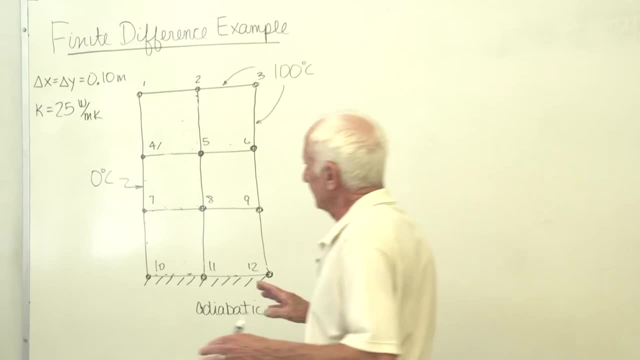 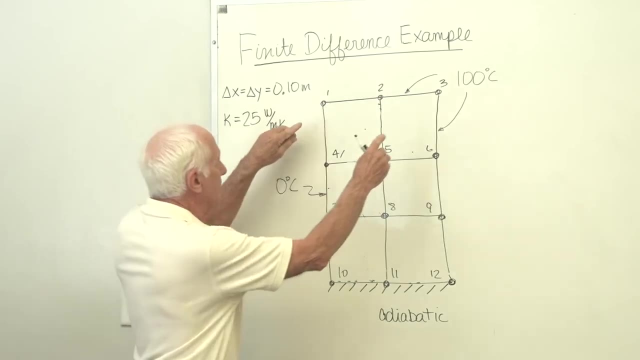 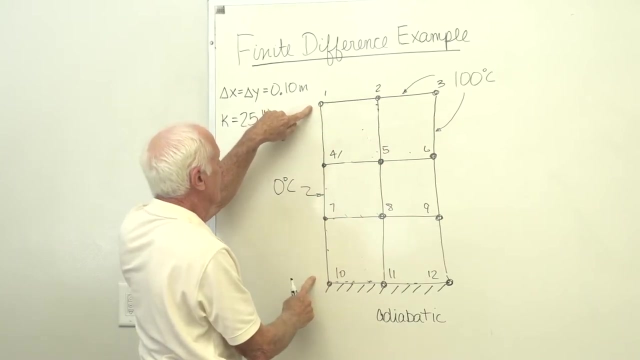 We're going to look at this plate. This is a plate whose thermal conductivity is 25.. We don't know how thick it is, but we do know it's 20 centimeters in this dimension and it's 30 centimeters in this dimension. 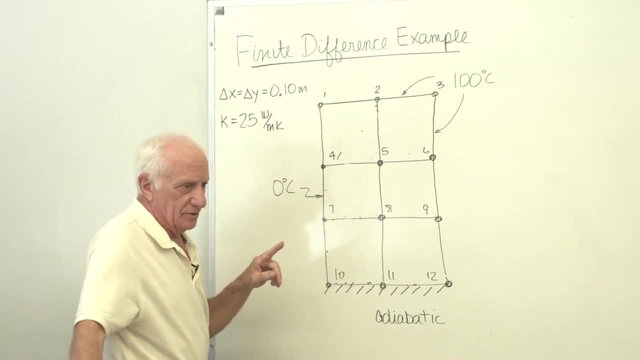 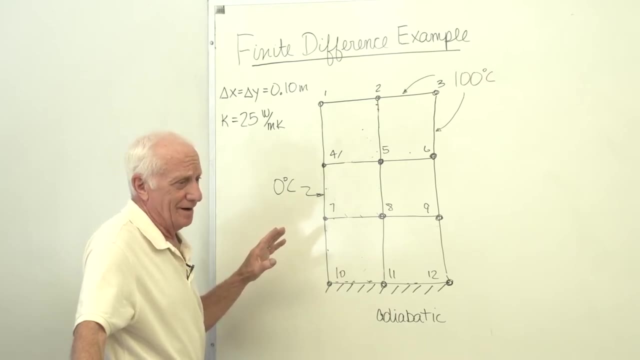 Our first goal is to set up a grid. So we're going to set up a really coarse grid, not one you want to do in the real world, but just to show you how the method works. So we're going to set a grid up of 10 centimeters. 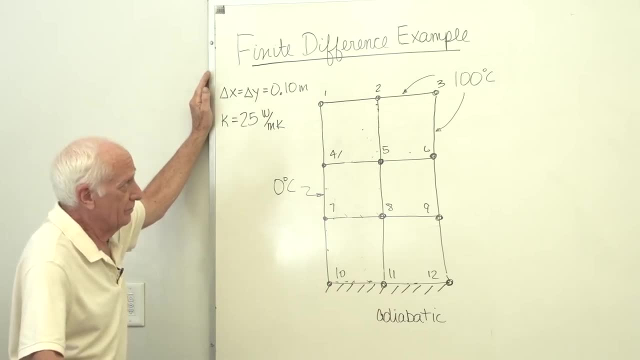 So you can see the nodal points, the big black dots. those are the nodal points of my grid. The left-hand side is kept at constant temperature- zero degrees C. The right-hand side is kept at a constant temperature- 100 degrees C. The top is kept at a constant temperature. 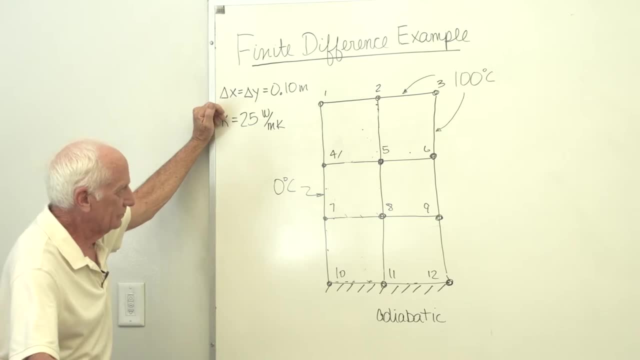 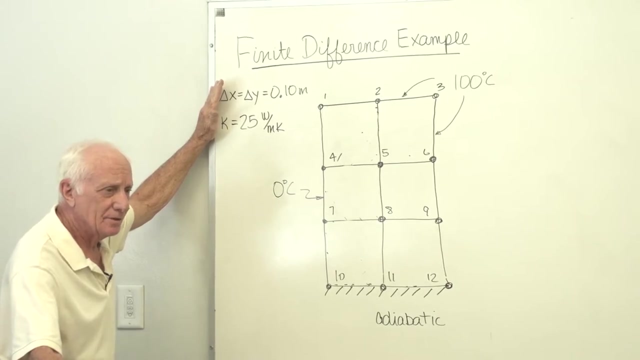 100 degrees C. Now I could, like I did last time we met, number the nodes M and N, M, column N, row, But that's too complicated for a simple grid like this, So I'm just going to number them. 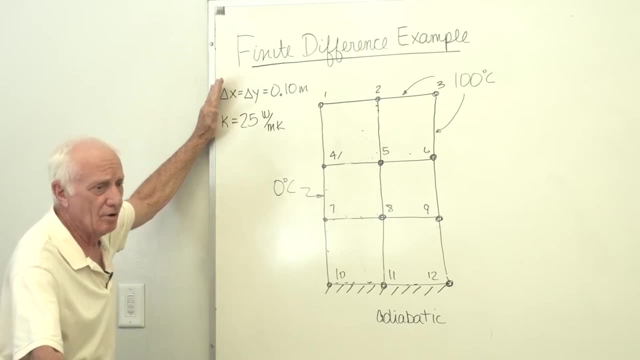 one through whatever. Well, if I had a 100 nodes, I'd use a double subscript, But for 12 nodes I'm going to just call them one through 12.. Node 1,, 2,, 3,, 4,, 5,, 6,, 7,, 8,, 9,, 10,, 11,, 12.. 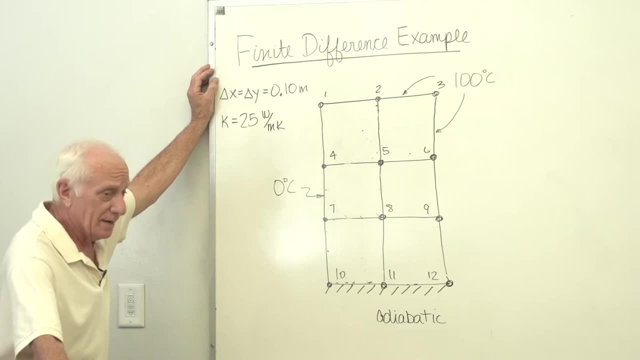 There they are. The bottom is adiabatic. Question to ask is: give me an estimate of the unknown nodal temperatures? Give me an estimate of the heat transfer Q. Let's start out with getting the temperatures Now, some temperatures I know, by the way. there are 12 total nodes. I know T2 equal T3, T6, T9, T12 equal 100 degrees. I know T4, T7, T10, Zero degrees, unknown T5, T8, T11.. 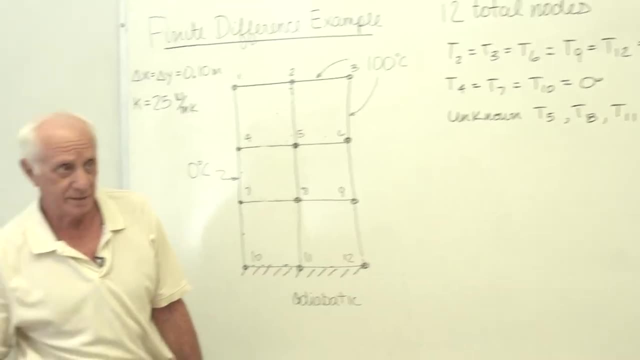 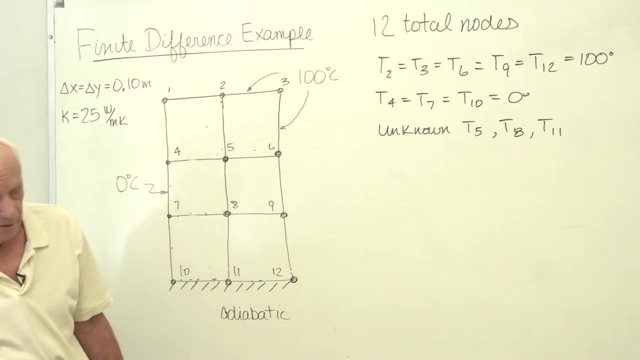 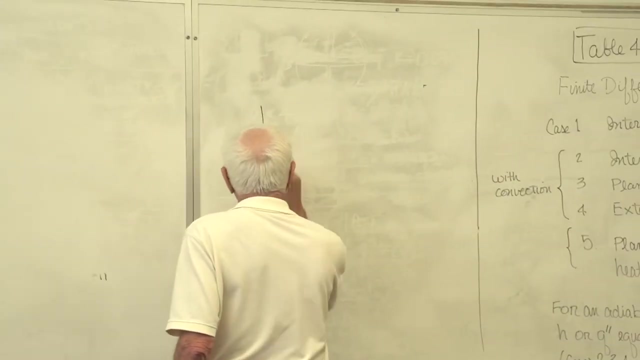 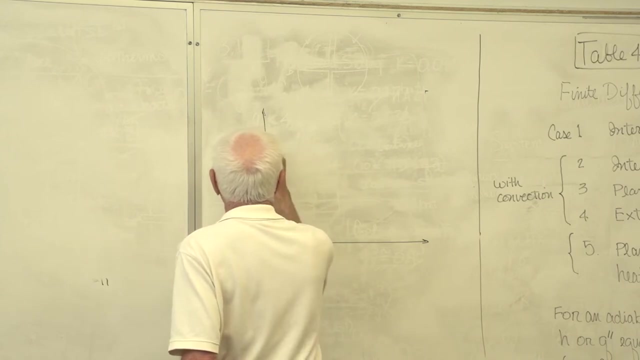 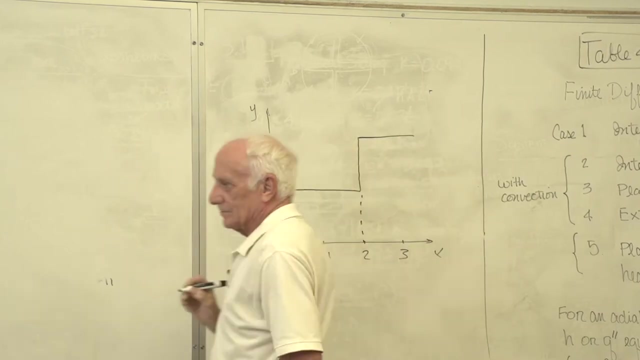 So that's what we're supposed to find Those guys? Yes, sir, T1.. T1, yeah, T1.. Here's a game you can play with your non-engineering friends, okay. So you ask him okay. 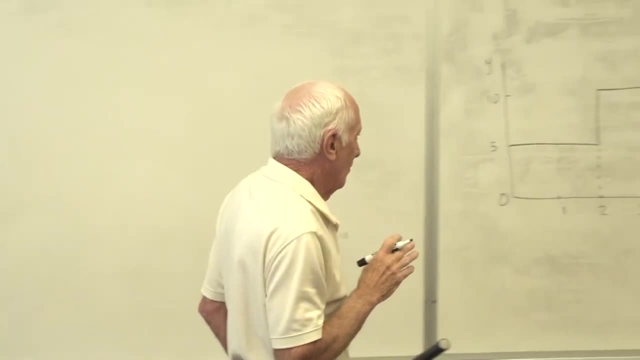 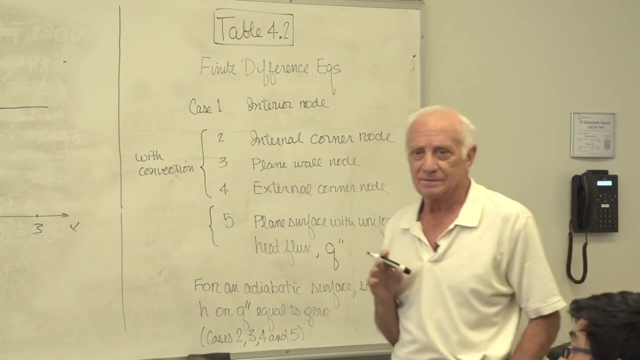 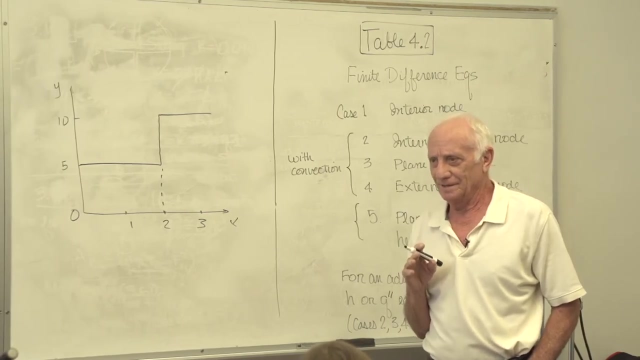 now why don't you give me your best guess? When x equal to what is y, Half the guys say 10, half the guys say five. Wait a minute. Somebody's right and somebody's wrong. No, they're both wrong, that's okay. 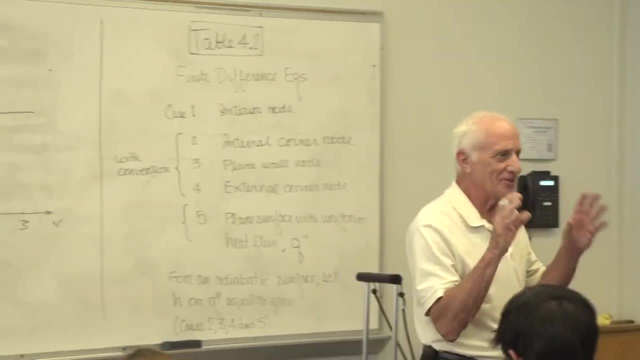 You can't ask that question Illegal. don't ask me. It was a good question. Thanks for asking, Otherwise I wouldn't have done that. I'm glad you asked, But no illegal question don't ask me. I don't know and I can't. 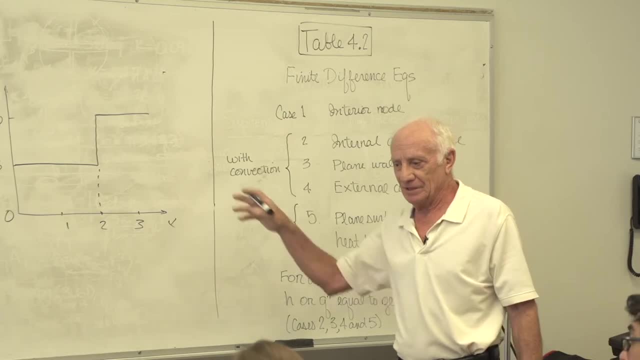 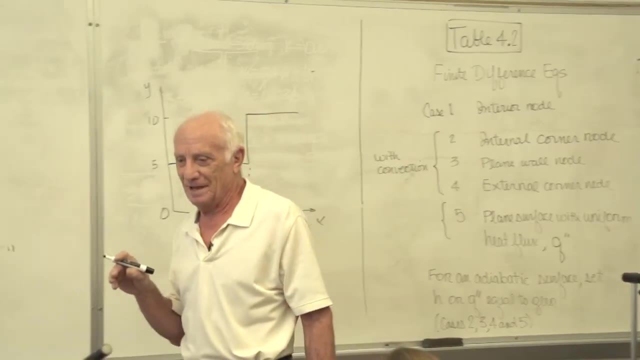 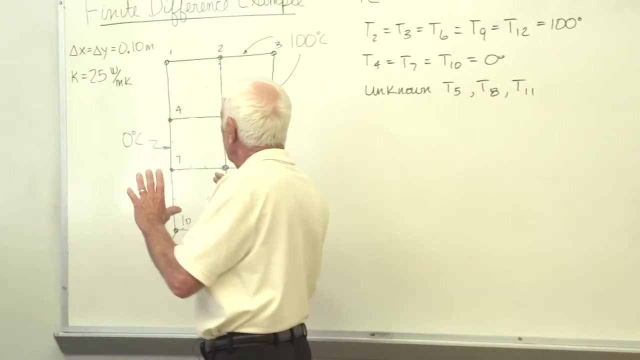 find out What's that called in math: Discontinuity: discontinuous there, infinite jump up there. So anyway, here's what it means in our picture As I approach the upper left-hand corner. on the left-hand wall, the temperature. 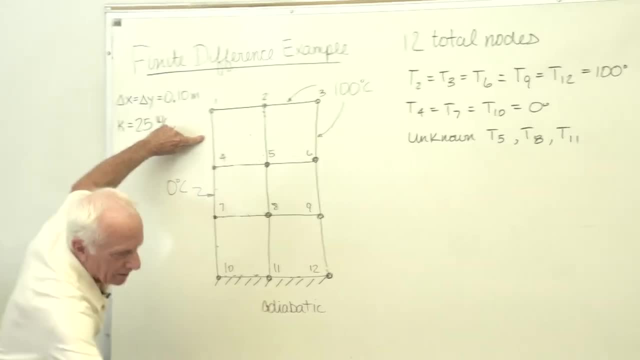 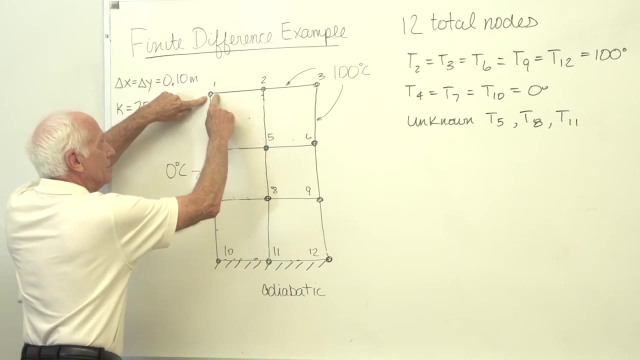 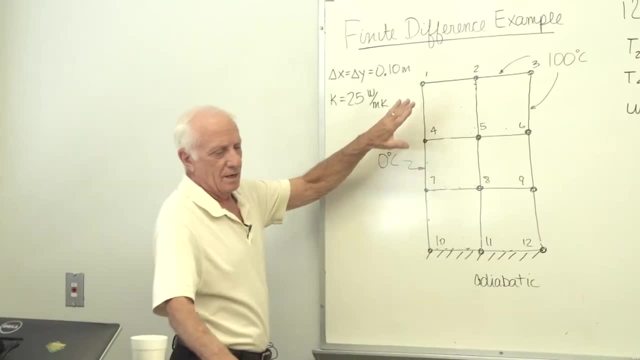 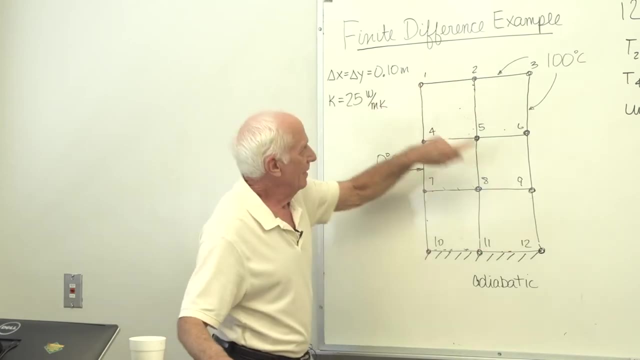 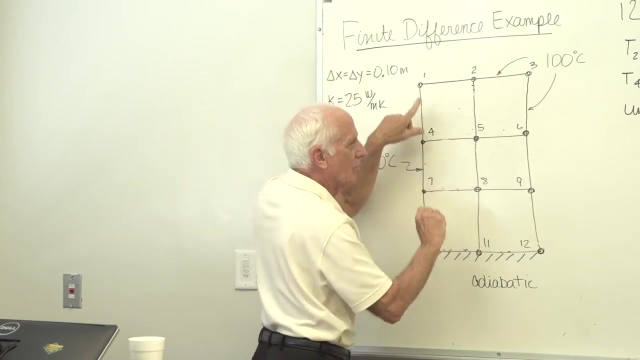 100 and 0.. If this were a copper plate, an electrical problem, where this was zero voltage and this was 100 volts, that will be called a short circuit. All the current would flow bam to there. Nothing would flow inside. 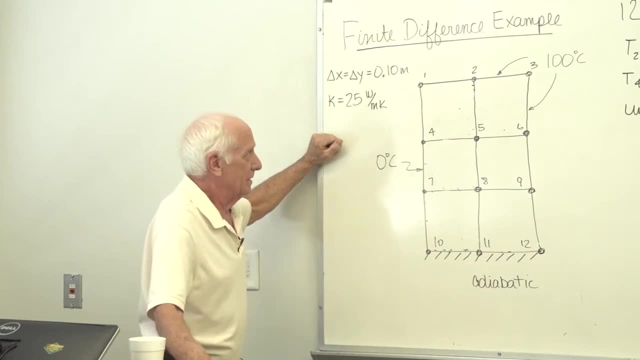 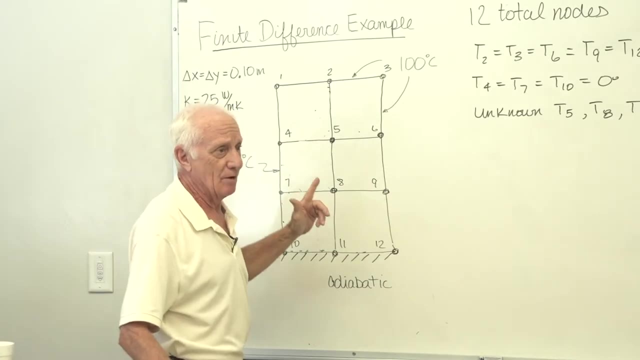 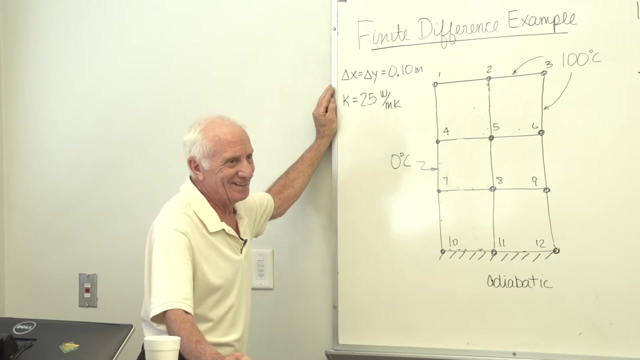 called a short circuit. You can't have that, So it's undetermined. You just say T1 is undetermined. I can't worry about it. Fine, it's out undetermined. Okay, Is that all right? Did you get the idea? 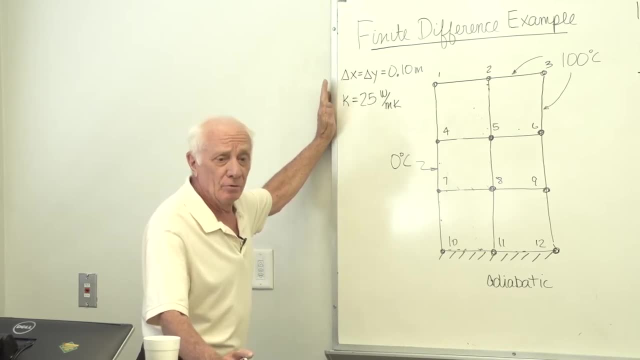 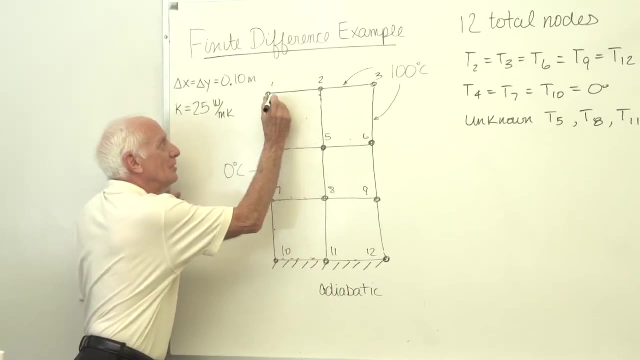 Yeah, I'll say: in the real world, can this happen? No, no, no, you can't do that. You can't do that. What you do is you might put a little thermal insulation right there, a little piece of insulation right there. 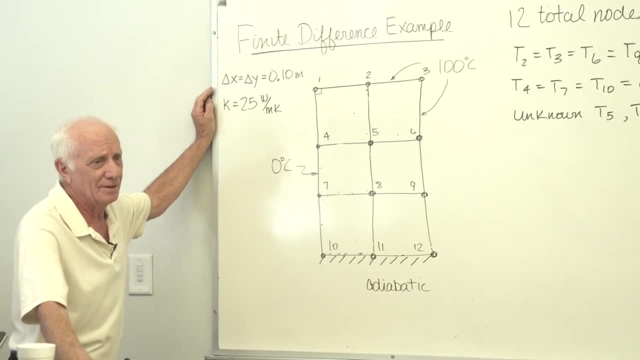 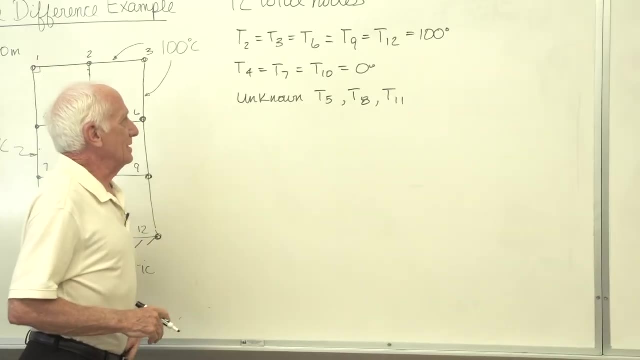 so they don't touch each other. That's the whole point. Don't let them touch each other. That's what you do in the real world, Okay, Okay, back to here. Three unknown temperatures, which means I need three equations for three unknown temperatures. 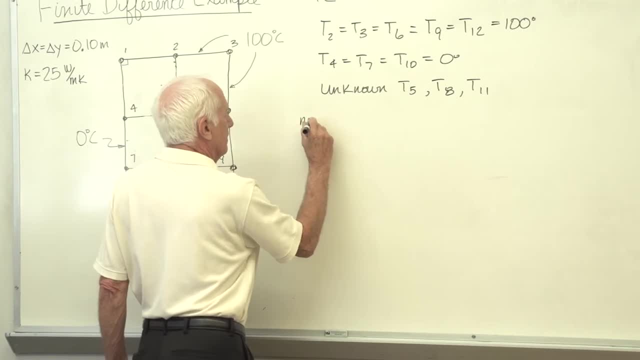 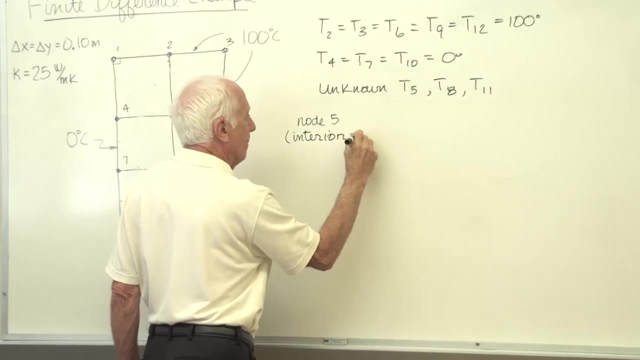 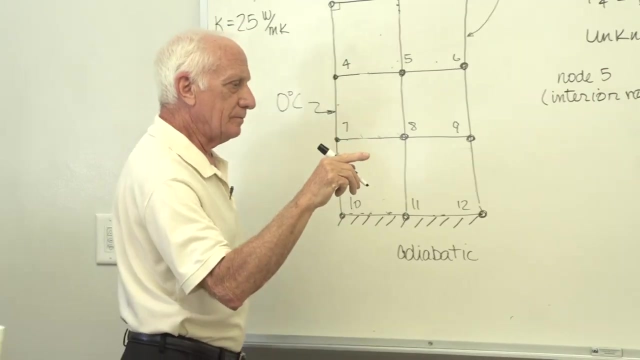 So let's take node 5.. Node 5 is an interior node. So here's what I found out last time For an interior node. here's what you do: You add the temperatures of the four surrounding neighbors and subtract off four times. 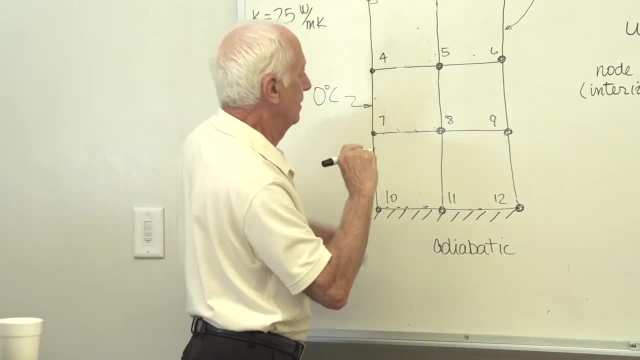 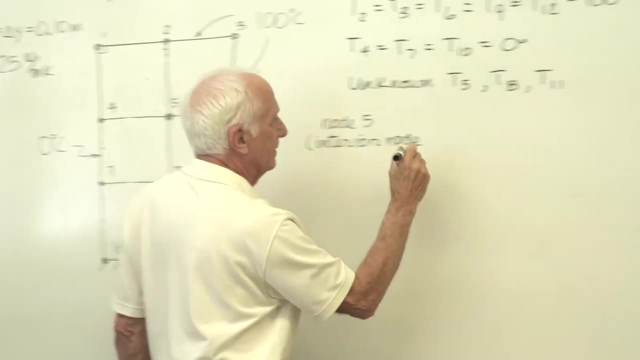 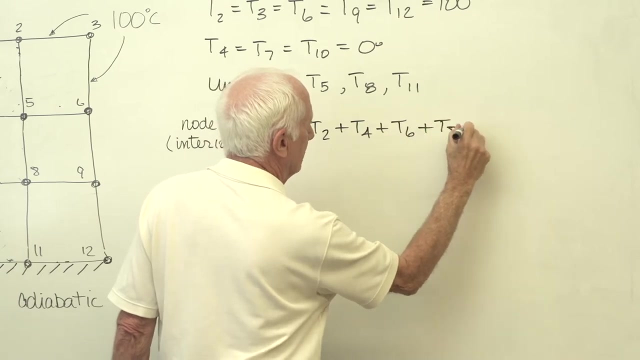 the temperature of the center node and that should be equal to zero. Center node T5. Surrounding nodes 2, 4, 6, 8. Minus four times the temperature of the center node must equal zero. 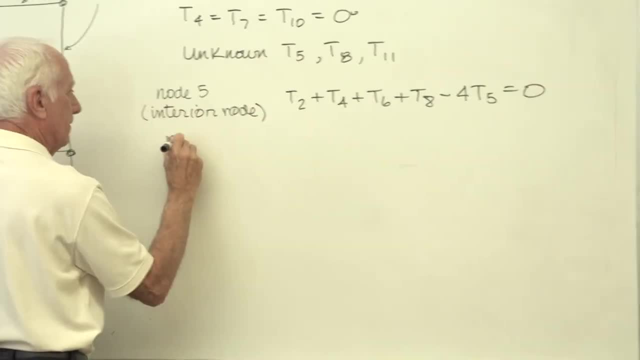 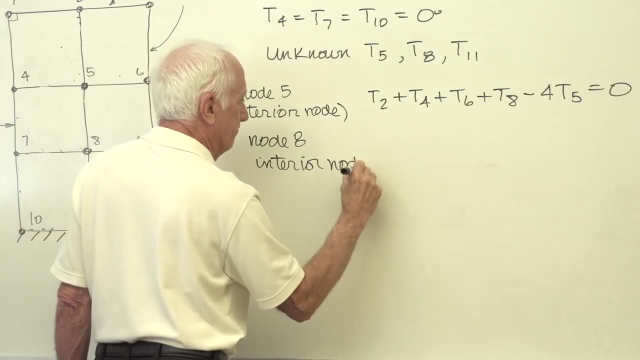 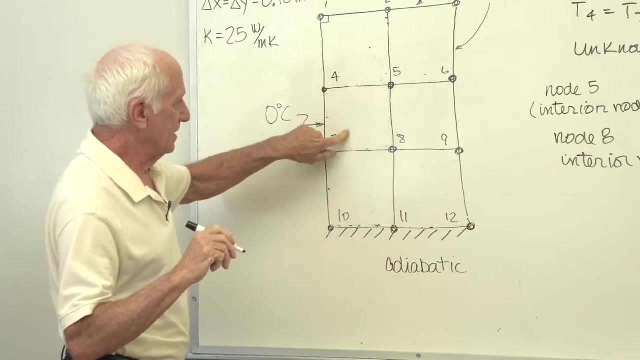 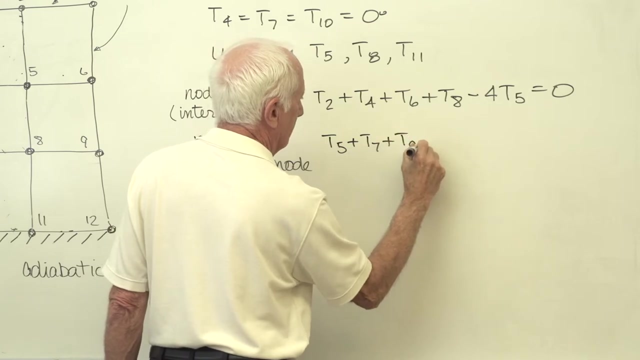 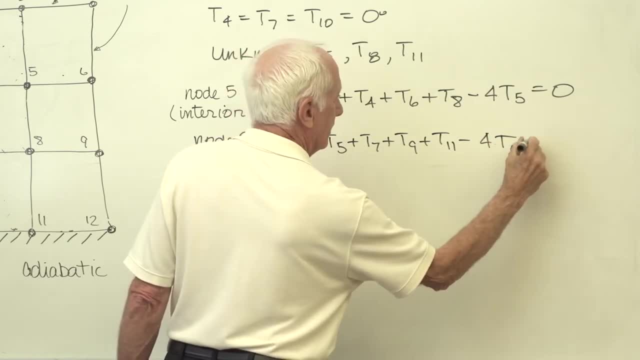 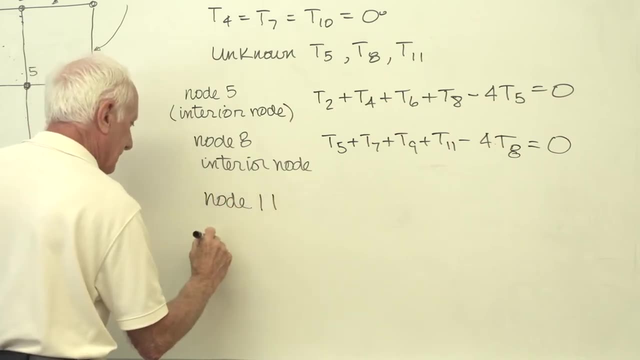 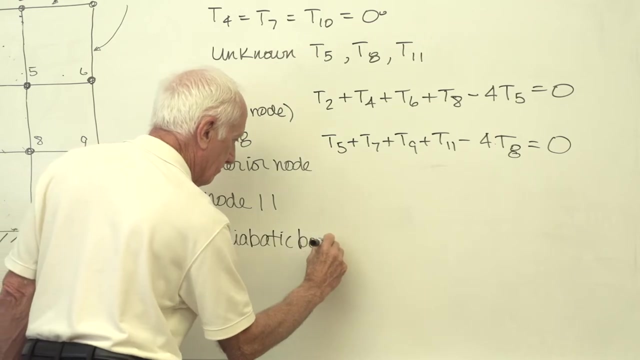 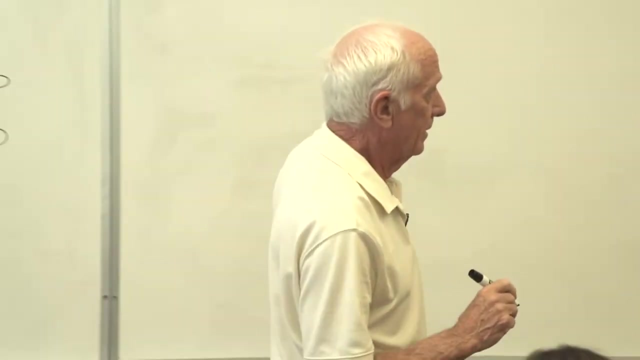 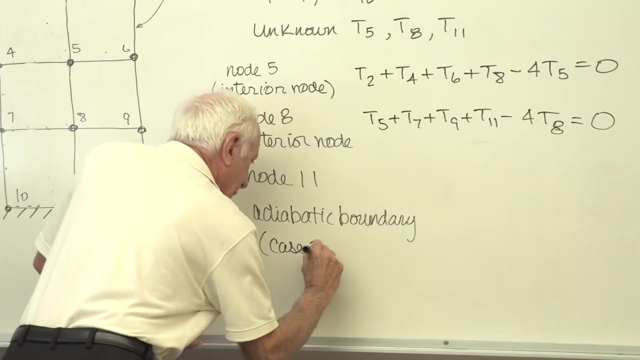 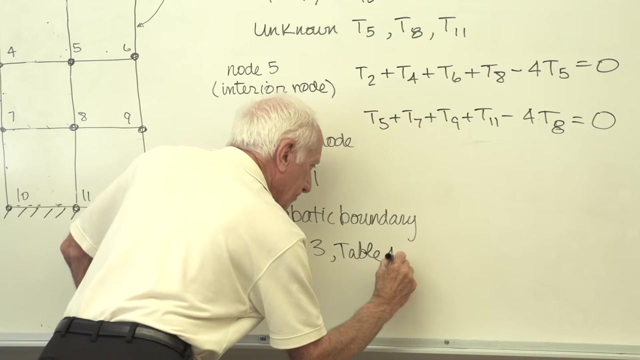 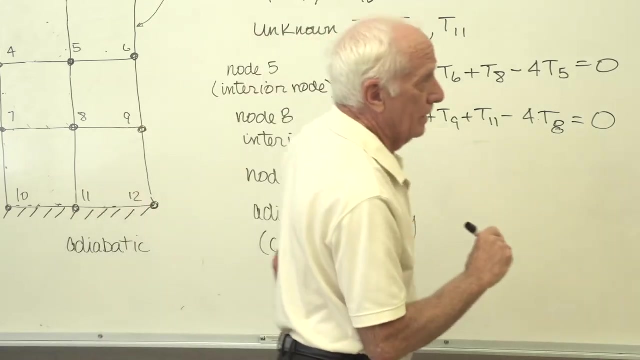 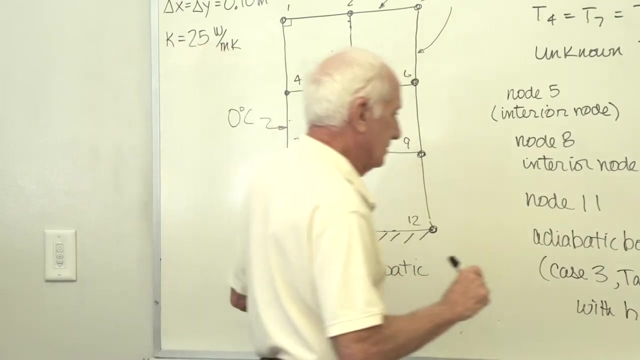 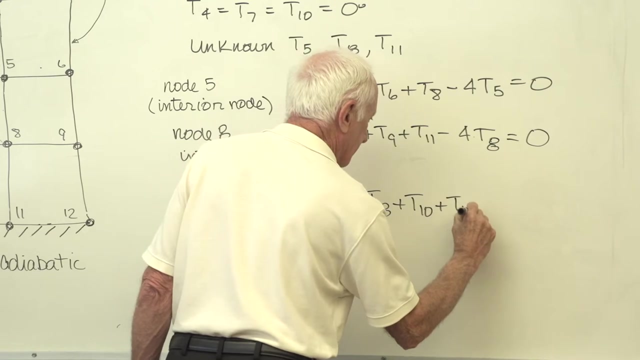 the center node equals zero, Negative, Negative, Negative, Negative, Negative, Negative. Note 11, adiabatic boundary. I'll just say it's case 3 with h equals 0.. Here, 2 times T8 plus T10 plus T12 minus 4 times. 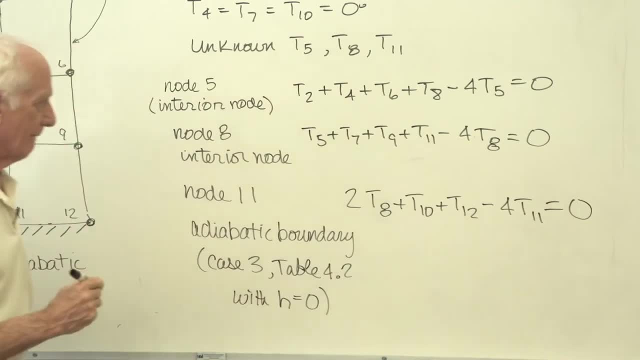 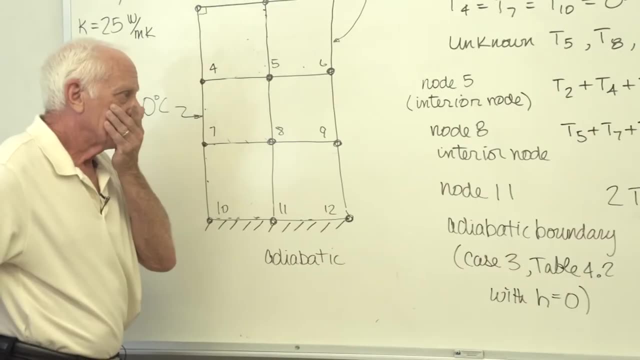 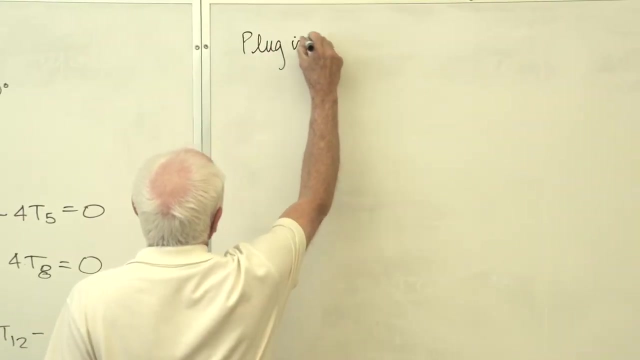 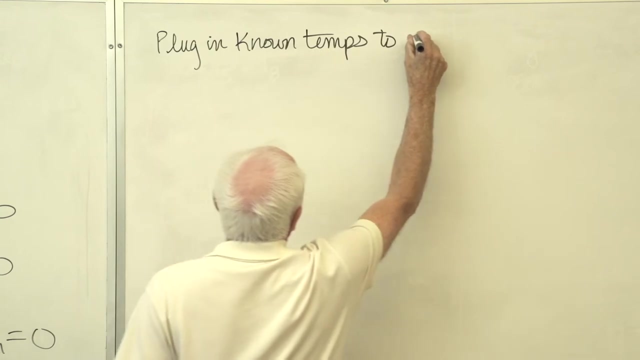 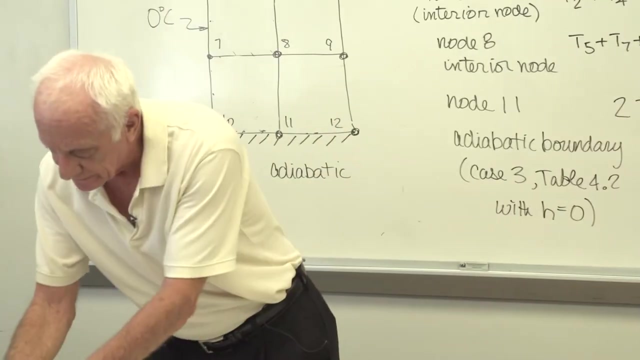 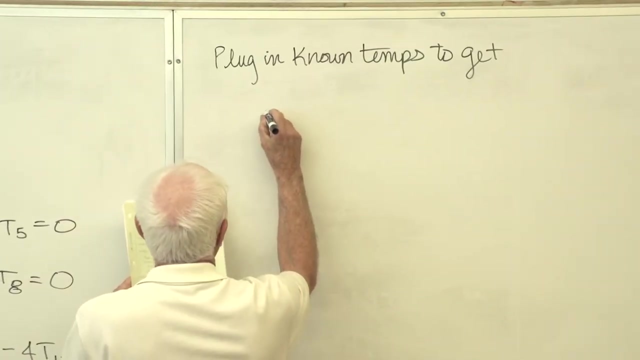 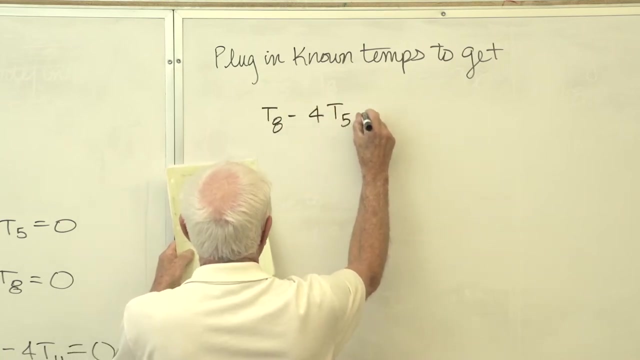 T11 equal 0. You can get that from case 3 by setting h equal to 0. Plug in known temperatures to get. Let's see, Maybe we have some way to use this easy. Let's show you a little bit of our. 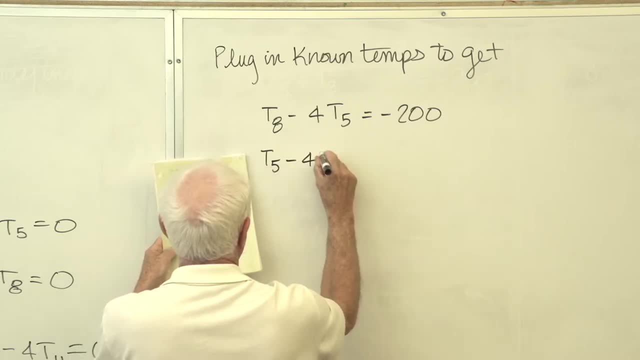 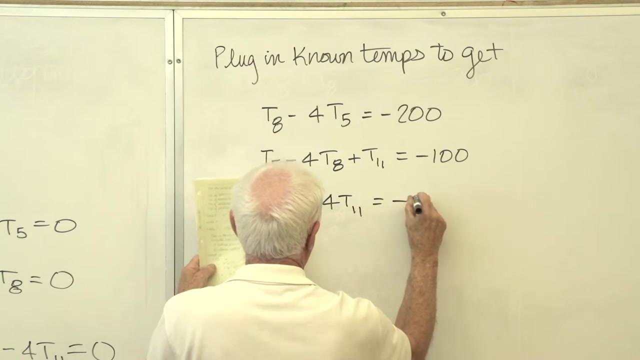 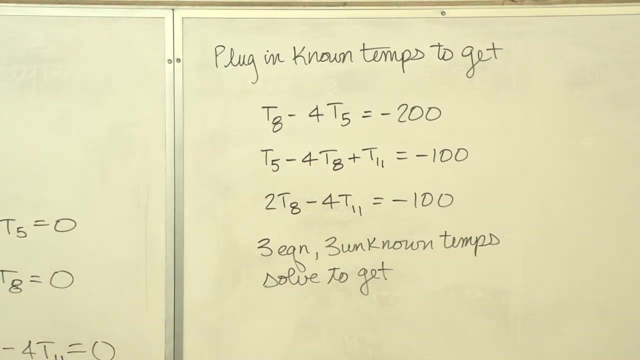 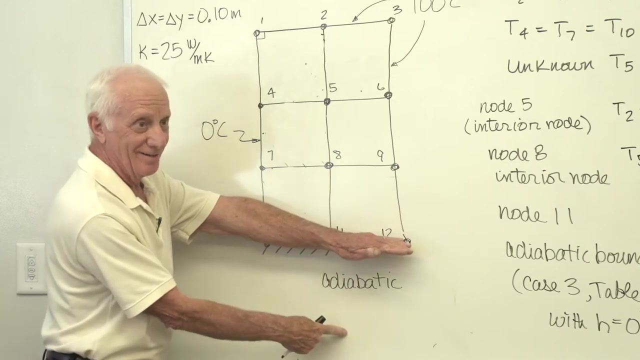 Tambay plan. Let's start with T and then we'll start with the lower axis. Okay, yeah, Adiabatic wall behaves like there was a T8 here and a T8 down here, That's why. So now add: 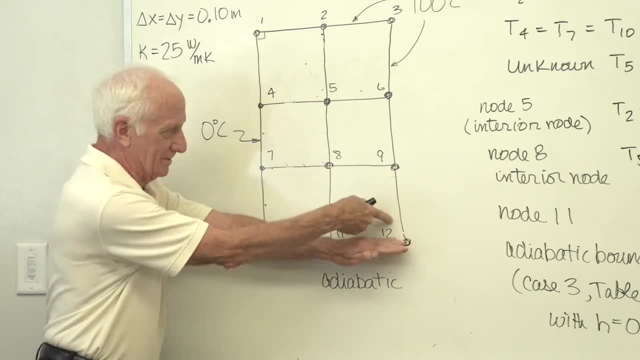 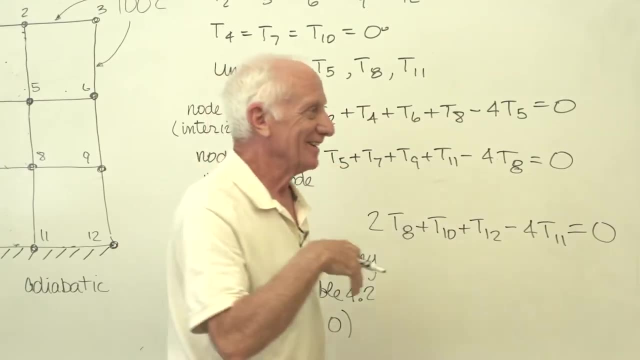 your four neighbors together: T8 plus T10 plus T12 plus T8, two T8s. It's symmetrical about the adiabatic wall. that's why- Okay, Now, I don't need you to solve it. 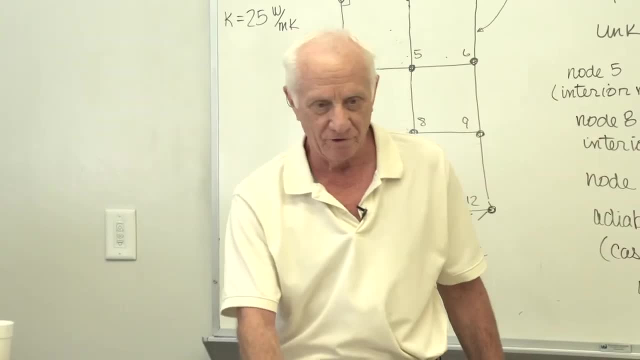 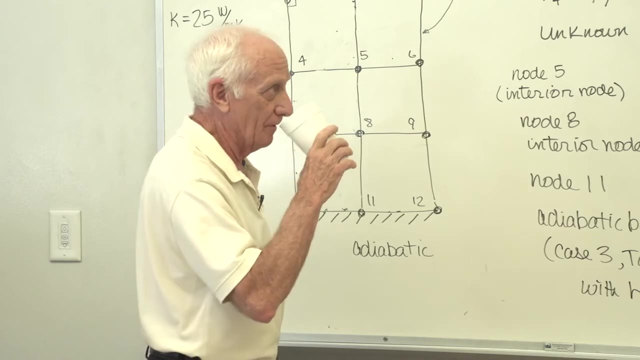 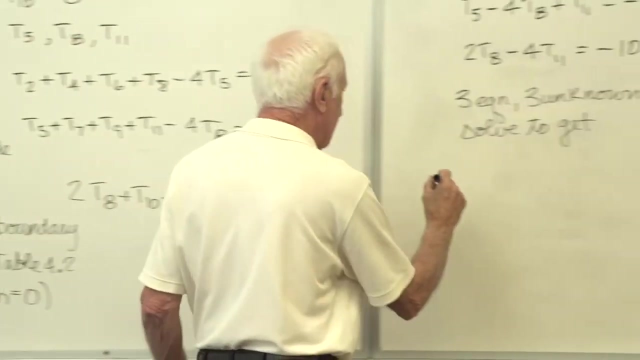 I don't know Excel matrix inversion. you solve it Ti with the solver function or whatever. So it's pretty simplistic. There's three equations algebraic, three unknowns. solve for them. When I do that, I get T1, 63.5 or T5. 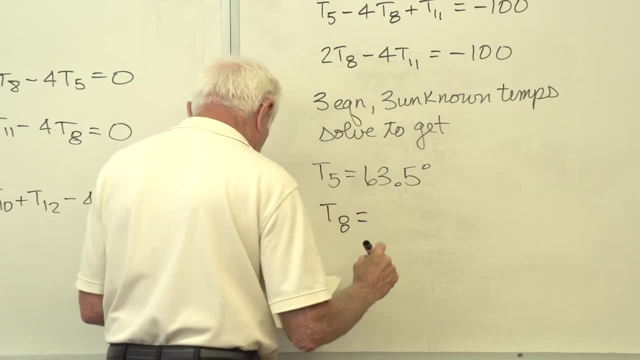 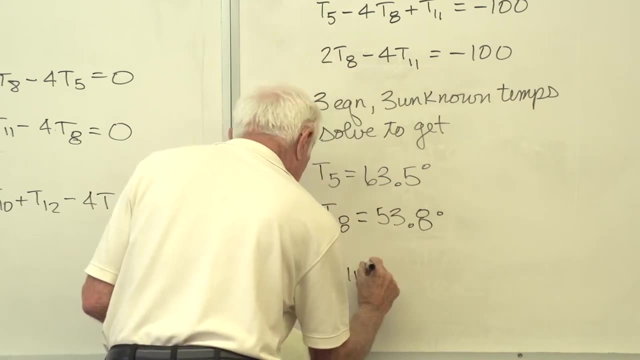 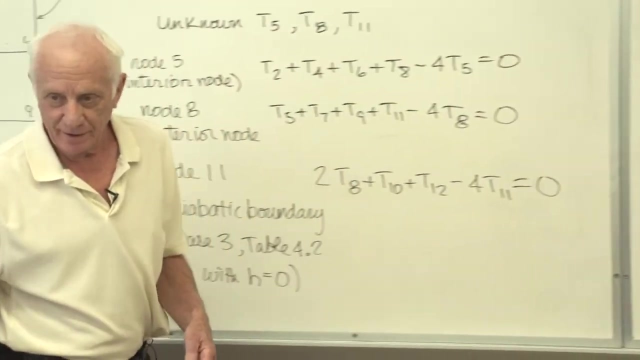 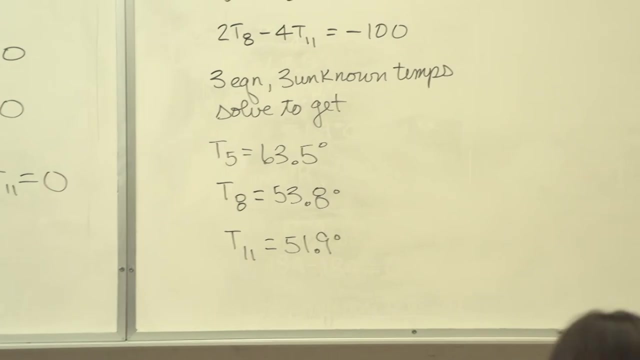 I get T8, 53.8 and I get T11, 51.9.. So that's my first estimate on the interior temperatures and the adiabatic wall temperature at the center. I know those are bad answers. I mean, the grid is way too coarse. 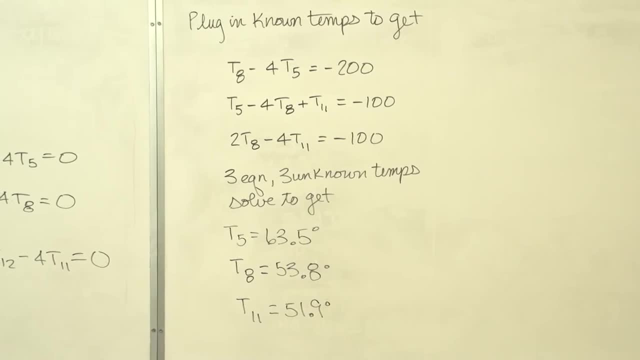 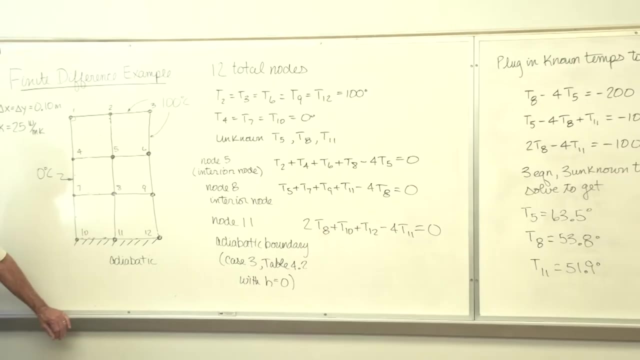 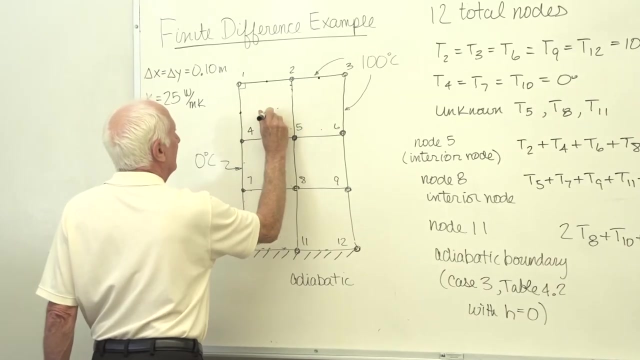 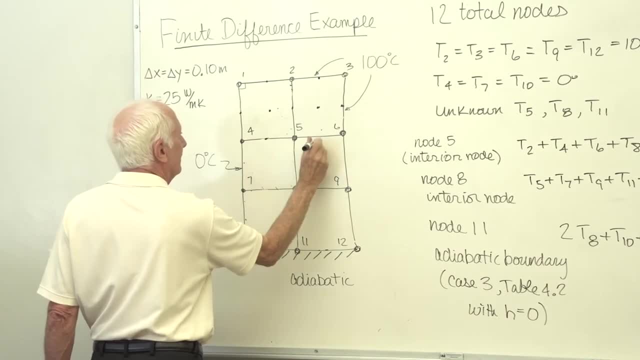 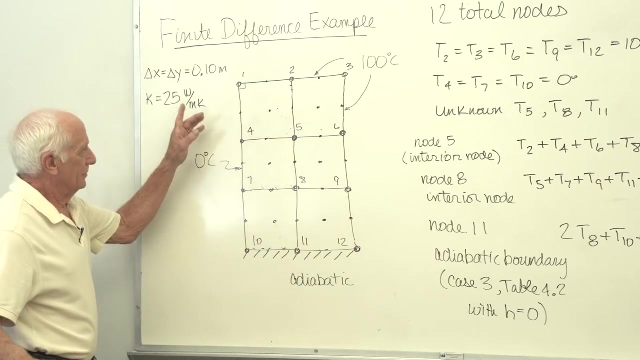 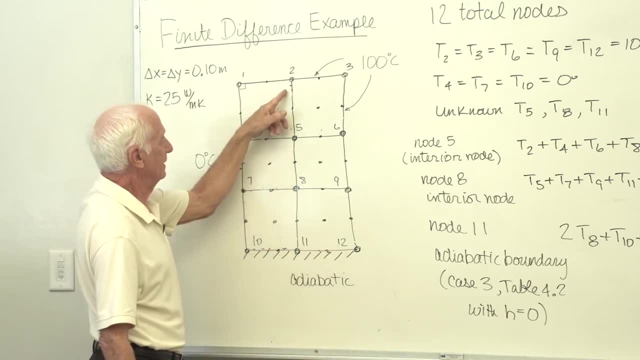 8,, 9,, 10,, 11,, 12,, 13,, 14,, 14.. 5.. One, Two, That's it, Thank you now. I'm going to fill this box now: 14,, 15,, 16,, 17,, 18,, 19,. is that right? 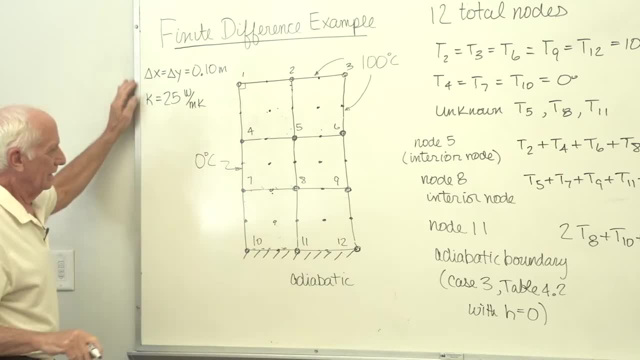 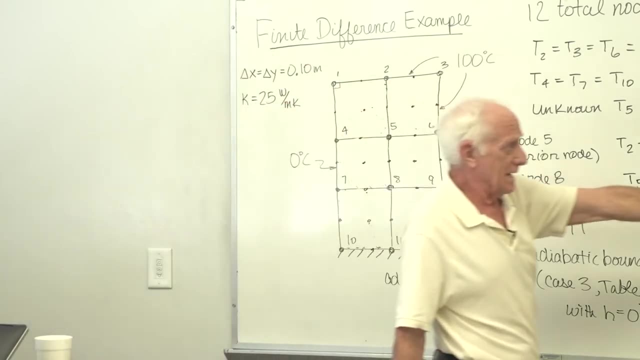 1, 2, 3, 4, 5, 6,, 12, 18.. Now you've got 18 equations, 18 unknowns. Those answers now will be a lot closer to the real answers You say yeah. 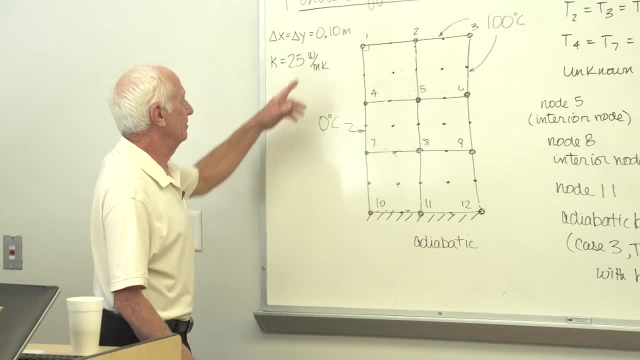 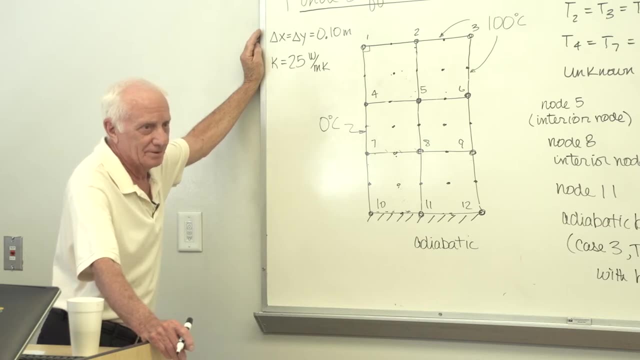 but I really want accurate answers. Make the grid size one centimeter. Oh my gosh, hundreds of nodes. now You're solving 150 by 150 matrix On your TI. you wait overnight for 12 hours until it spits the answers out. 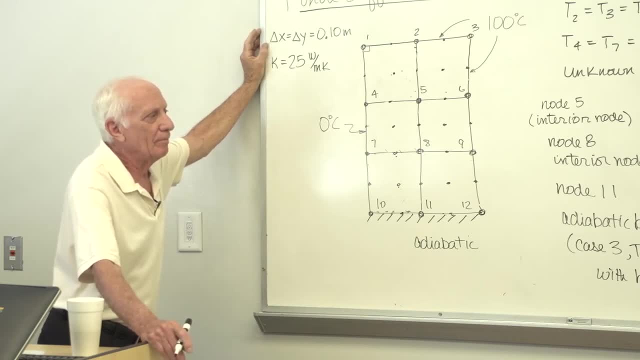 Yeah. so what's the penalty? you pay More computing time. What's the good news? Better accuracy. Is it worth it? That's your call. You're the engineer. You figured out. What do you want? Where, if I have the grid size? 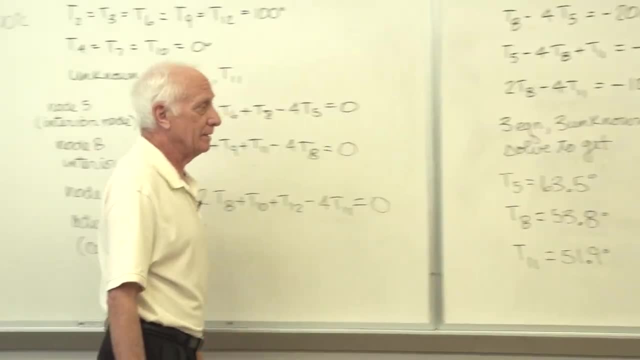 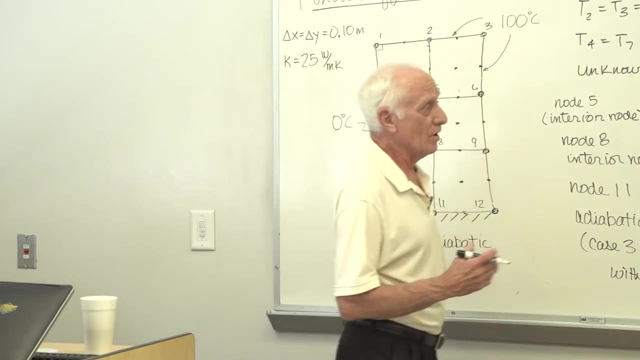 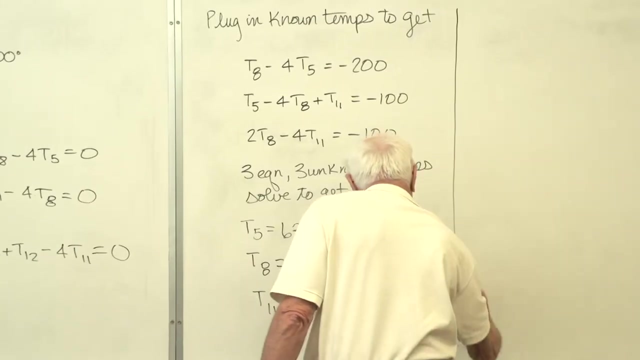 the temperatures don't change by more than one-tenth degrees C. Okay, fine, That's your criteria. Keep going till you get there. So that's the game you play. as far as what accuracy do you want? Okay, Now, this is ME4150. 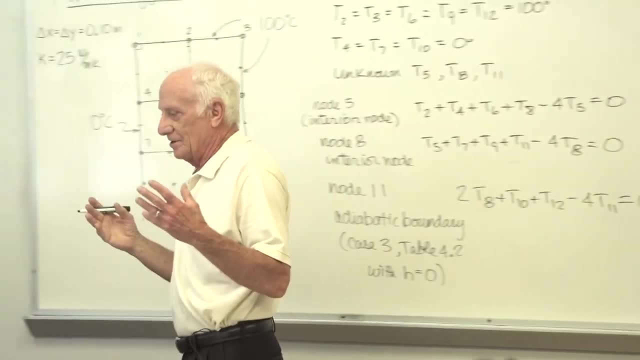 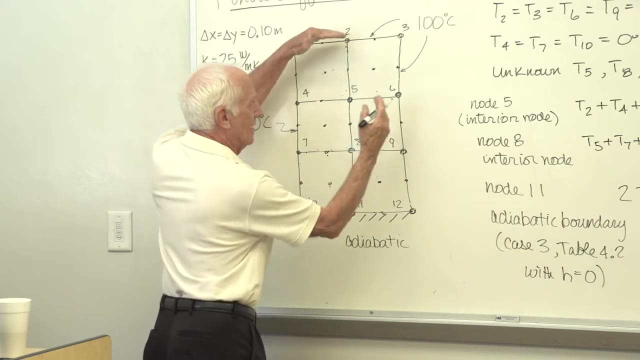 The title is heat transfer. So same old game With conduction. once we get the temperatures, the next thing to do is to find out how much heat's transferred from where to where- From the top and the right-hand side, out the left-hand side. 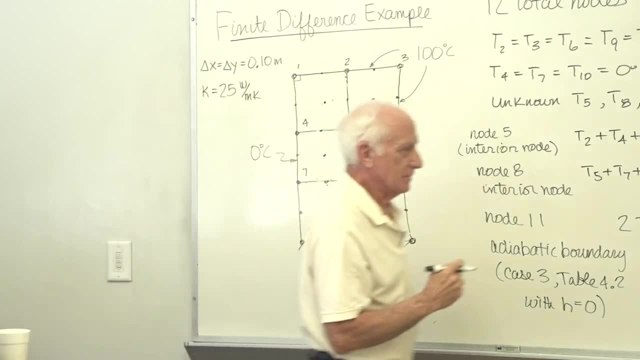 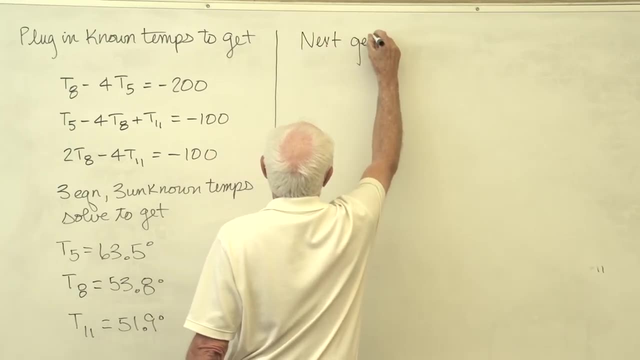 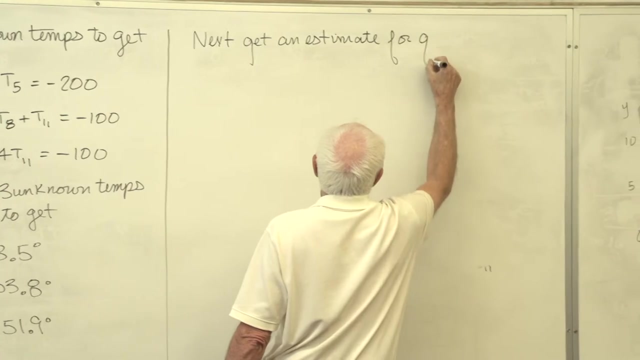 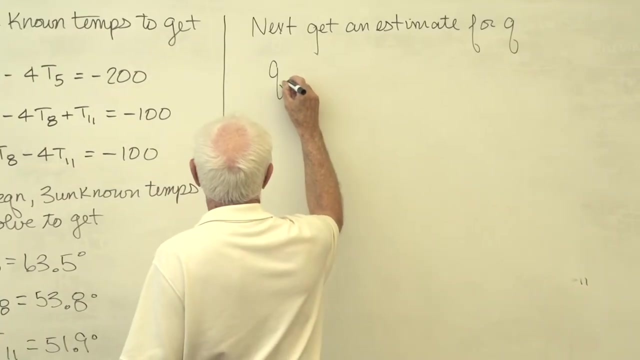 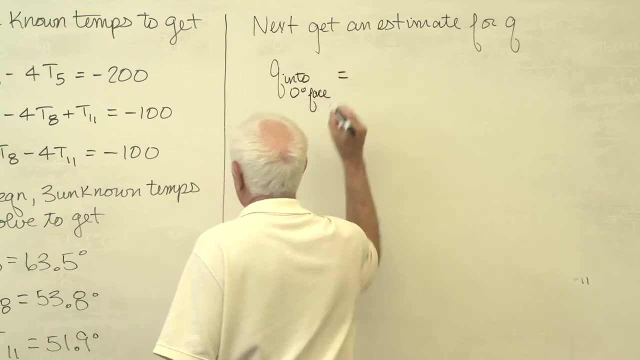 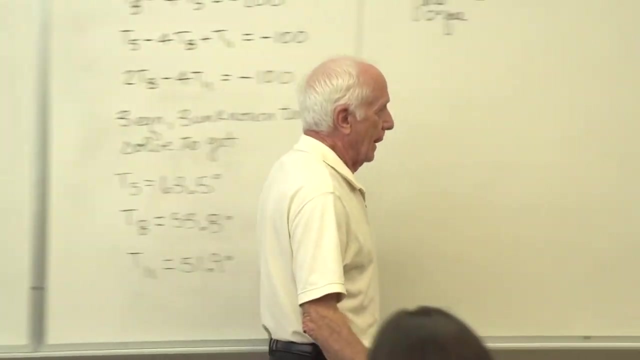 100 degrees goes out the zero-degree face. So I'm going to find out how much heat we have. First we'll look at Q. that comes into the zero-degree face. All right, Here's how we do it. Remember we first talked. 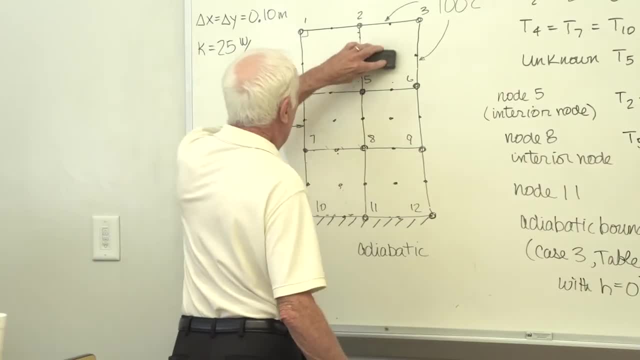 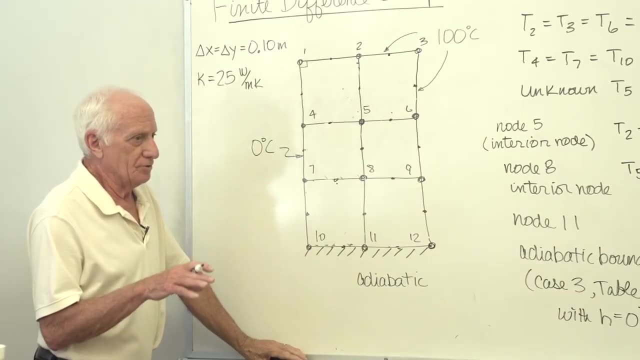 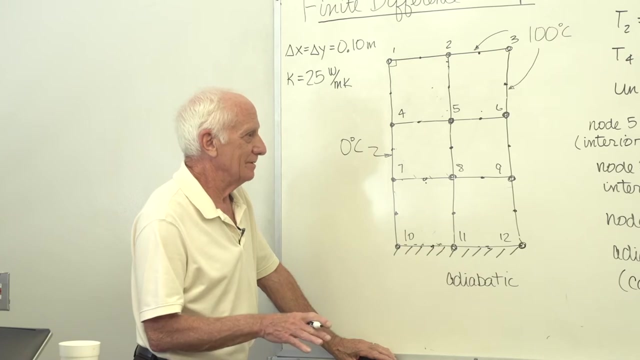 about numerical methods in the grid and we said you lump the mass at the nodes and the nodes are connected by heat conducting rods. The only way for heat to be conducted is through the heat conducting rods. Here's a node on the zero-degree face. 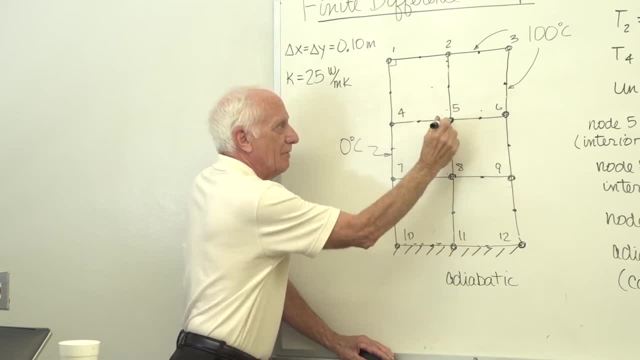 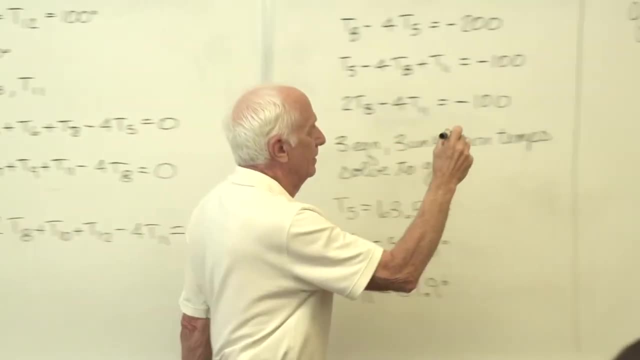 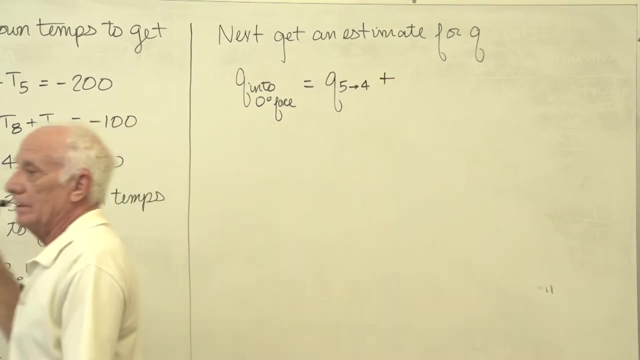 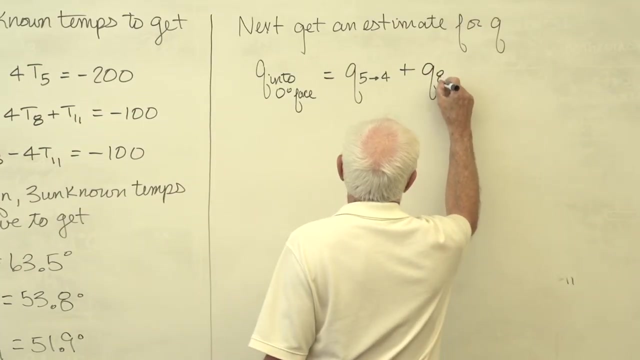 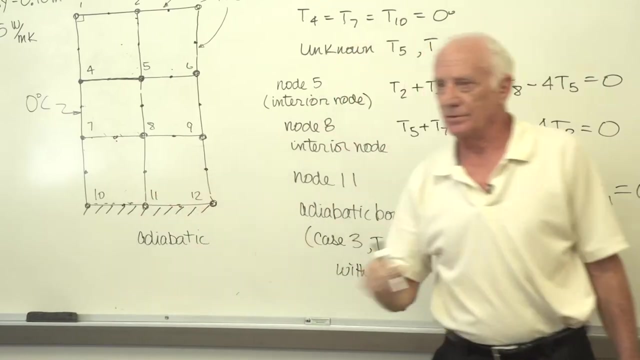 Heat comes in from the right-hand side. heat goes from 5-4 through this heat conducting rod right there, Q5-4.. Heat goes from node 8 to node 7 through the heat conducting rod. Heat goes from 11-10 through. 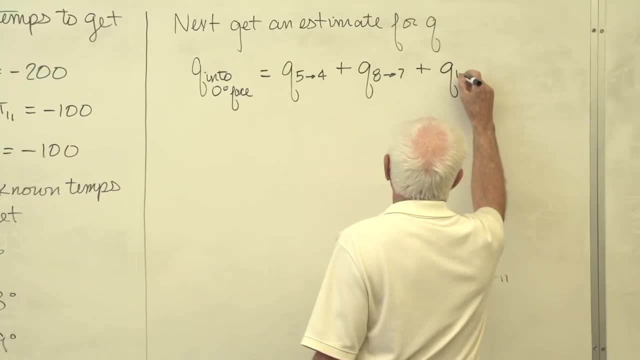 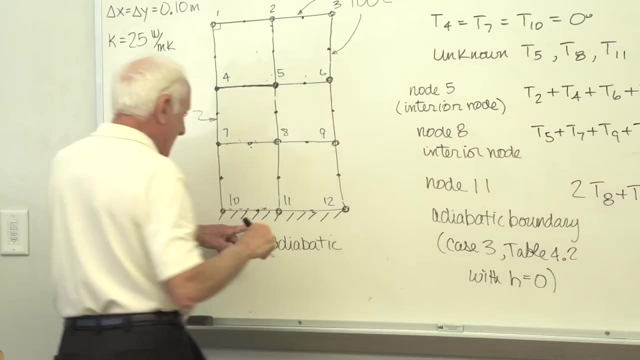 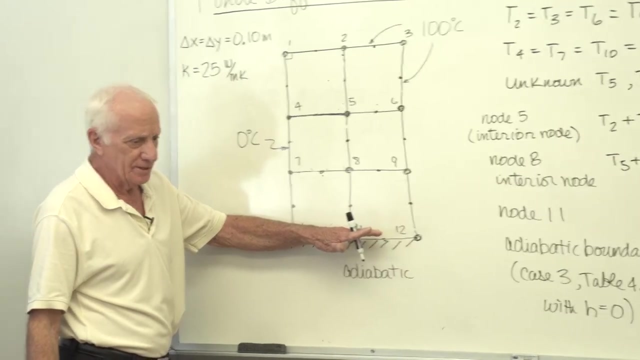 the heat conducting rod. Now don't get confused. You say, yeah, but that's an adiabatic wall. I know, but remember what adiabatic wall means: Heat will not be transferred normal to the wall. I understand that. 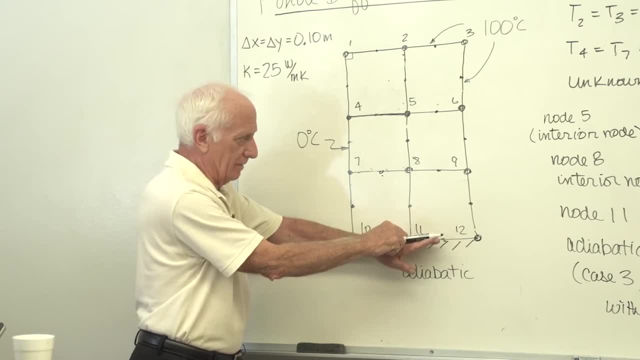 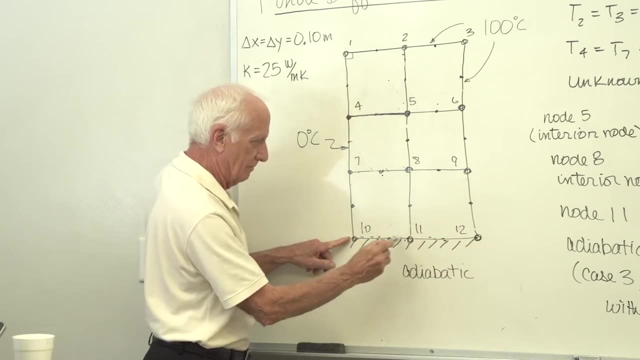 Can heat be transferred parallel to the wall? Sure it can. What's this temperature 100. What's that temperature Zero? Of course there's going to be heat transfer along that. This is a heat conducting rod. Heat can't go this way. 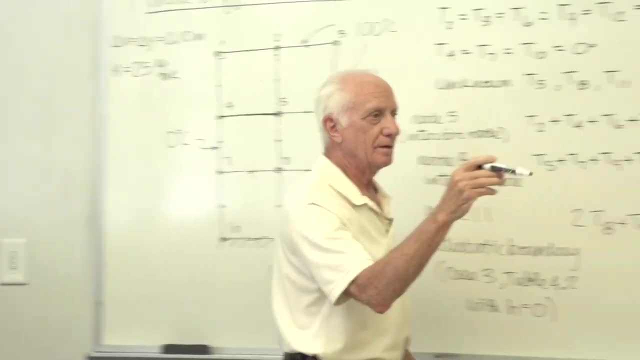 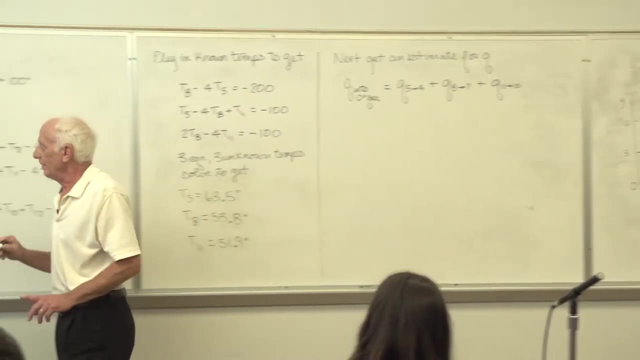 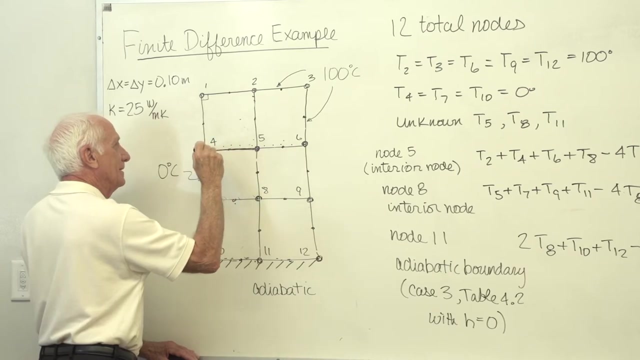 But it can go this way. Question over there. Yeah, Wait, what The heat conducting rod? No, I'll give you an example At temperatures 100, 90, 80, 70,, 60,, 50,, 40,, 30,, 20,, 10, 0. 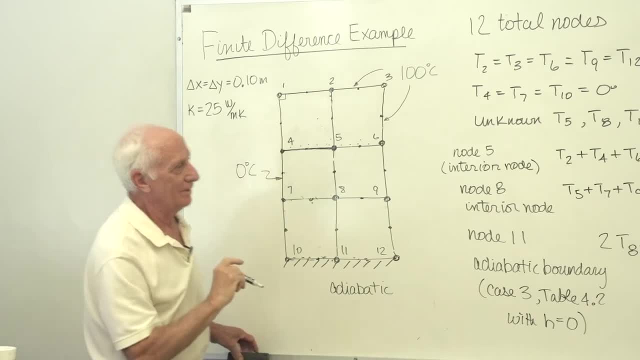 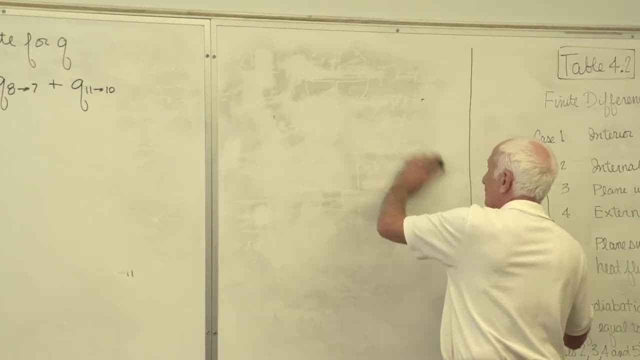 It's not the same temperature. Oh, I'm glad you mentioned that. Thank you, I'm so glad you mentioned that Because what I meant to do first was to draw the heat flux plot, just to give you an engineering interpretation of this. 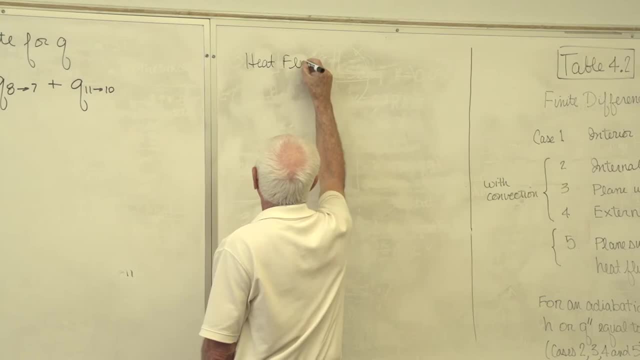 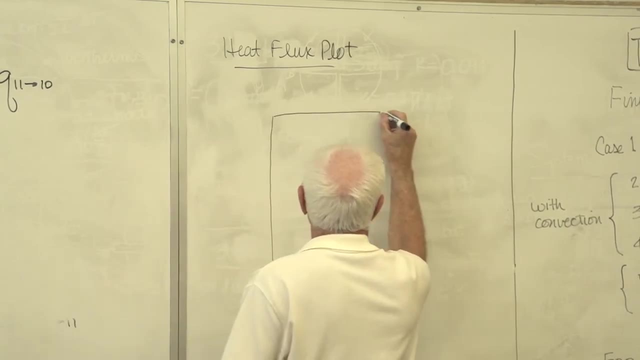 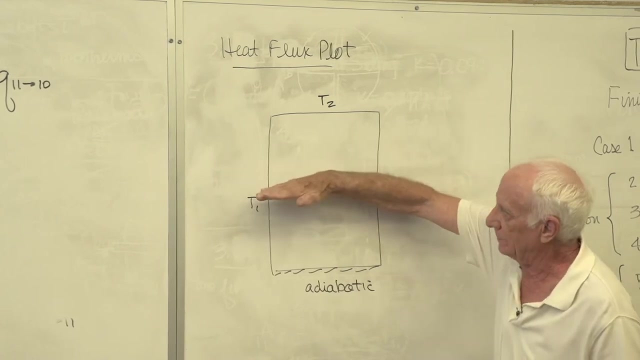 Heat flux plot. So here is our adiabatic surface. at the bottom I'll say: T1 is here, T2 is here, T2 is here, Okay. Geometric symmetry: yeah, right through the middle. Geometric symmetry, yeah. 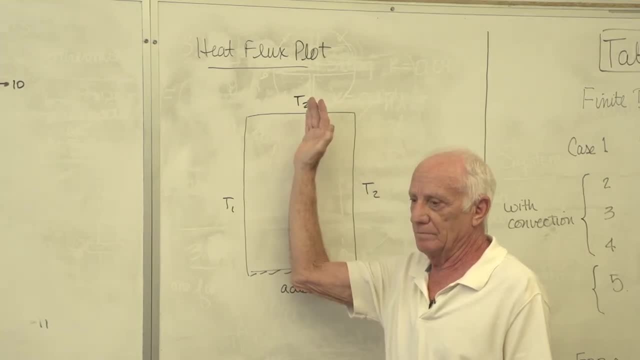 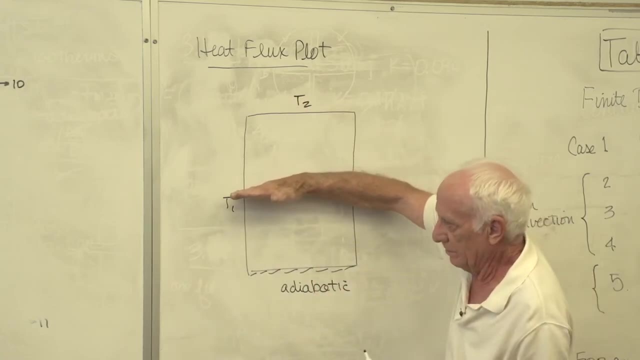 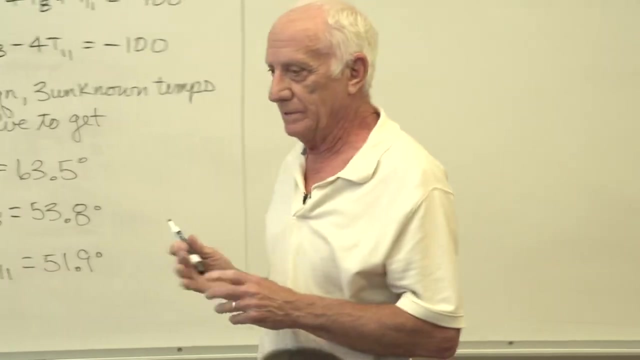 right through the middle vertical and horizontal lines, Thermal symmetry: vertical line T1, T2, no. Horizontal line through the middle: adiabatic T2, no, There's no lines of thermal symmetry. Conclusion: okay, I can't use that. 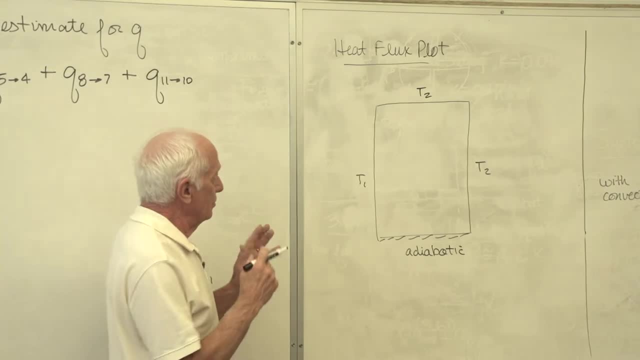 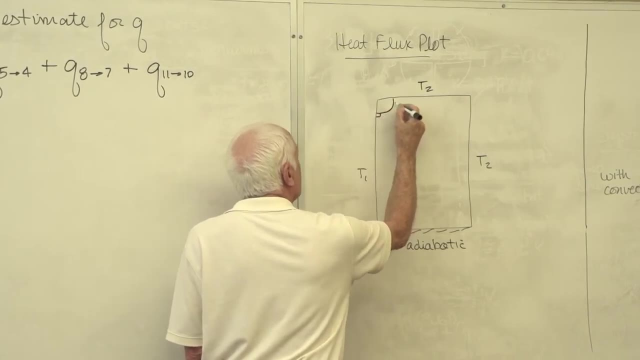 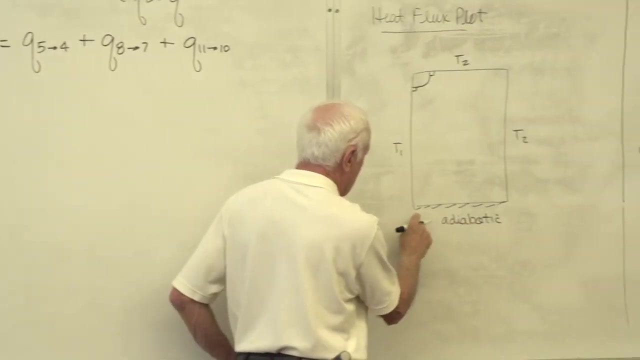 But here's something we did twice already. We said you know where two corners come together of different temperatures. The heat pretty much flows around the closer you get, almost like a quarter circle almost. So I know that one At the bottom this is adiabatic. 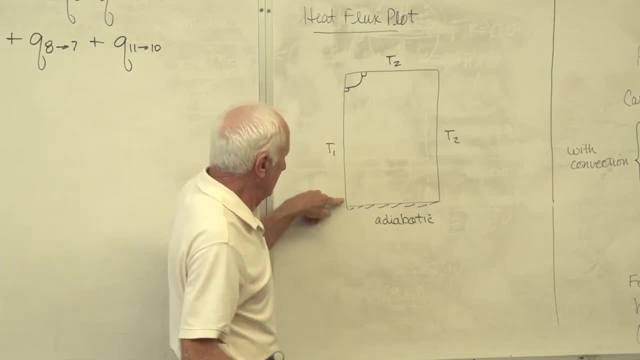 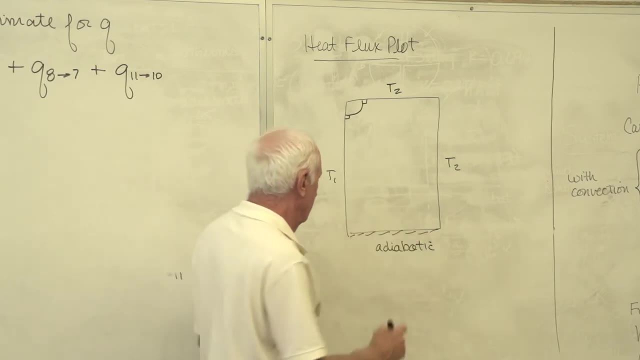 Let's assume T1 is hot, T2 is cold. Heat comes in near the bottom of the hot surface, T1. It can't get out the bottom, So it pretty much travels along here somewhat horizontal like that. Okay, there's an adiabat. 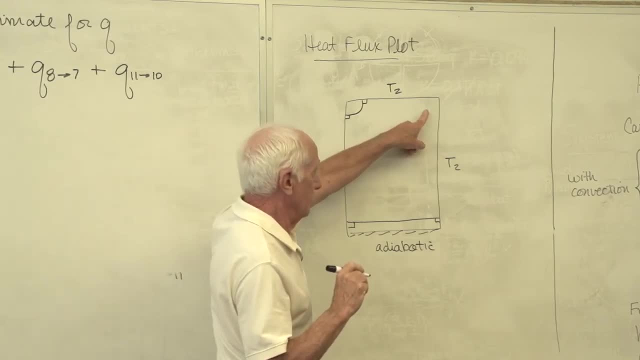 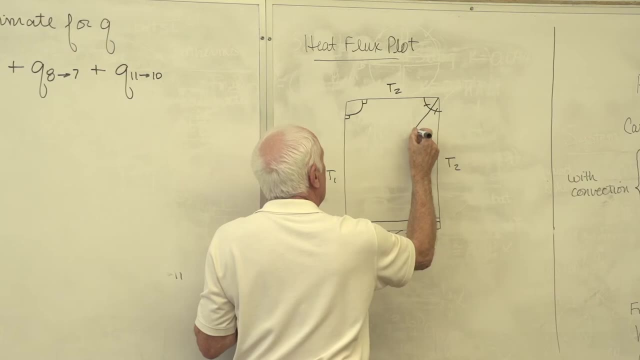 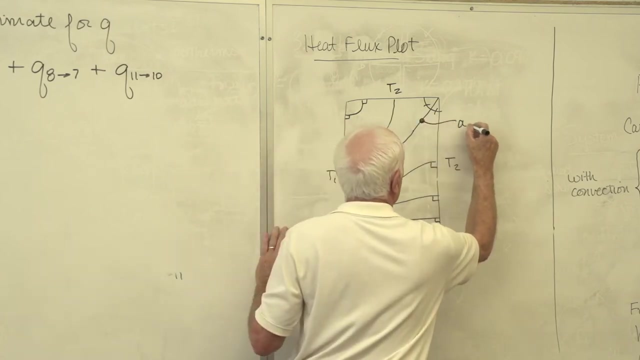 Oh, that's an isothermal corner. I know an adiabat comes out of that corner and it bisects that corner and then it has to go out down here or vice versa. Fill in the rest. There they are. These are the adiabats. 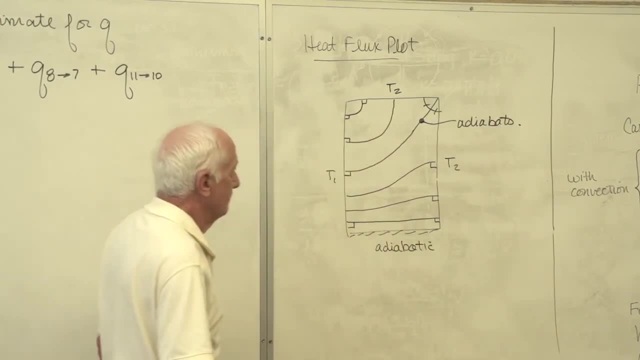 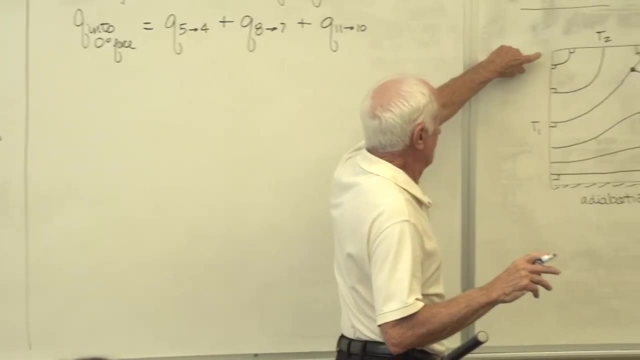 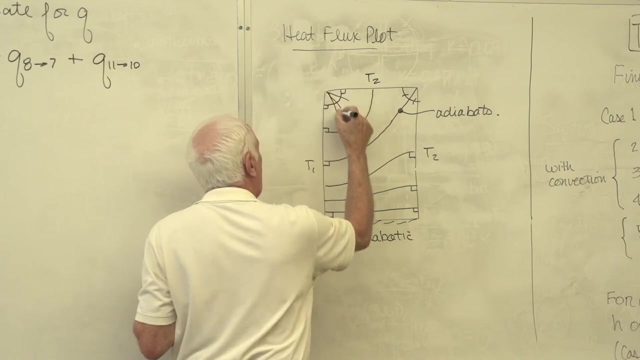 Now we'll draw the isotherms. We did it twice before. The isotherms that come out of a corner where two different temperatures are there, at the corner: T1, T2, they come out in a fan pattern like that: 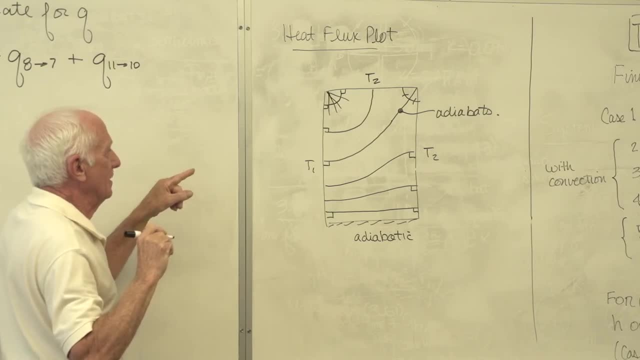 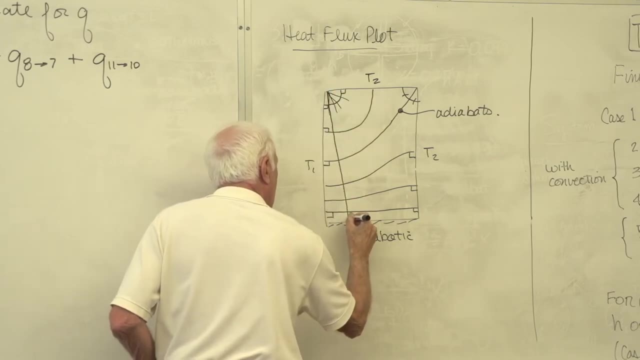 Okay, good, When the isotherms get to an adiabatic boundary, it says they come in at right angles. Okay, Everywhere, everywhere, inside the boundaries, it says they must cross at right angles. Okay, draw a few of these in. 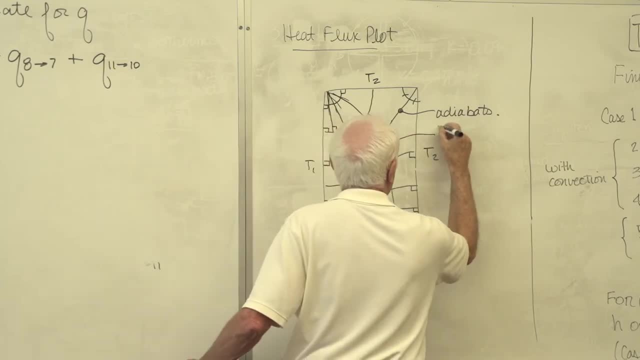 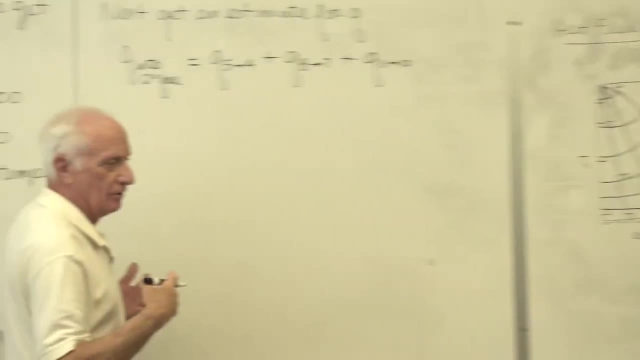 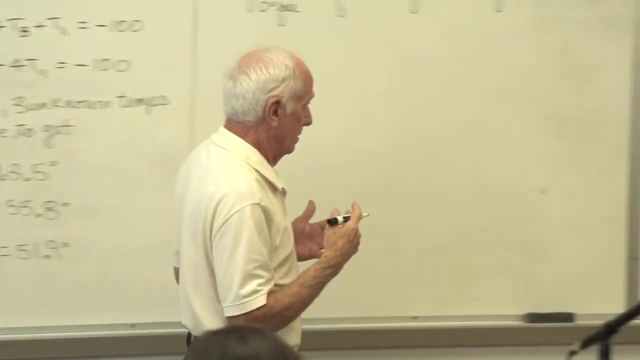 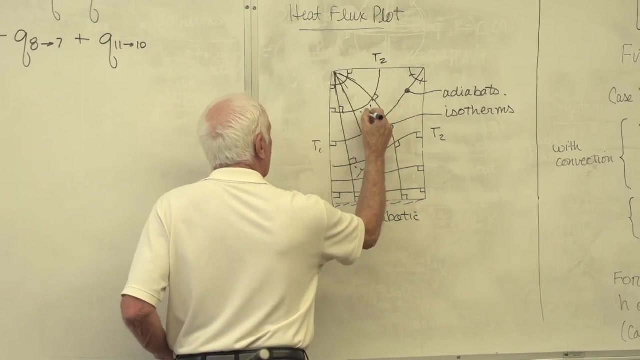 These guys are the isotherms, So that gives you a little bit of engineering intuitive feel for what's going on. If you want to get more accurate, you can construct curvilinear squares. He's real good. He's not bad at all. 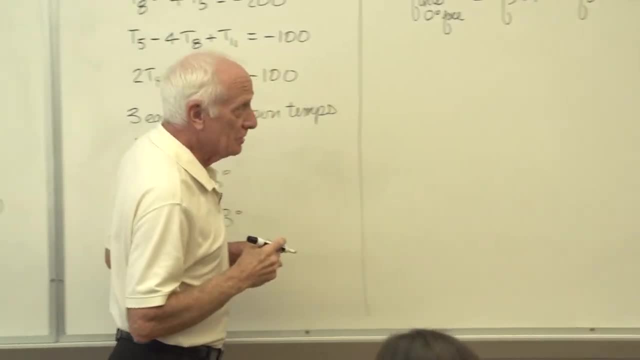 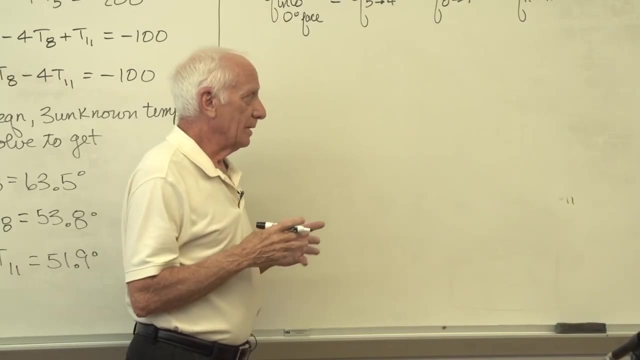 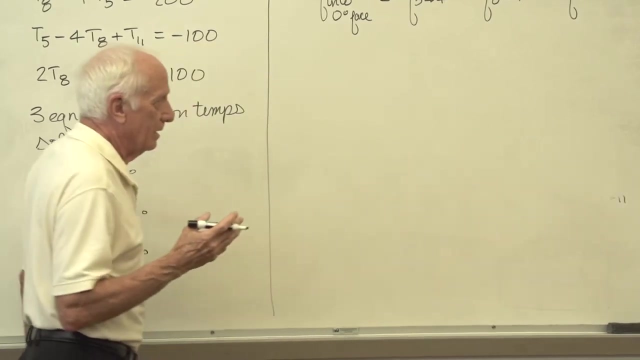 You can do that and that'll give you an estimate of the heat flow, mk, delta T over n. It'll give you an estimate of temperatures in there if you construct reasonably curvilinear squares. So yeah, but we're doing it now by numerical methods. 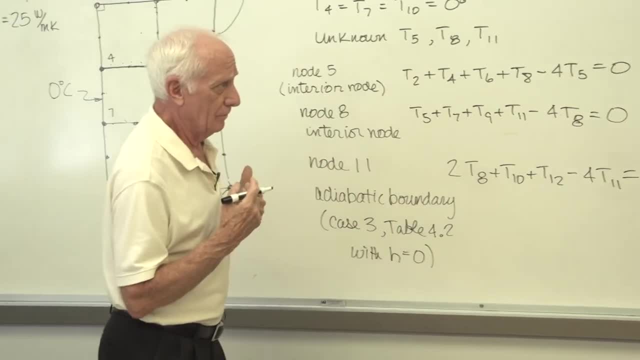 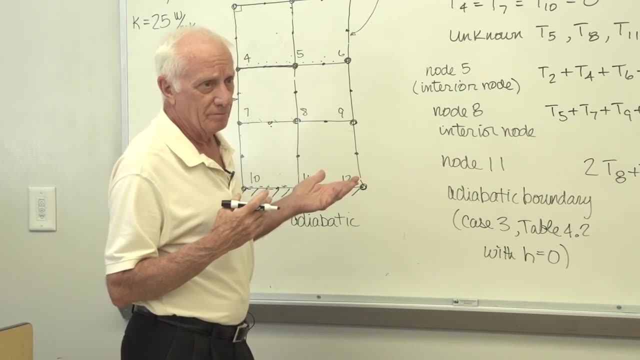 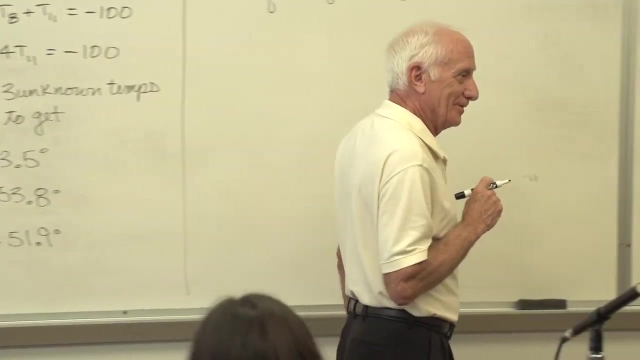 But that. that's the physical picture of what's going on, which gives you some feel for the problem. Numbers on a spreadsheet do not give you a feel for a problem. Graphical things like that give you a feel for a problem. Why do you think Moore's circle is so important? 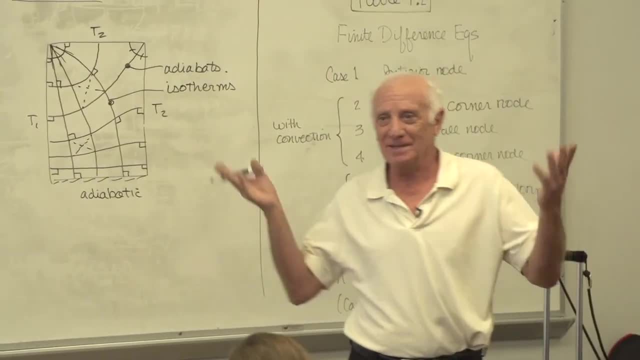 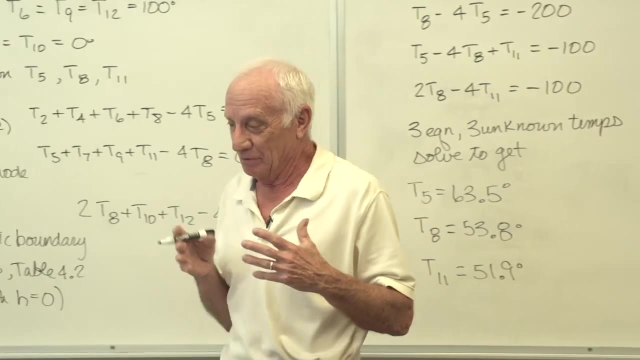 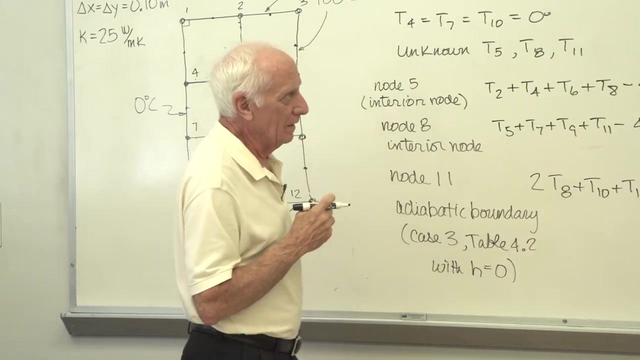 You can do it by equations and they're accurate to 15 places accuracy. Oh no, Moore's circle tells a great story, a phenomenal story, but you see it visually. It gives you that engineering, intuitive feel for a problem. Same thing here. Let's do it. 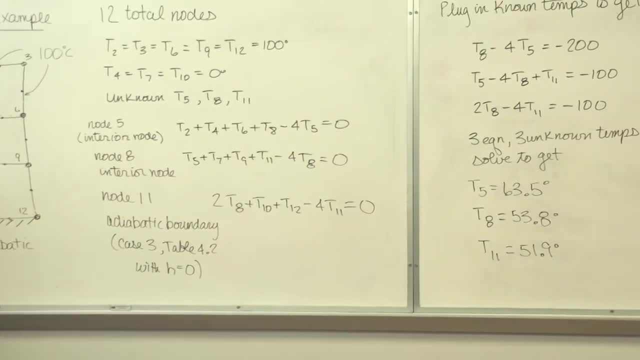 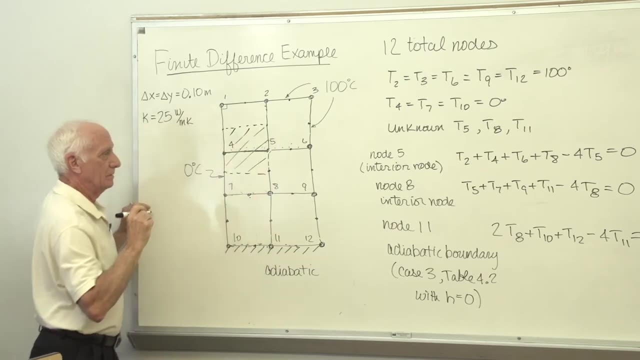 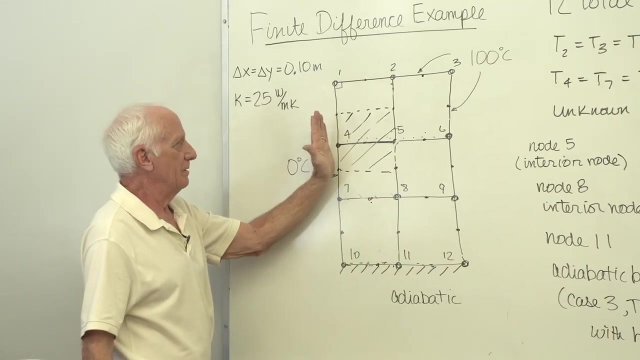 Q5 to 4.. Now this heat conducting rod replaces that much material. 5 to 4.. Here's the heat flow. What's the area? My hand, what's that? Delta y times 1, the area is delta y times 1.. 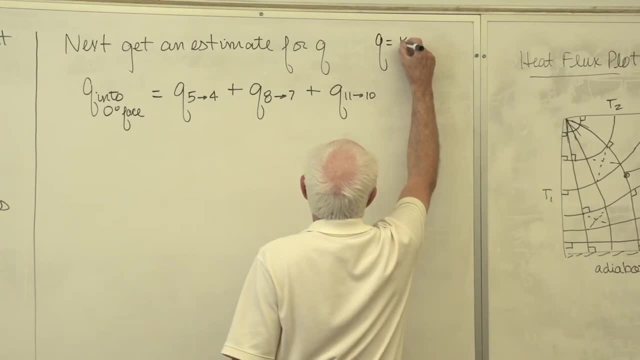 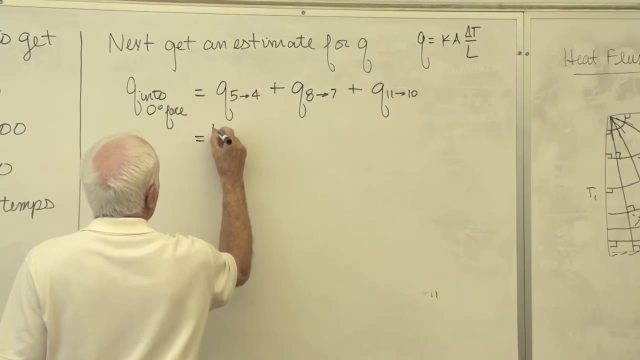 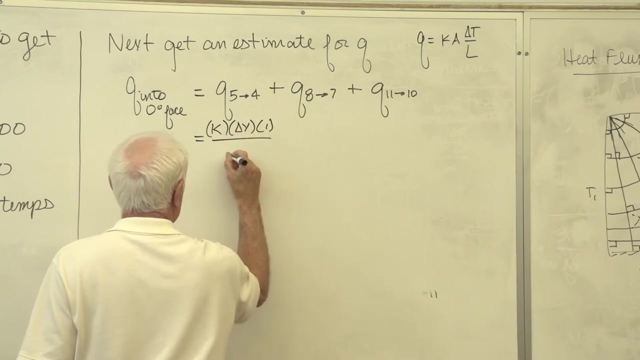 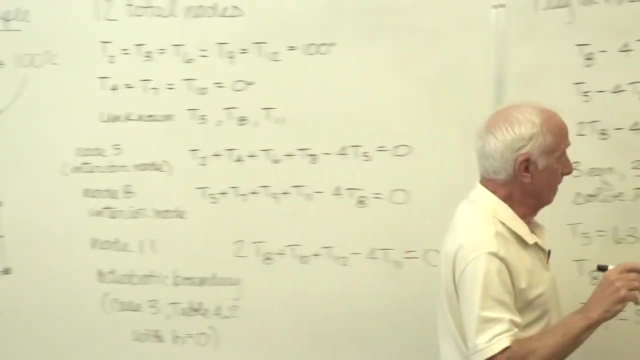 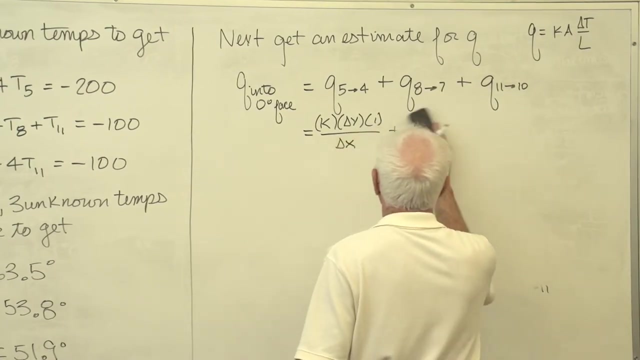 We're using Chapter 1.. Okay, K, the area. delta y times 1, divided by the distance, the heat traveled, delta x. Okay, Eight to seven, same thing k. Oh, put the temperatures in there: T5 minus, T4 plus k area. 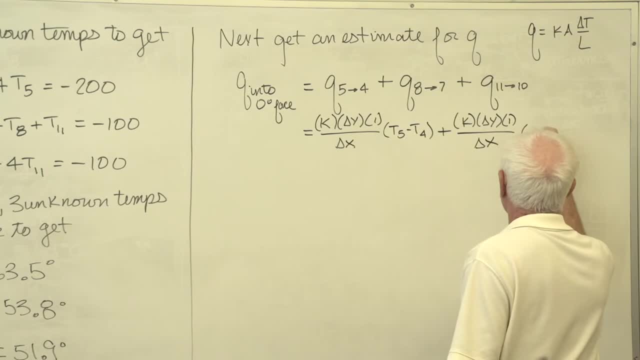 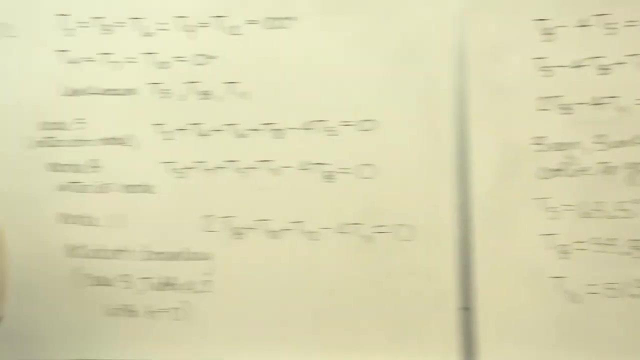 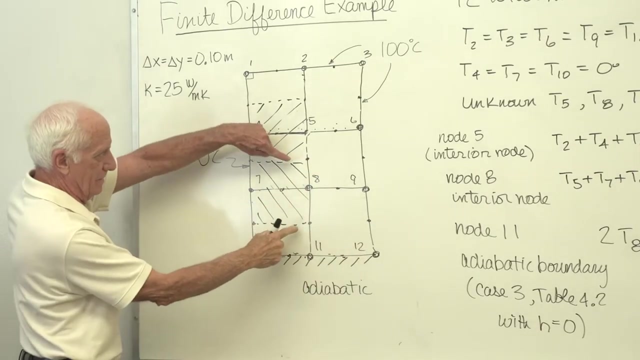 delta y times 1, delta x, T8 minus T7, plus. now you got to be careful. So okay, let's do eight to seven. first There's eight to seven, But now 10,, 11 to 10,. 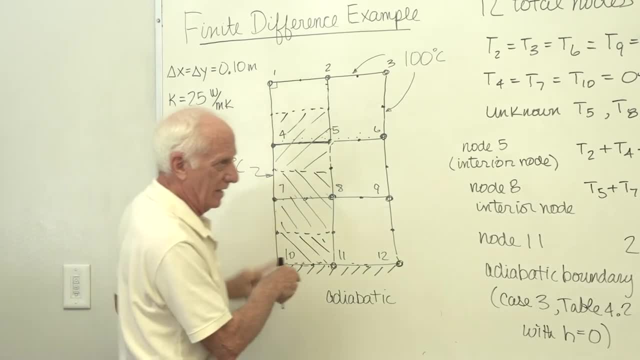 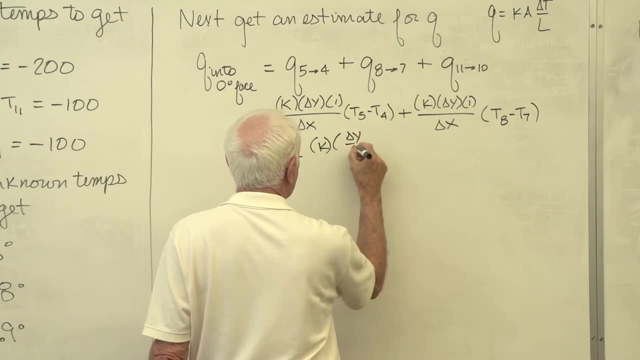 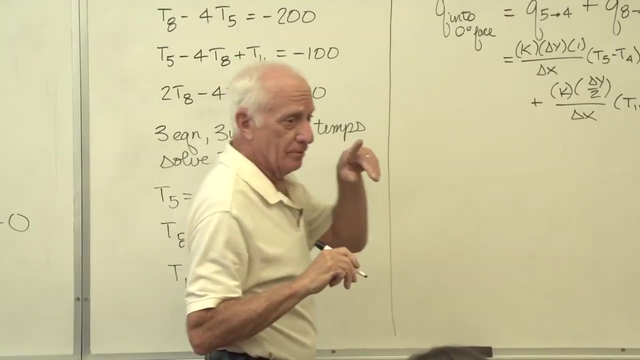 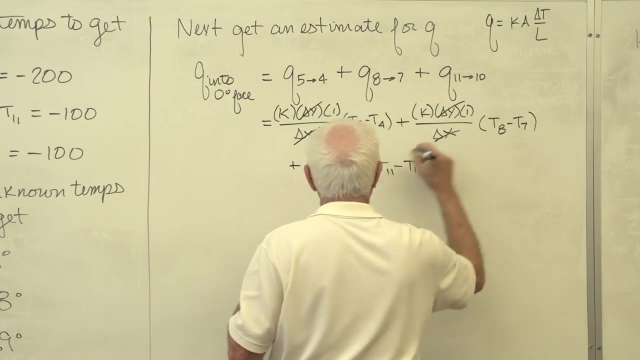 the area is half half of y, So there it is. If we make the grid square, delta x equals delta y makes life easier. Cancel, cancel, cancel, cancel, cancel, oops, not k. delta y, delta x. 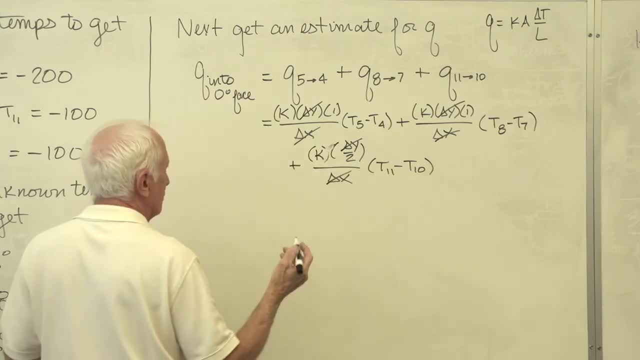 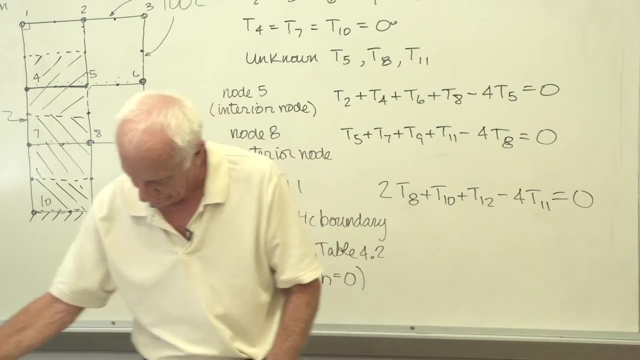 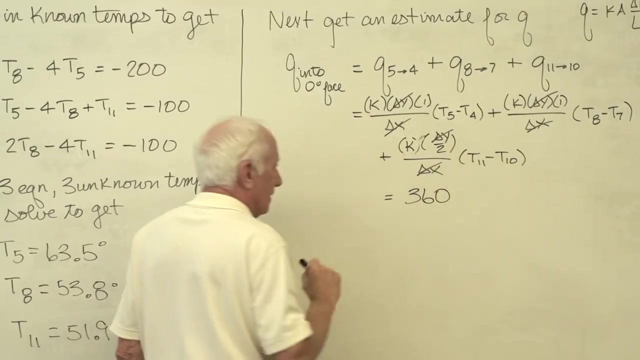 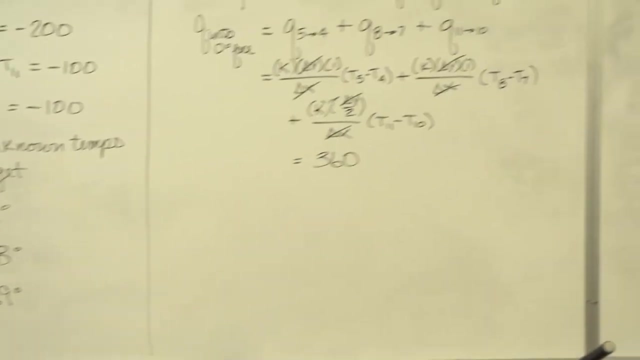 I know k 25.. I know all the temperatures. Put them in there, and q is equal to 360 watts. You say yeah, but look at this picture: The zero-degree phase is covered. We've covered that much of it. 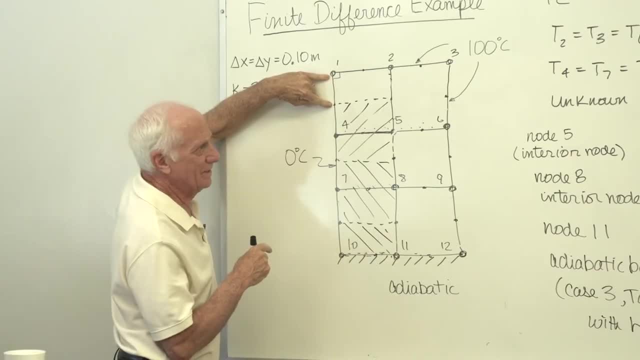 but we've ignored that much of it. We didn't account for that right there, I know That's why, my course it's because my grid is so coarse. If I want to get a better q, I'm going to put more nodes in here. 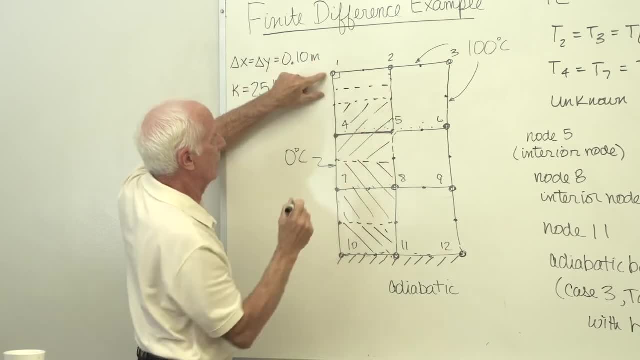 and I'm going to reduce this now to this much area that's unknown by having the grid size. If I have the grid size, this will be ignored. This will be accounted for. Say yeah, but I want a better answer. 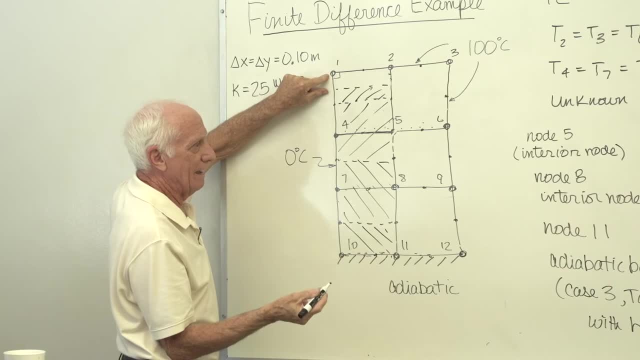 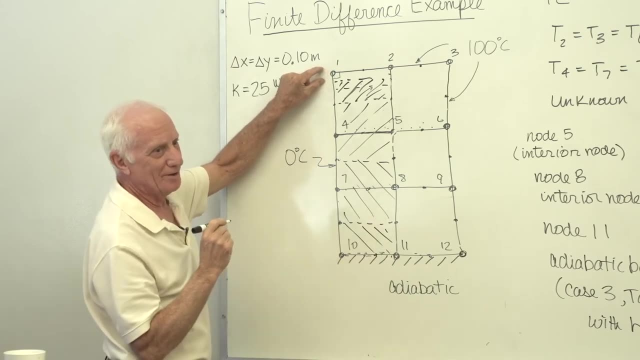 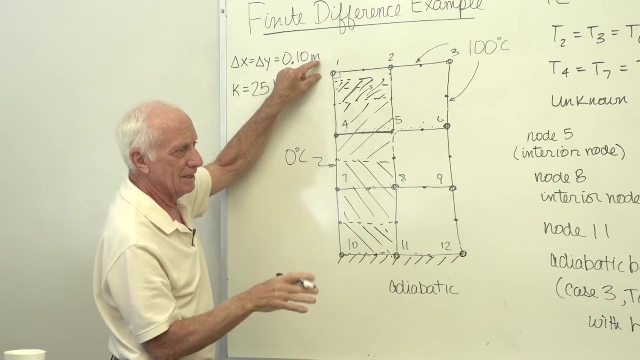 Okay, Make more nodes, Have it, Have the spacing. Now you're ignoring this little piece. You get better and better estimate of q as you make the grid finer and finer. at the cost of what Computing time? Now, what comes out of? 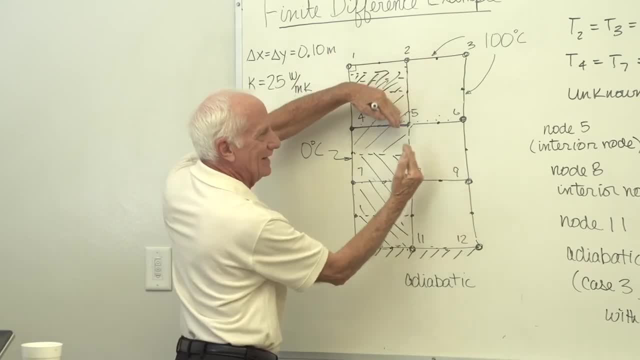 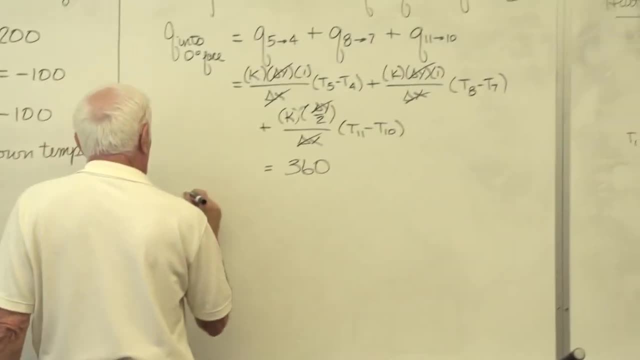 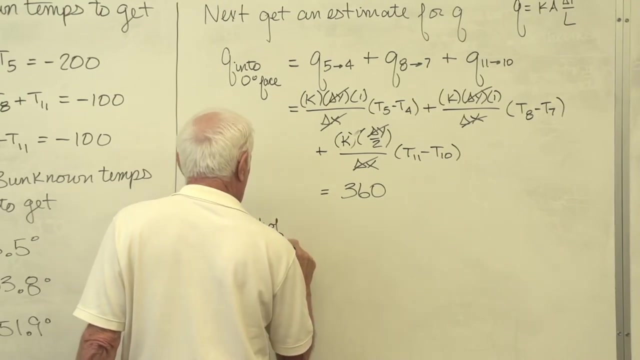 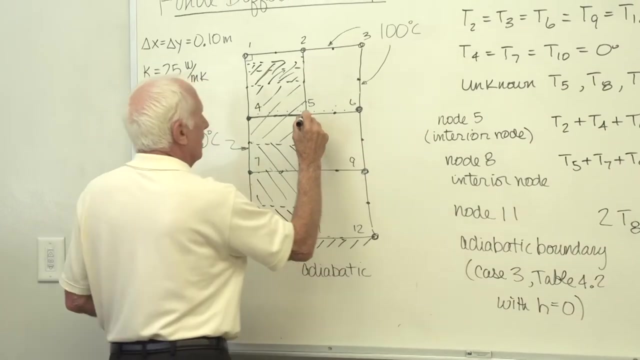 the zero-degree phase should have come in the top and right-hand sides. What comes in Here in steady-state should go out here. Okay, Let's try that then. Q out of 100-degree phase. All right, Look at the heat conducting rods from five to two. 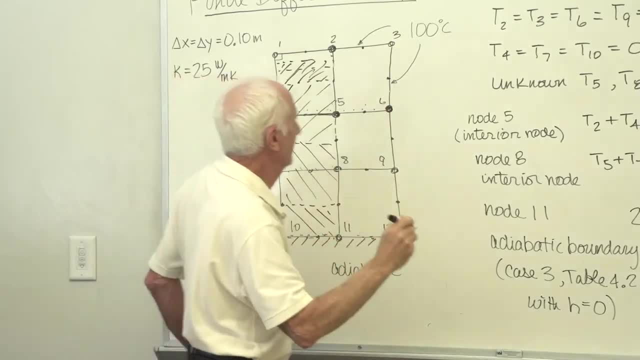 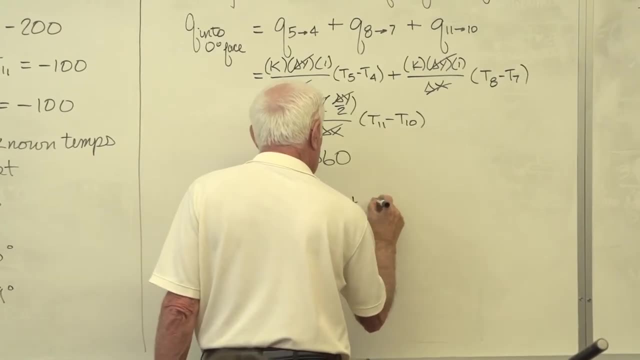 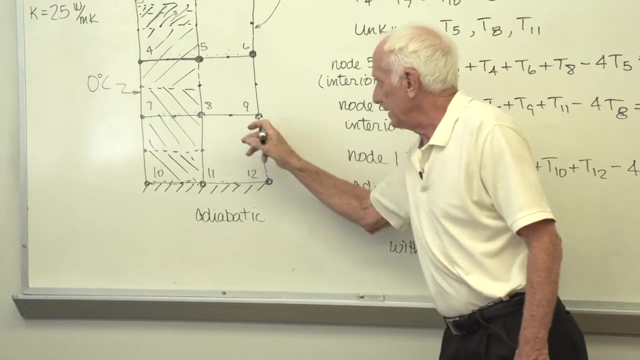 from five to six. Okay, Let's do five to two first. Well, q five to two Plus q five to six, plus q eight to nine. I'm sorry It should be six to five, nine to eight. We've got five there. 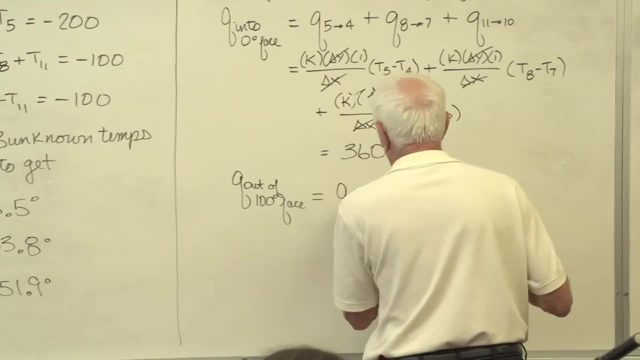 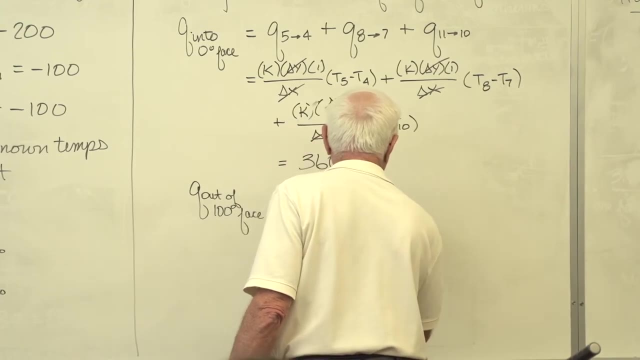 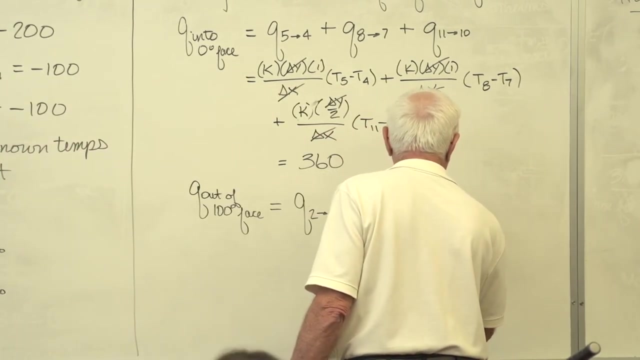 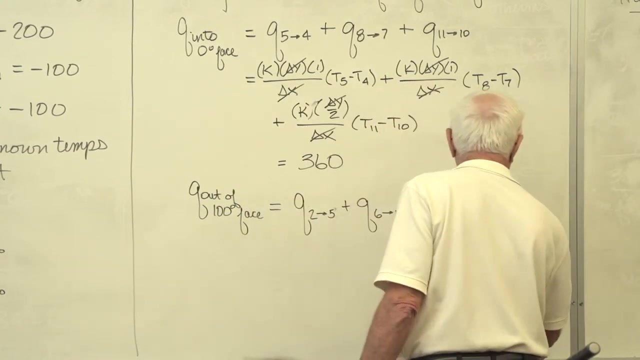 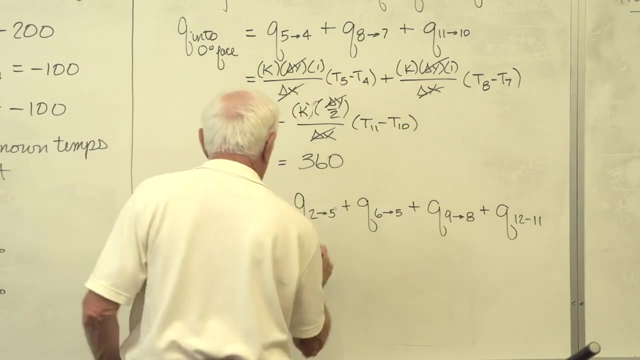 So the hot temperature is two to five, six to five, two to five, six to five, And then we have nine to eight, and then we have 12 to 11.. I'm not going to go through that. Do it the same way I did it here, when it comes out to be 356.. 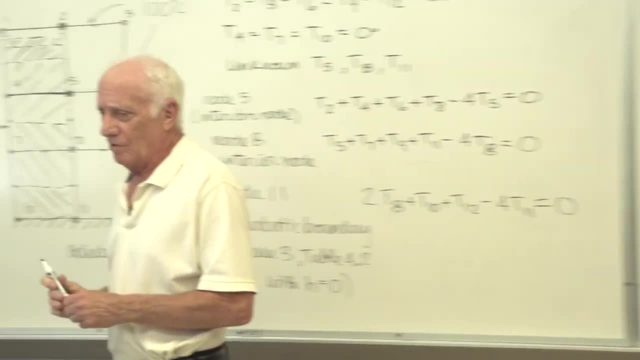 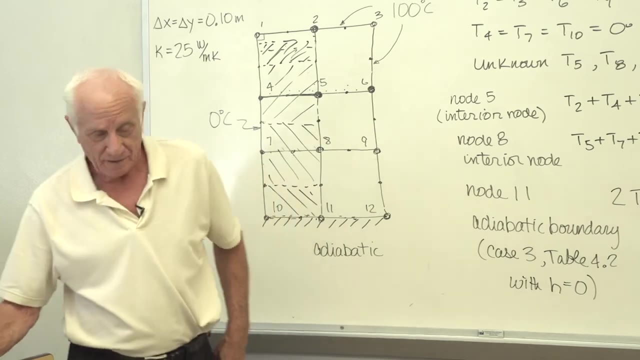 Yeah, I know they're not equal, because my grid size is so coarse. I'm surprised it's that close actually. I'm very surprised it's that close actually. I mean. so what's my answer? Add them together and divide by two: 358.. 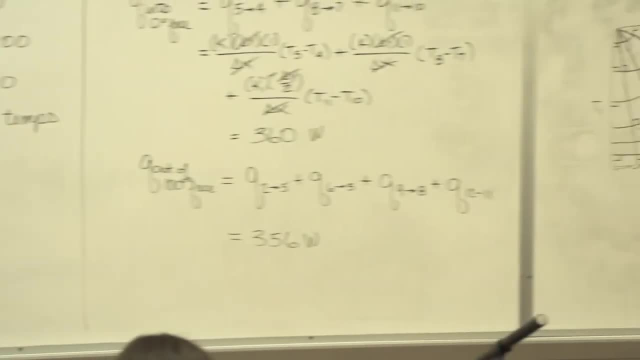 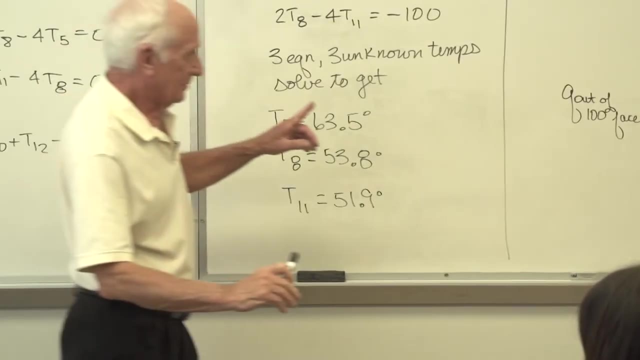 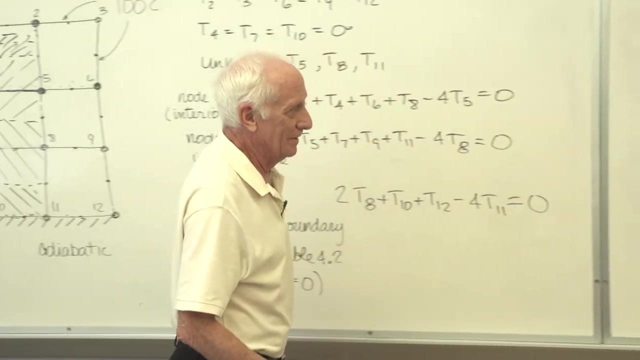 That's my answer of what q is. That's my approximate answer. The finer your grid size, the closer they're going to agree. But again, at the expense of what computing time is it worth it? And that's your call. 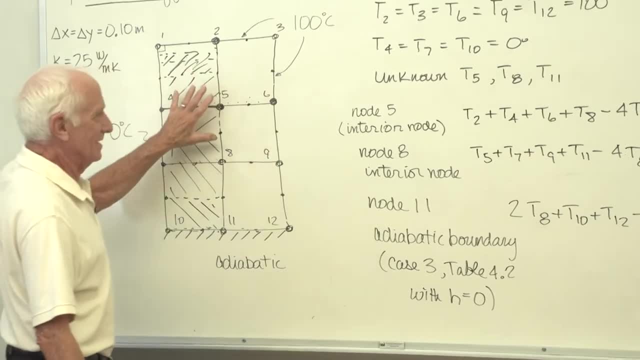 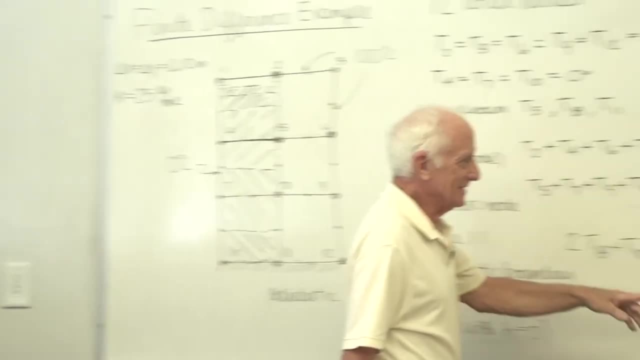 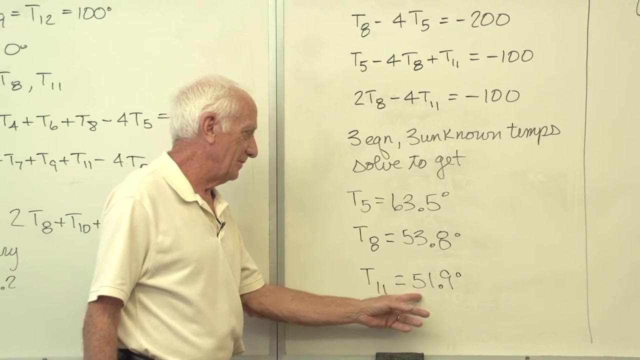 Okay, The finer you make the grid size, the more accurate your temperatures are and the closer q is to the actual q. These guys here. no, that nine means nothing. It might be anywhere from 51 to 53, that temperature. 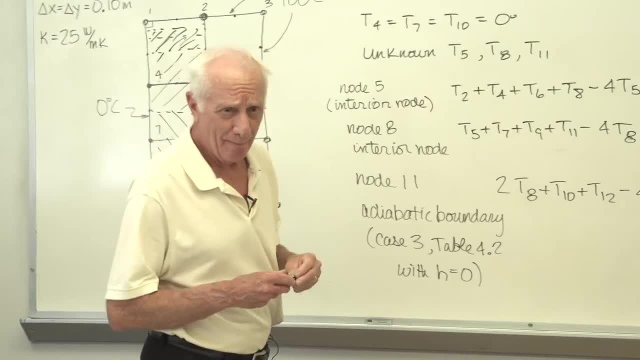 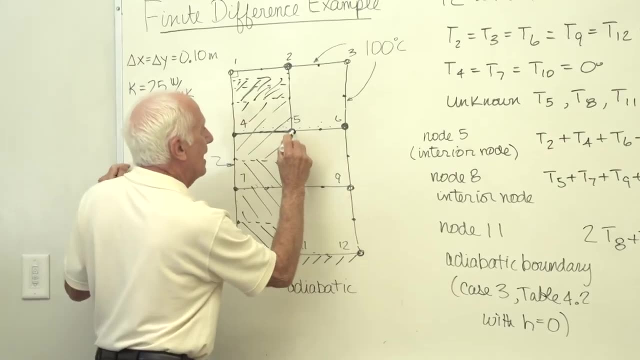 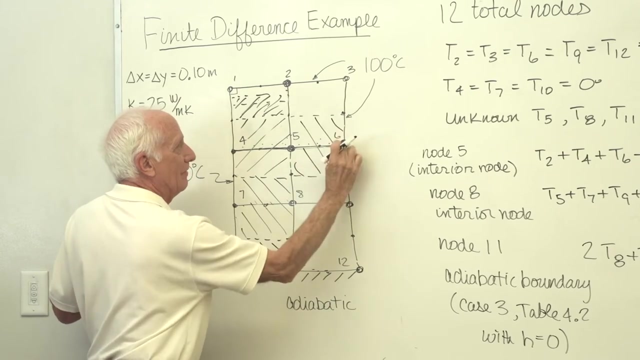 Okay, Any question on this then? Yes, sir, Why do we start in between the boxes again? Yeah, Let's take six to five. This rod replaces. how much material, That much material. All the heat from here to here is called q65.. 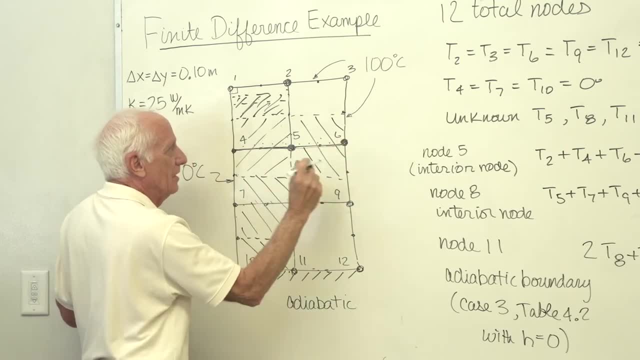 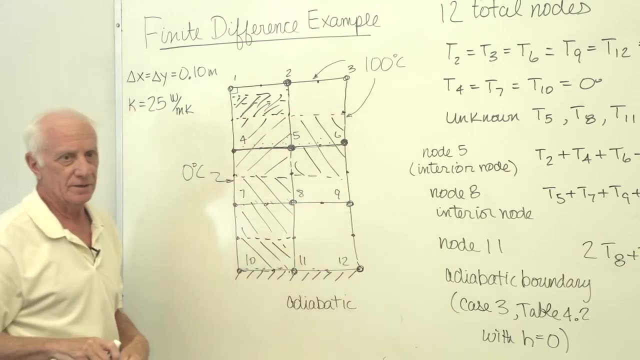 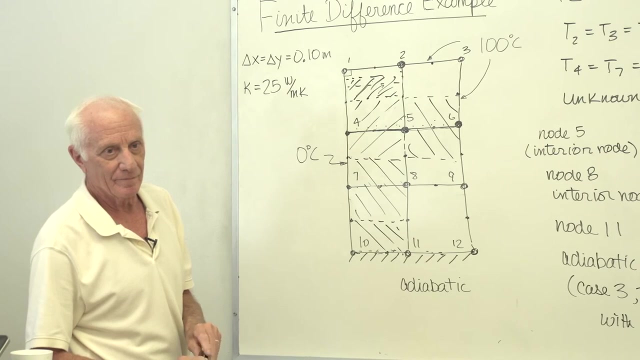 It's replaced by a symbol. node six to node five: How high is this? Delta y: How far did he travel? Delta x: Okay, That's how you do it. So is it just theoretical or not theoretical, but how you're in between two to five and then one to four. 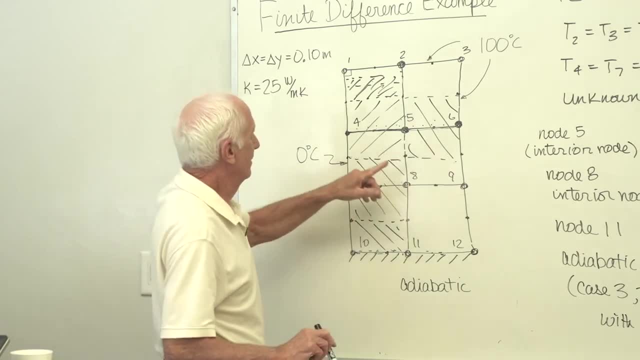 that's arbitrary. Wait, two to five, and what now? So they're in between two and five and then one to four. Yeah Right, That's just arbitrary because it's just going to cancel out, right. There's one here. 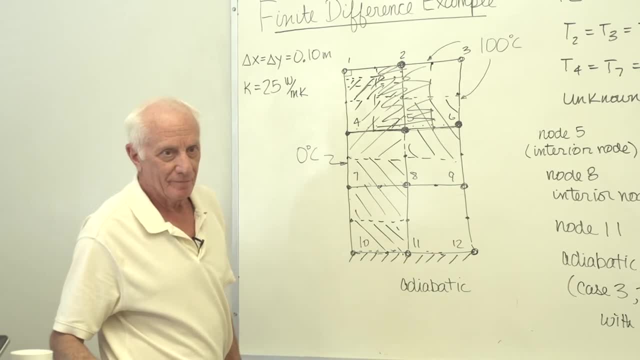 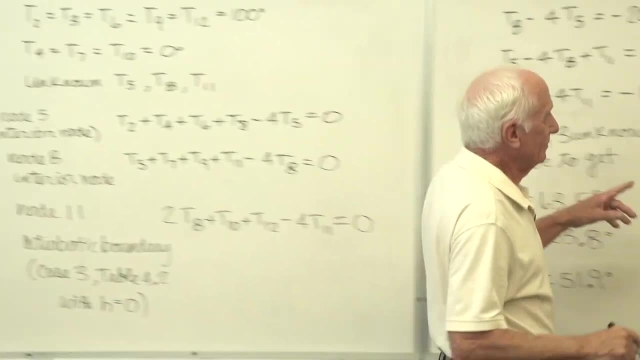 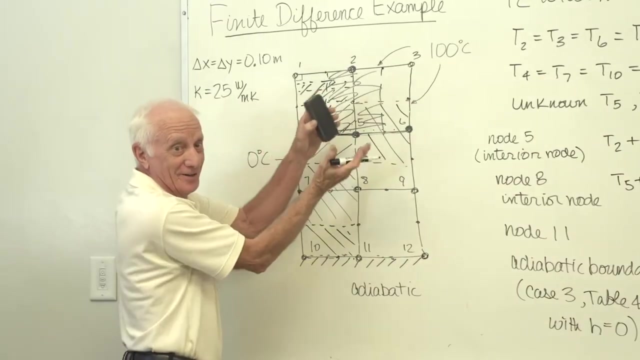 So how high up is it going to just equal What's equal to one another, Like how you created the equation where, like the Delta y and Delta x, it ended up canceling out. Yeah, Otherwise things would change. These would change. You want to make it life easy? 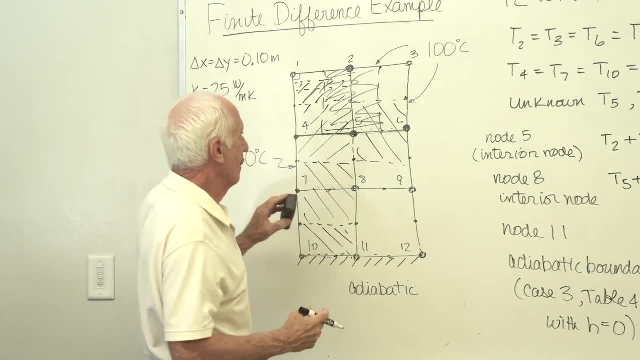 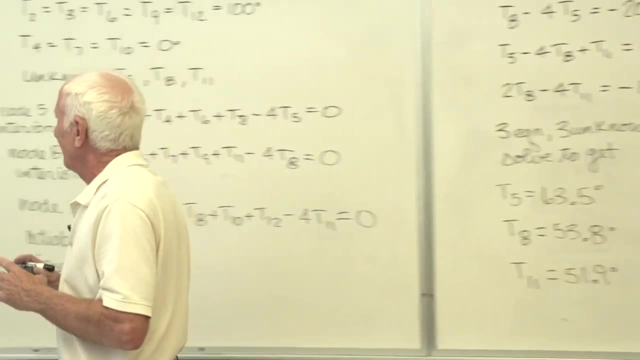 so you try and make Delta x equal Delta y. Yes, sir, So for finding the q out of a face, you just need to be adjacent to that face, right? Here's what you have to do. You see, you say well. 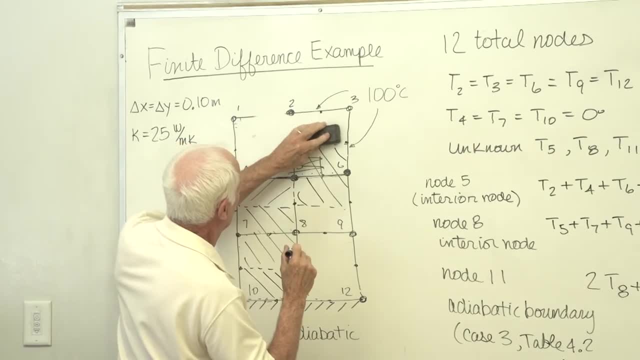 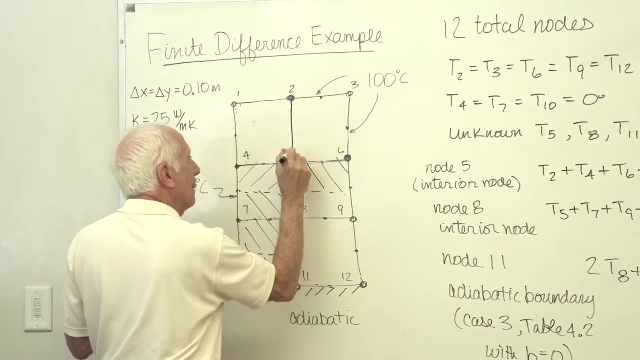 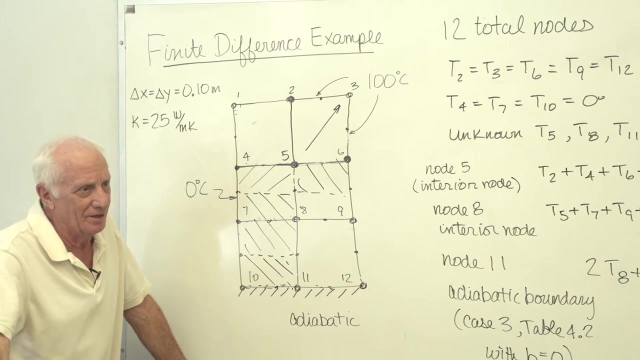 it looks to me like how about heat going that way? I say no, illegal. illegal Heat only is transferred along heat conducting rods. Is there a rod from five to three? No, Okay. Is there a rod from five to six? 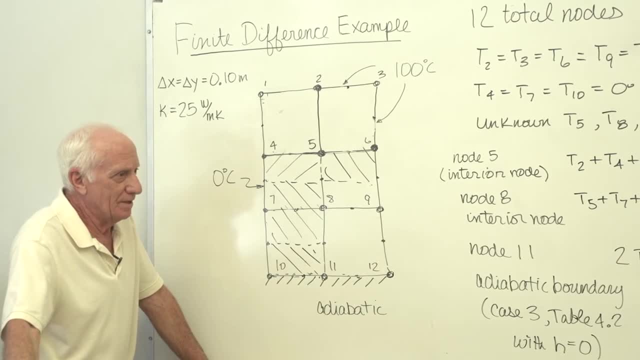 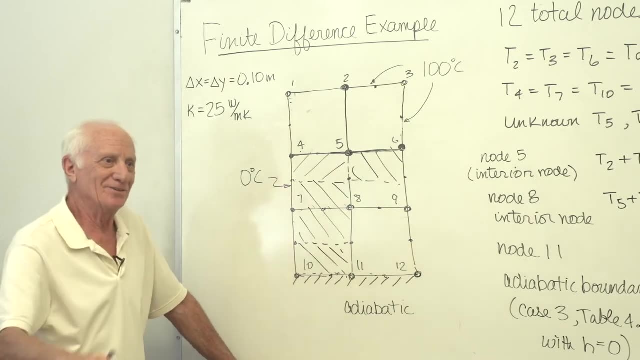 Yes, From five to two. Yes, All the heat is conducted along those guys There. When you draw this picture, these are the heat conducting rods. Now, is that something else? you had a question? Yeah, So if you had even smaller nodes? 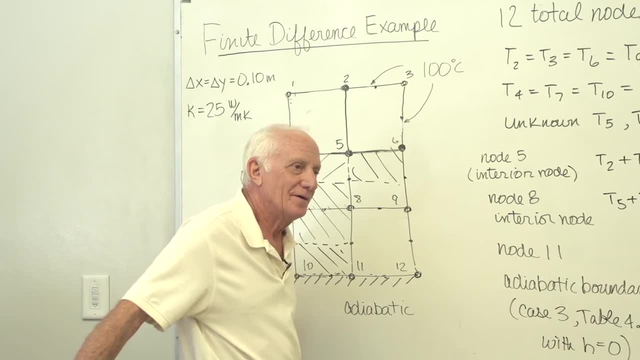 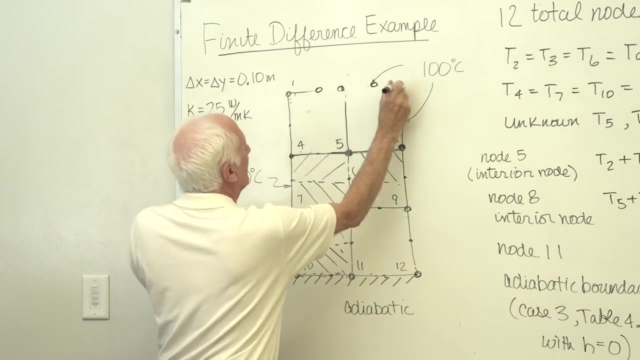 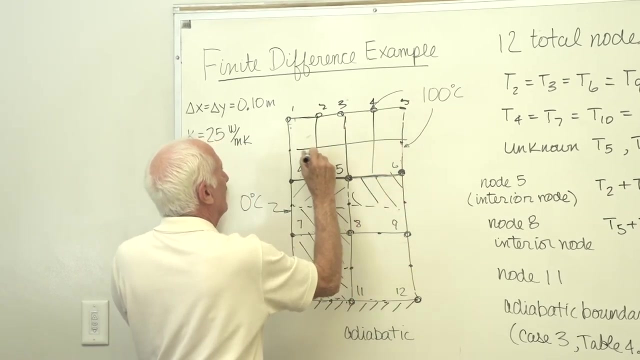 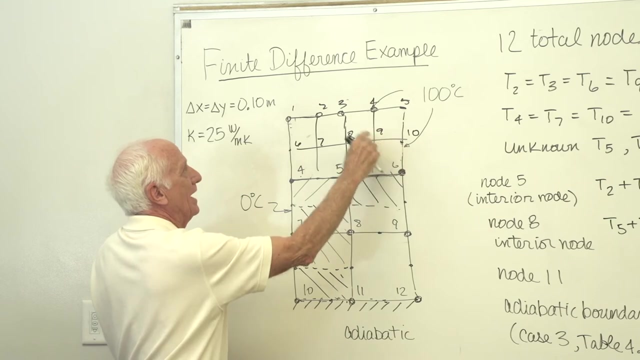 so say you had like five going this way, would you use so the one, two, three, four, five. would you just use five to four Along here? Yeah, Like the top, Yeah, Yeah, Okay. Four to nine, three to eight. 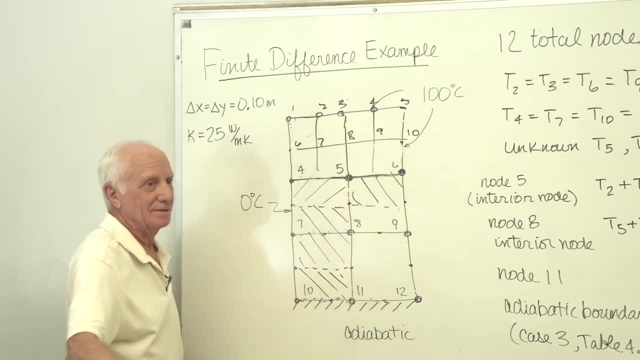 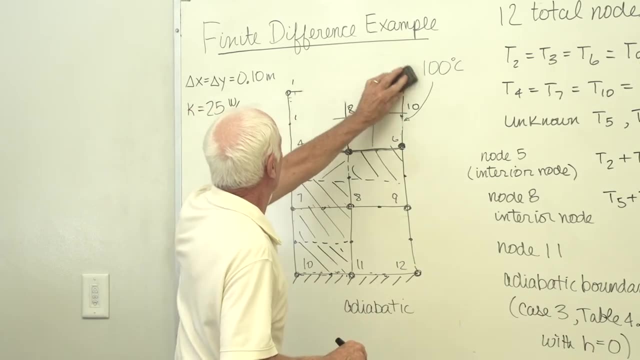 two to seven, ten to nine, blah, blah, blah, blah, blah. Yeah, Yeah. So how can we ignore two to one? Okay, I got it, Yeah, Okay. I'm not sure if you mean that's real. 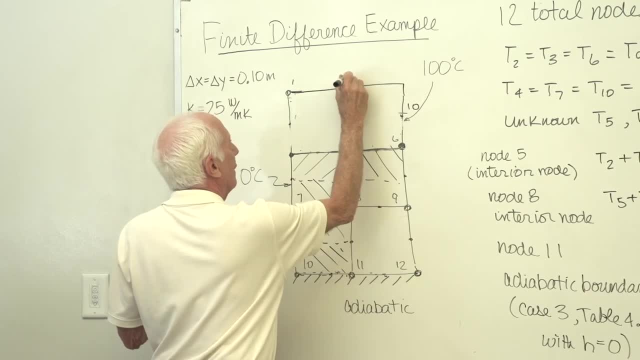 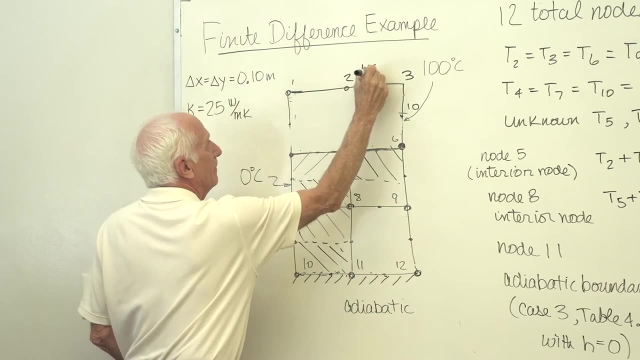 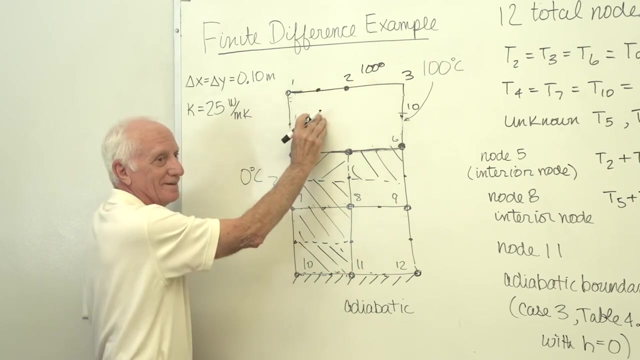 Yeah, Yeah, Okay, That's a good question. What's the temperature here? A two to a hundred. What's the temperature there? It's a temperature right there, a hundred. Problem said, the top surface is at a hundred except the corner. 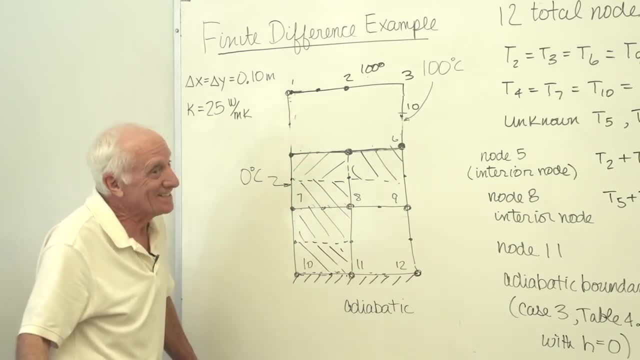 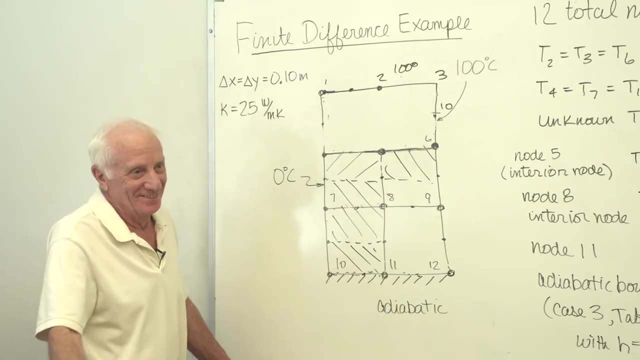 That's what the problem says: Okay, Okay, Yeah, It's got to say that. It's got to say that: Yeah, Over here the left-hand face is zero, except right there, illegal. I thought it was an assumption. 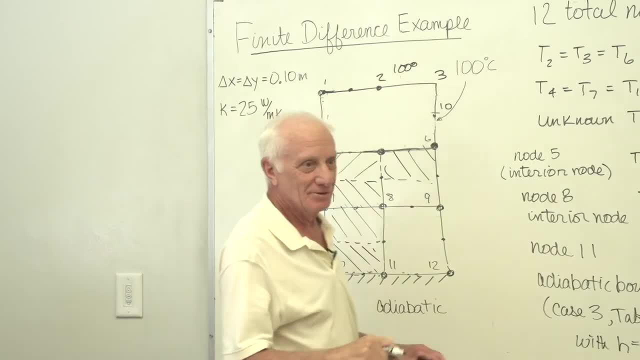 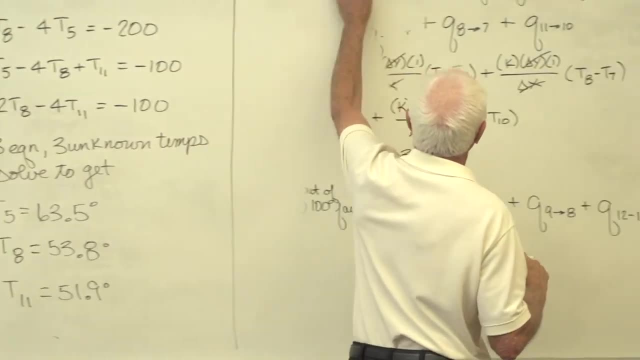 Yeah, No, no, It's going to say it. It's going to say it in the problem. Okay, Was there another question? Okay, Yes, sir, If you draw the box for the area that it replaces for six to five. 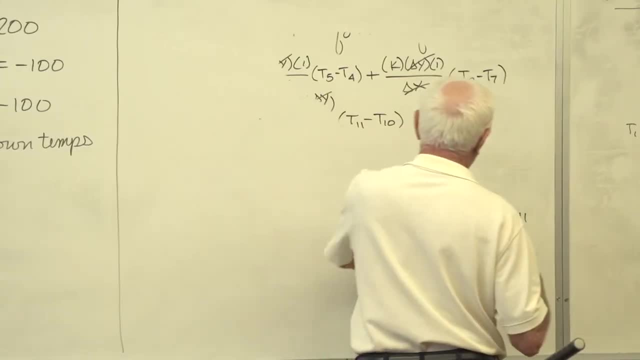 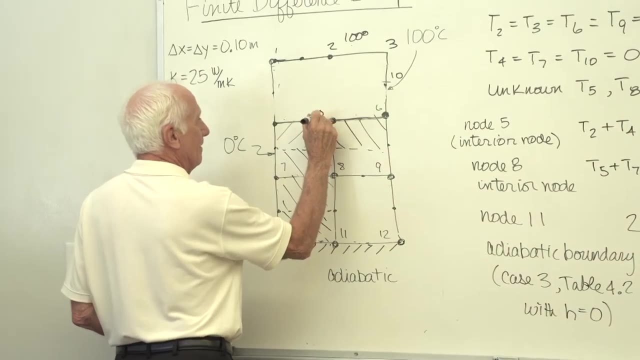 Six to five? The original one, Yeah, Uh-huh. And then if you draw the box for two to five, they overlap by Six to five. Yeah, This was five. Yeah, Okay, There's six to five. Which one? Yeah, They overlap. 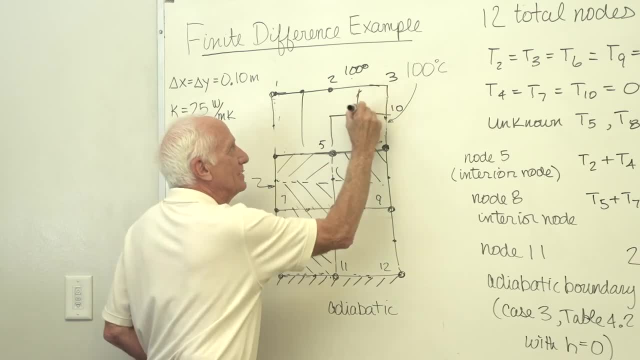 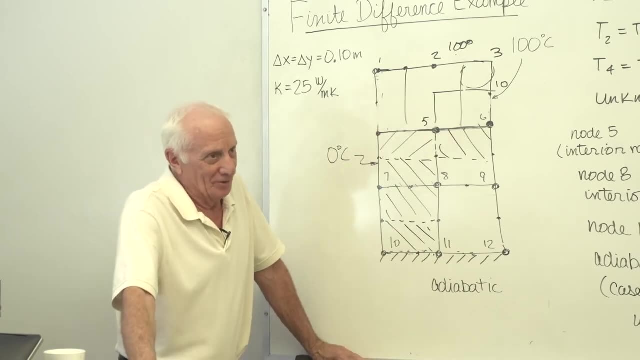 Yeah, You got it Right In a way. how about this area here? Conclusion: I ignored it, So I double count here. ignore that one. You know there's errors built in this thing, But guess what, As you keep reducing the grid size, they go away. 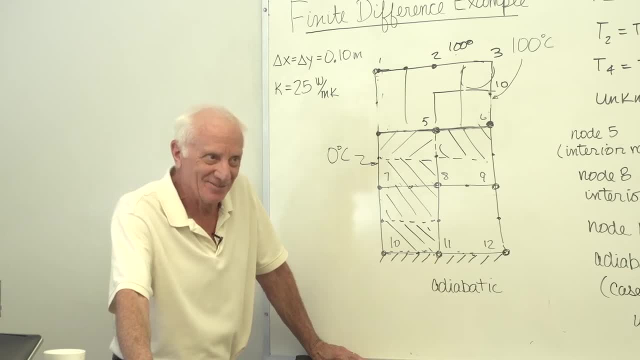 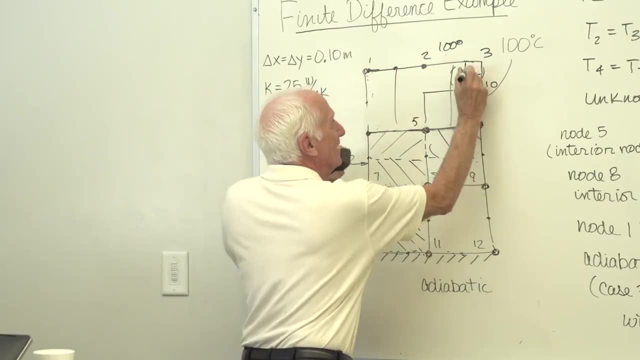 The errors get smaller and smaller. the problem: errors get smaller and smaller. That's right. Yeah, The corner starts to just this area gets smaller. now, you're missing that much. now, you're missing that much. now, you're missing that much. 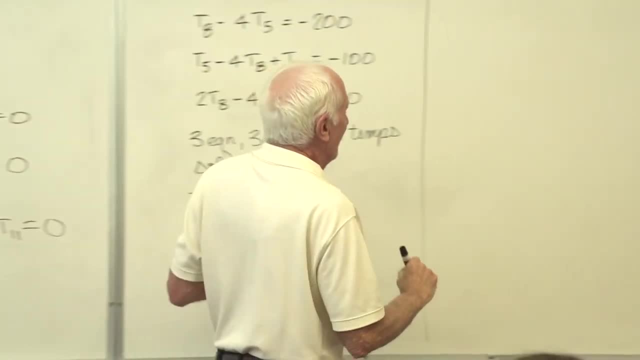 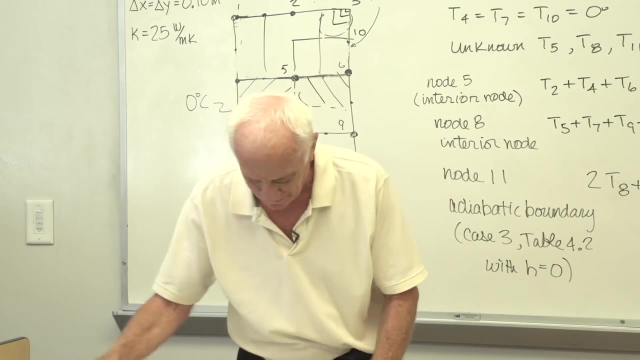 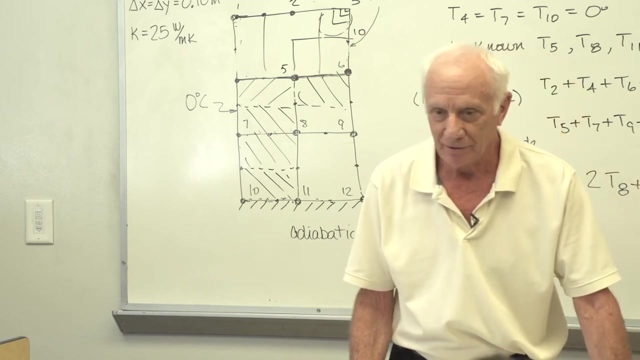 At what cost? More computing time. Yeah, That ends our chapter on 2D heat conduction. Now I'm going to go over some problems for homework. Did it get over, you guys, yet? homework? Yeah, Okay, Let me answer you please. 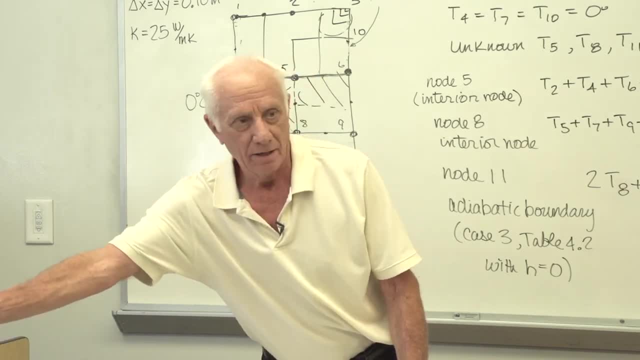 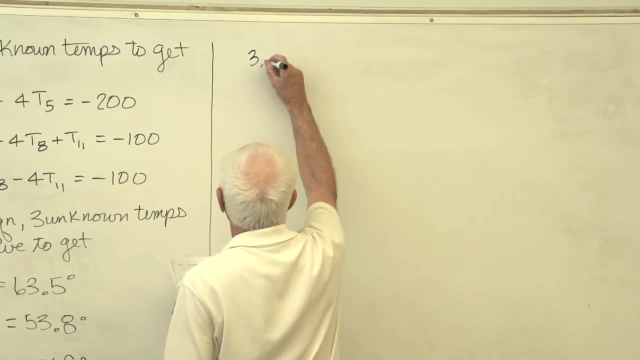 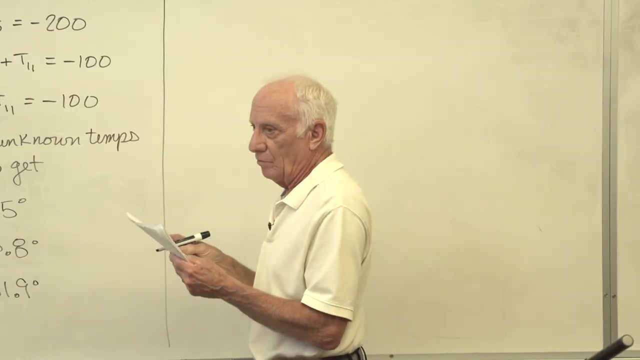 Thank you. Did anybody come in late that didn't get their homework back? Okay, Just so you know the numbers on this 315,. main problems on that was getting the correct K values. pretty much for that wall with studs, insulation, wallboard and siding. 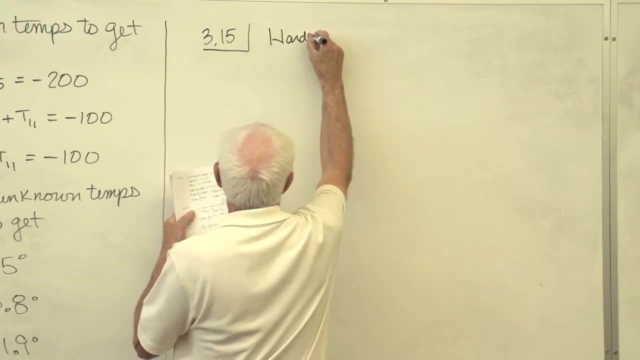 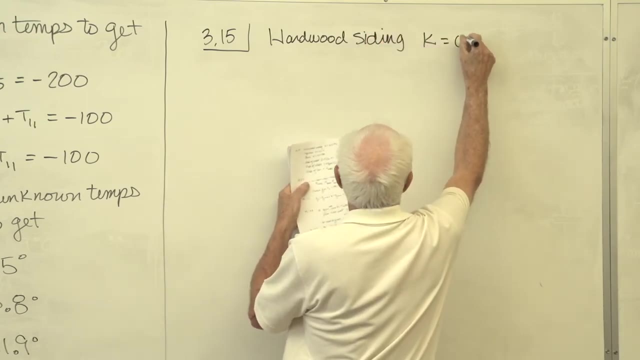 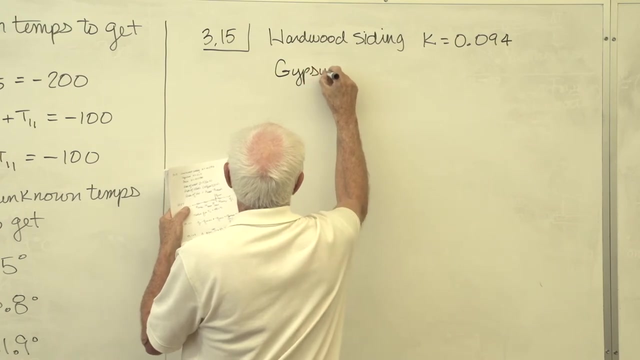 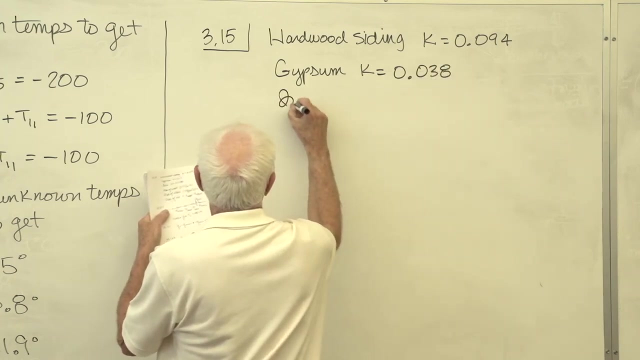 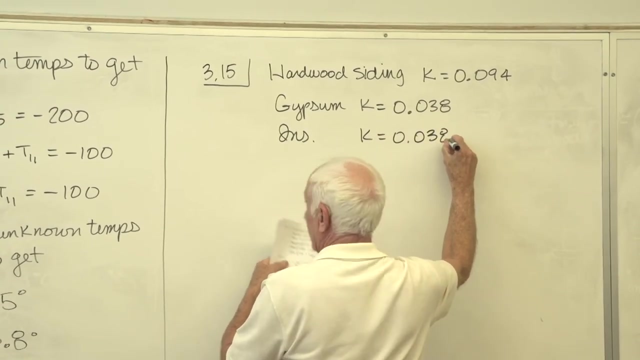 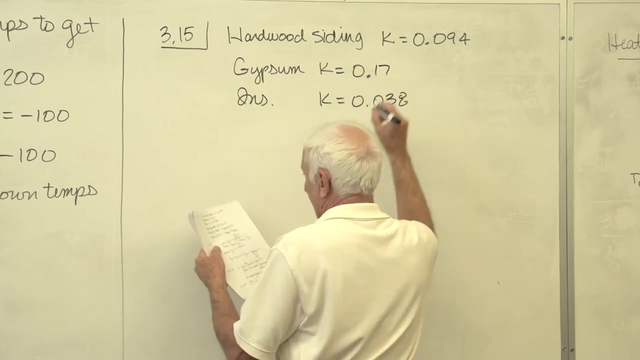 So the hardwood siding K equals 0.9.. 0.9.4.. Gypsum 0.38.. Insulation: 0.38.. This guy here is 1.7,. gypsum 0.17.. Area of the total wall. 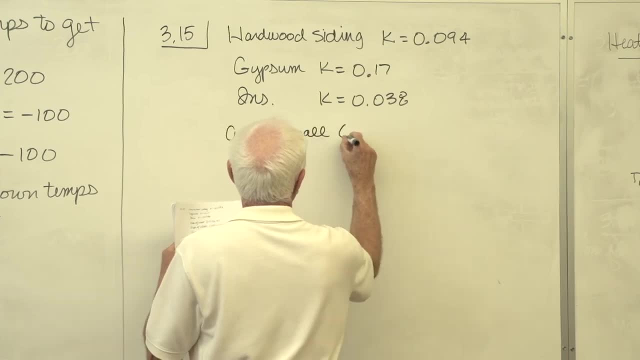 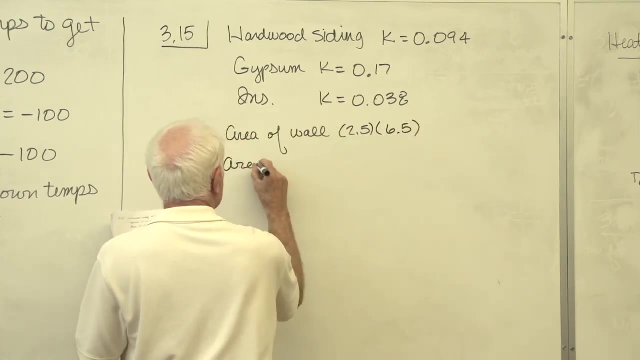 2.5 meters high by 6.5 meters long. Area of studs: there were 10 studs. Each stud is four centimeters and 2.5 high. Each stud four centimeters by 2.5 meters Area of insulation. 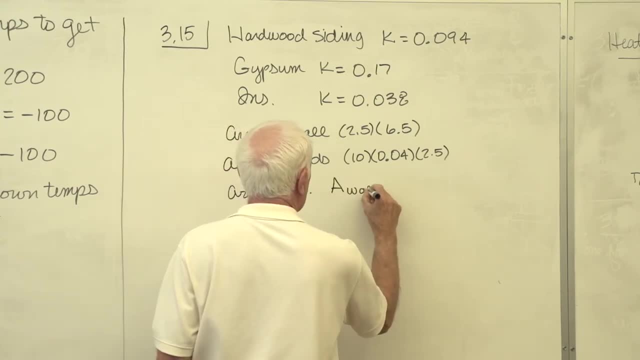 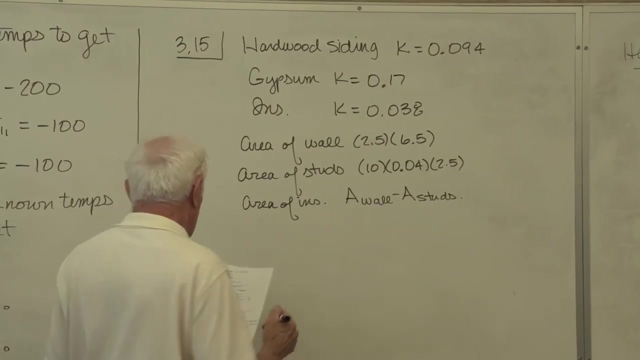 area of the wall minus area of the studs. You need those areas, of course, for your resistance. Ka over L. There's your areas. If you didn't get these K values, see me after class and I'll point out exactly in the tables where. 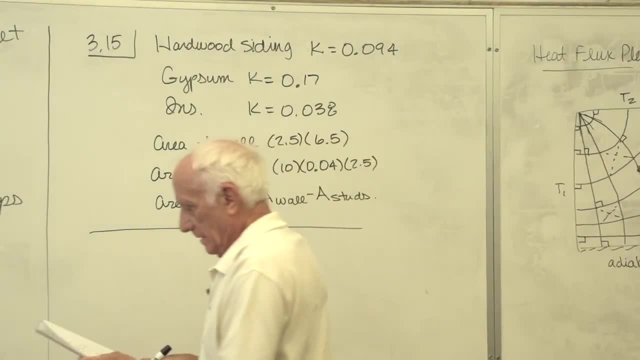 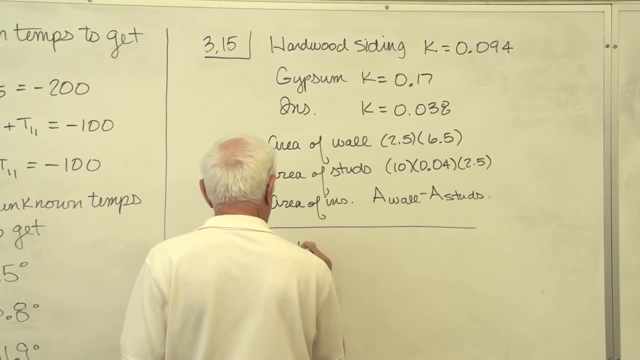 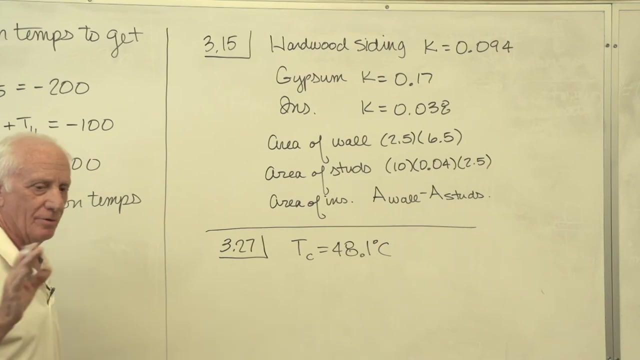 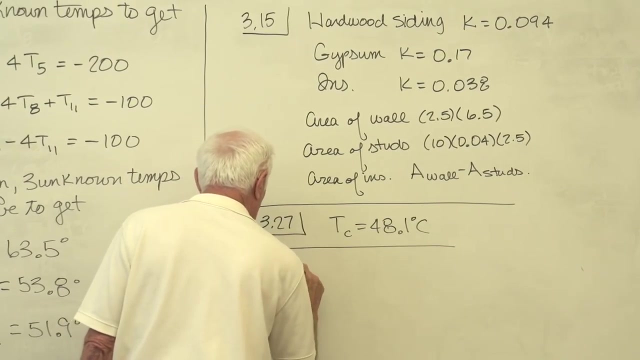 the correct value is for you. so you know: 327.. The correct answer for the chip temperature 48.1 degrees C. I think I had down 46 point something degrees C. The correct answer is 48.1 degrees C. 311 is a solar collector panel. 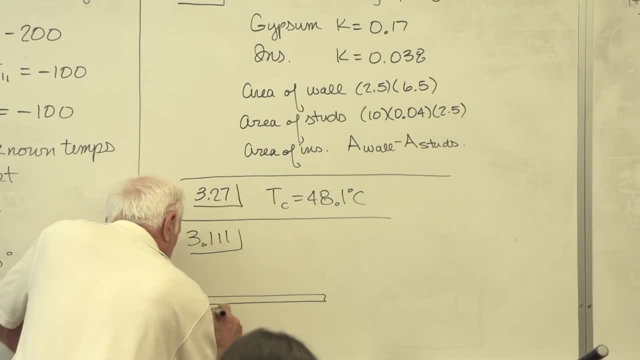 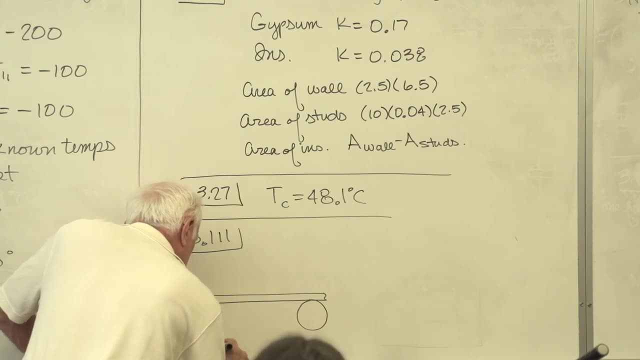 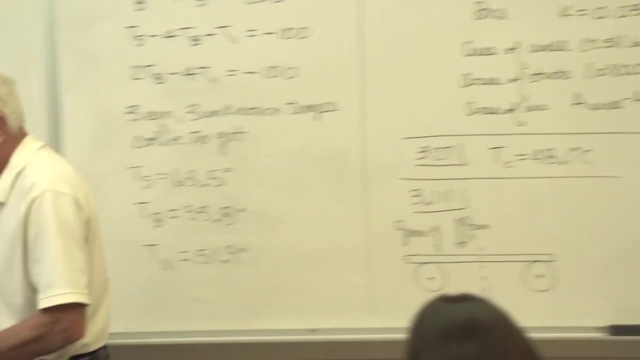 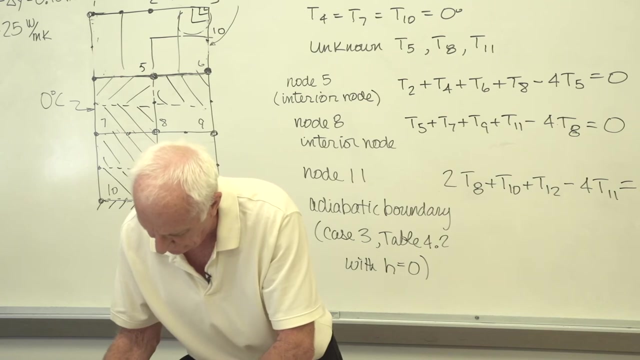 which behaves like a fin. There's two tubes carrying a fluid, generally water. x measured from here, L is halfway. There's convection coming out to the air. There's radiation coming in from the sun. The way you start that problem is to go back to fins at. 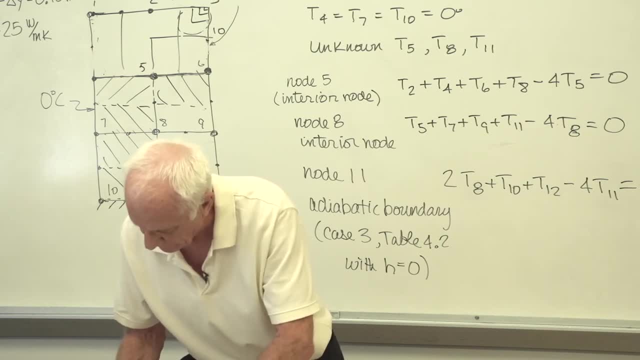 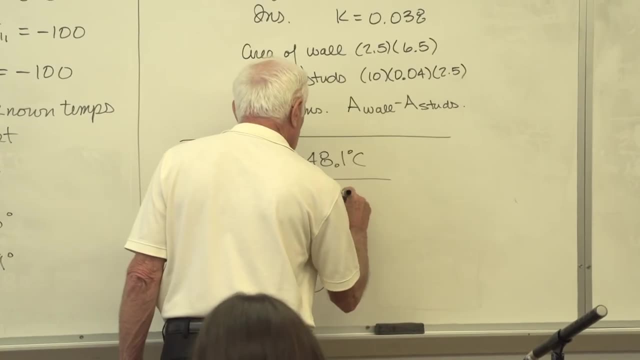 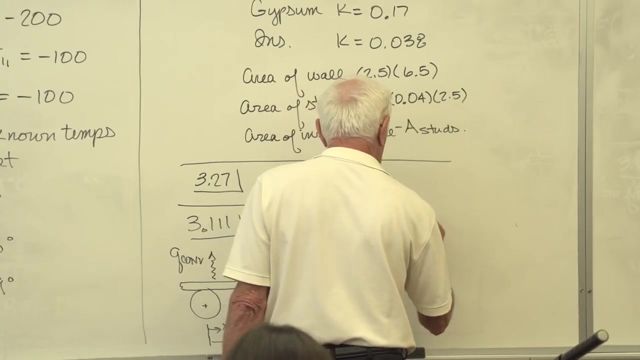 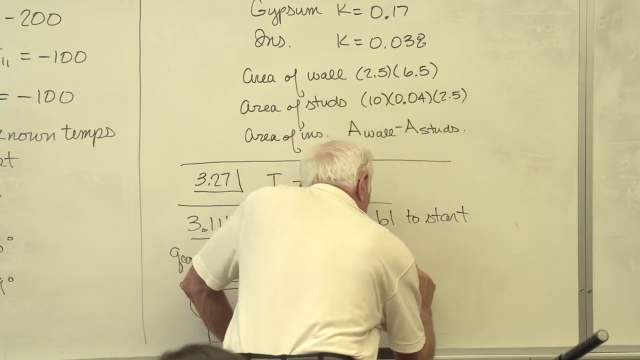 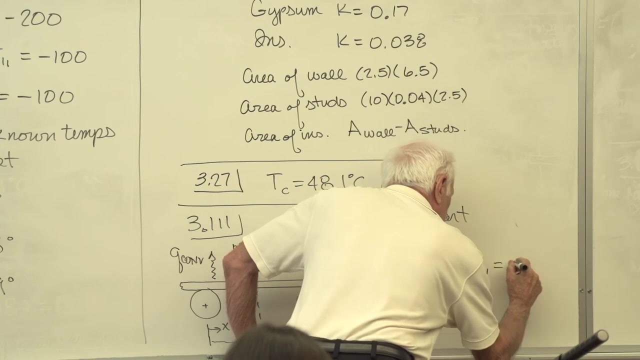 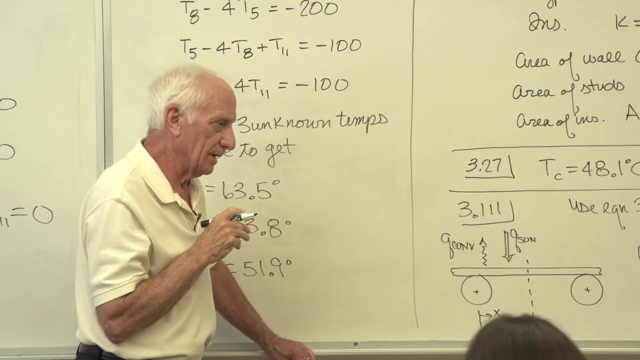 the derivation of the fin equation for temperature, which is equation 361.. 361.. 361.. and you have qx minus qx plus dx minus q. convection equals zero. That was equation 361.. We did that in class. We took a small differential element. 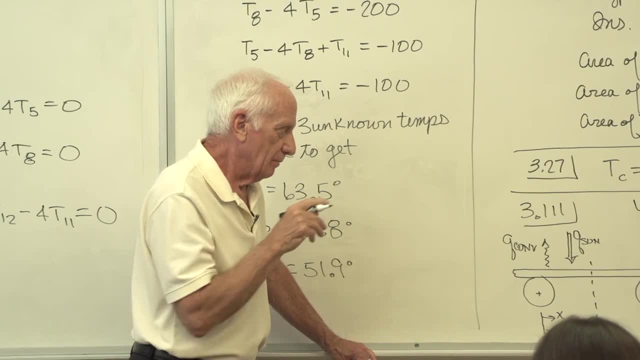 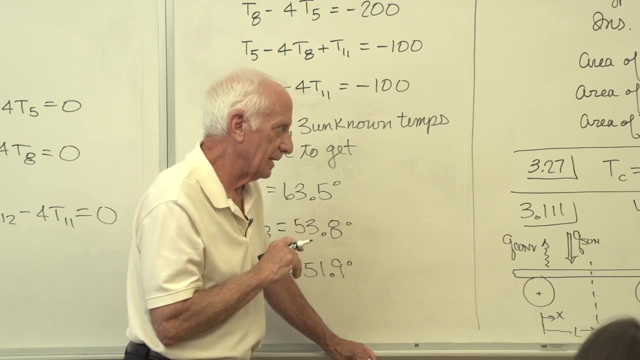 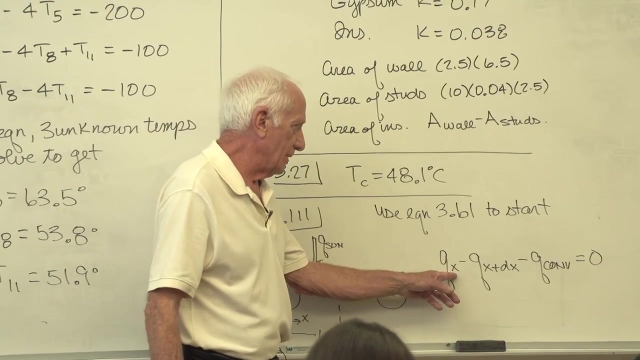 of length, dx, out of the fin. We wrote that equation, energy balance on it. From that we got a differential equation relating temperature as a function of x In words, heat coming in the left side of the element by conduction qx. 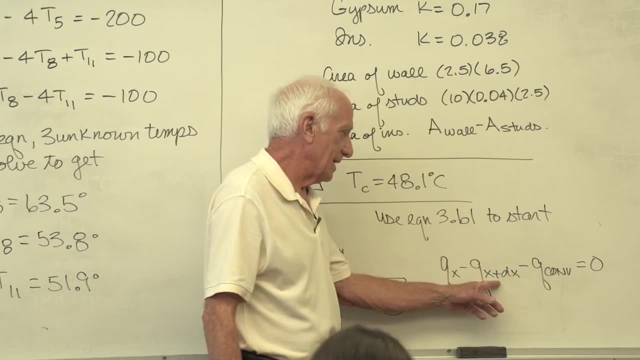 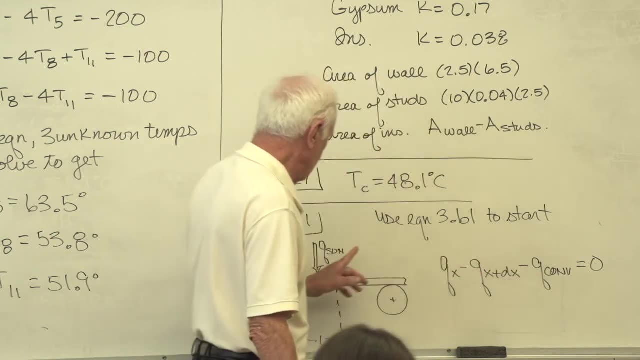 minus heat going out the right side of the element by conduction: qx plus, dx minus the heat loss by convection to the fluid at t infinity. Now what's the difference here? You see the picture. The difference is: I've got to. 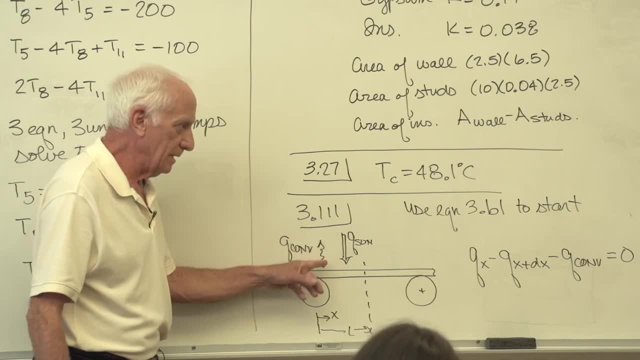 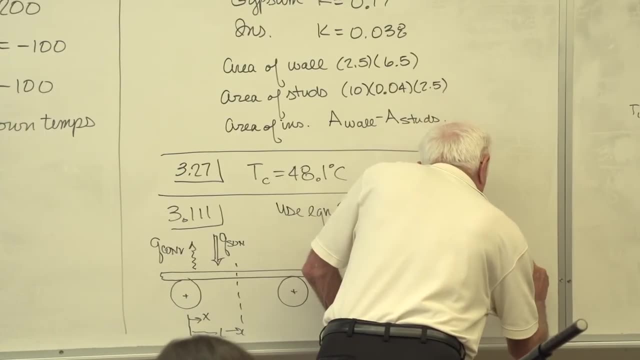 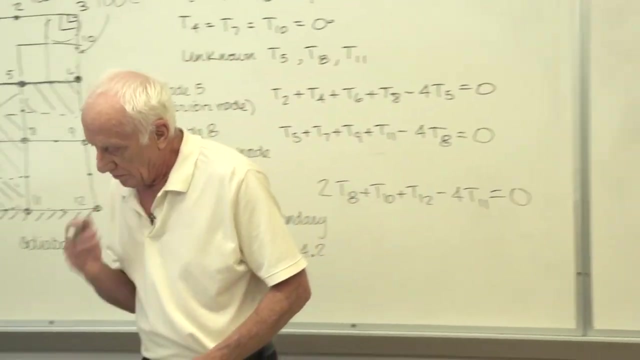 throw in q sun as an input, It's coming in. Coming in means positive, So this becomes plus. q sun equals zero. That's a constant. It's just a constant. q sun is given as a constant. You then follow what I did in. 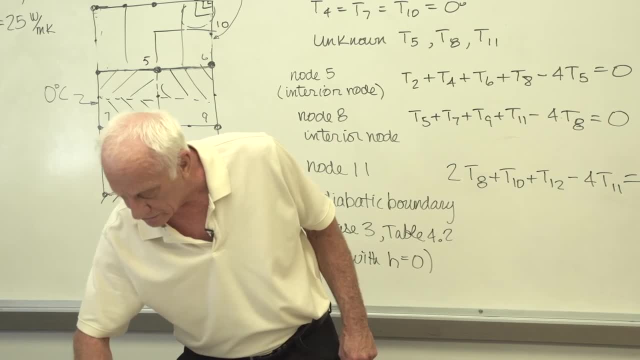 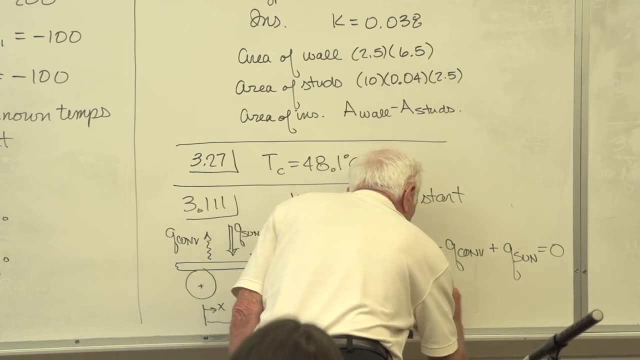 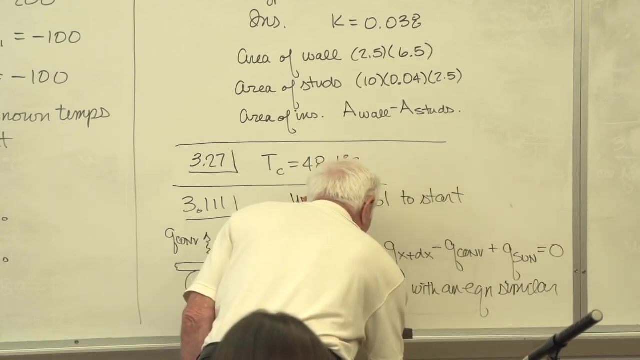 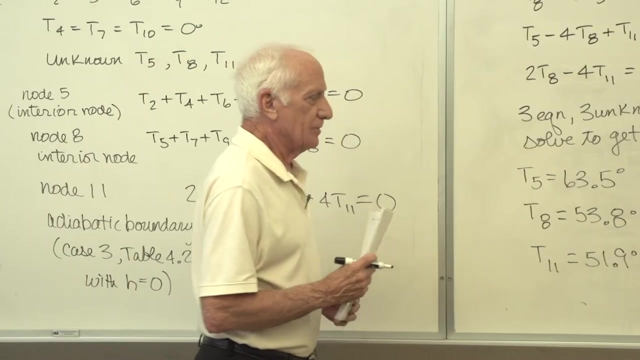 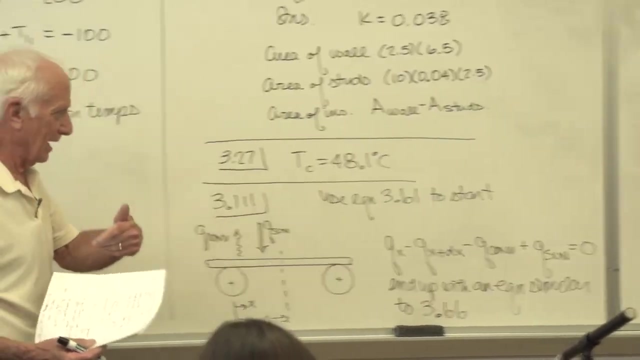 class or in the textbook on that page, until you end up with an equation similar to the 366.. Which is the governing differential equation. So it's a pretty straightforward solution. All you do is throw a constant in and then follow line by line. 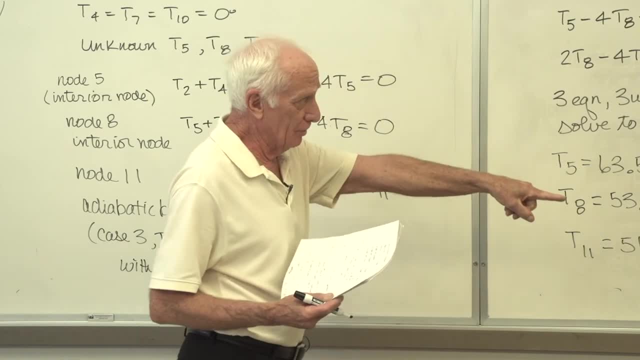 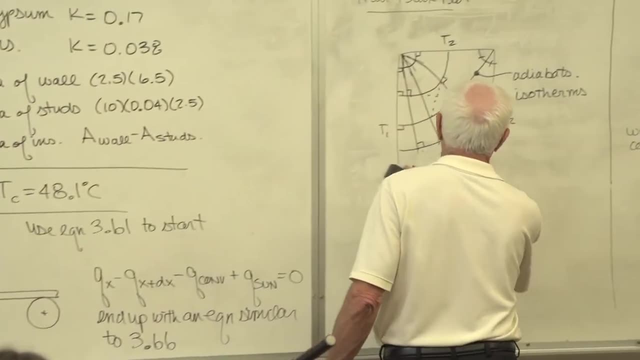 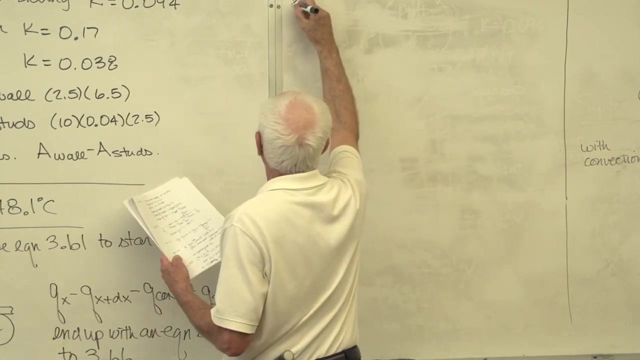 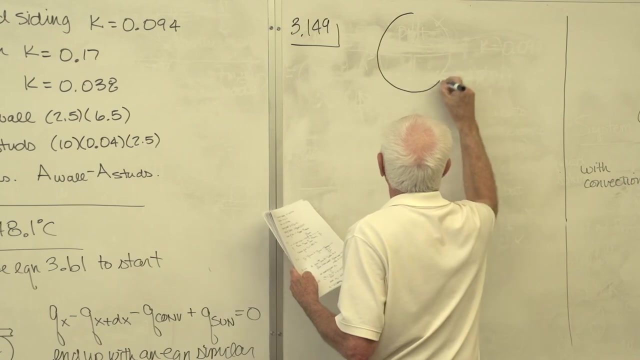 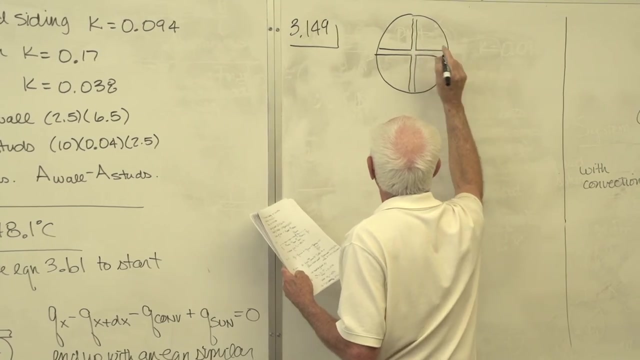 five lines what he does in a textbook to get something similar to equation 366.. Which is a governing differential equation 3149.. This was the circular tube separated by there's baffles. here there's baffles. here There's fluid. 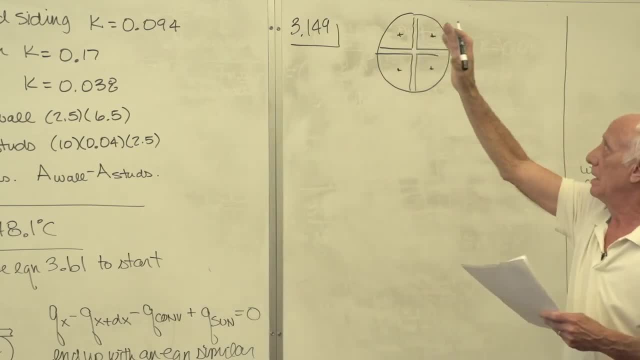 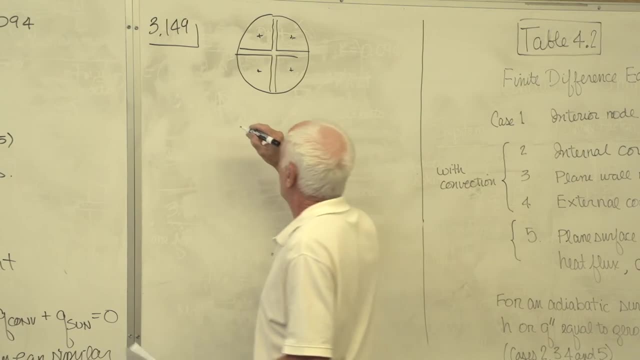 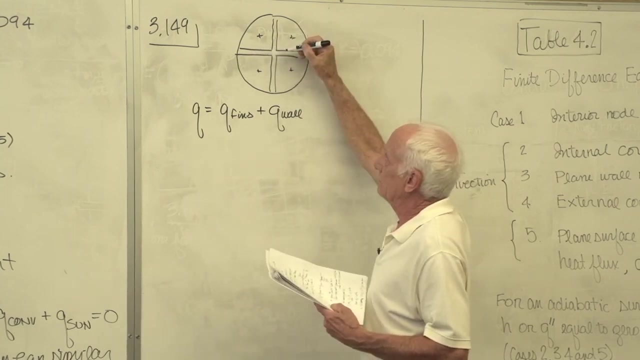 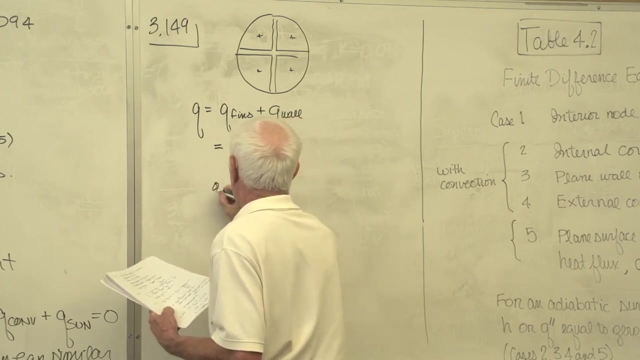 Flowing. This tube comes out of the blackboard. These are baffles, So the fluids flow in these four quadrants. So I have q, equal q from the fins plus q from the wall. These guys behave like fins. This is t base. 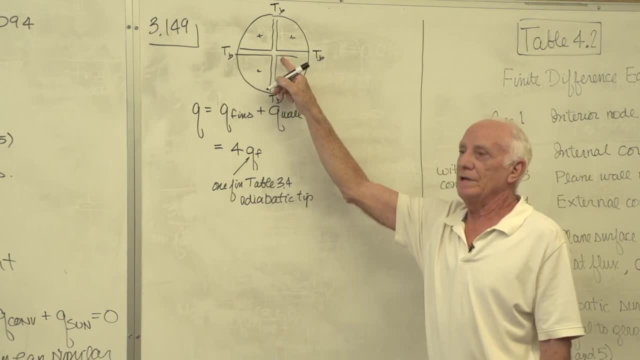 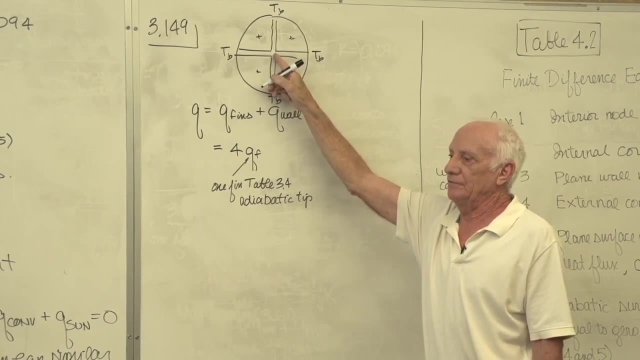 In the middle. no heat crosses horizontally, no heat goes up and down vertically. Conclusion: At this point these fins behave as if they have an adiabatic tip. Case 2, Table 3-4, find QF got it. 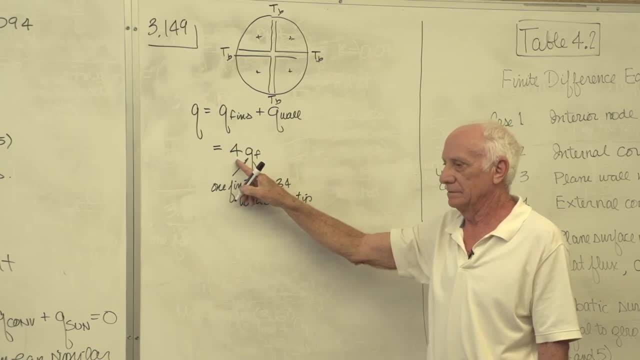 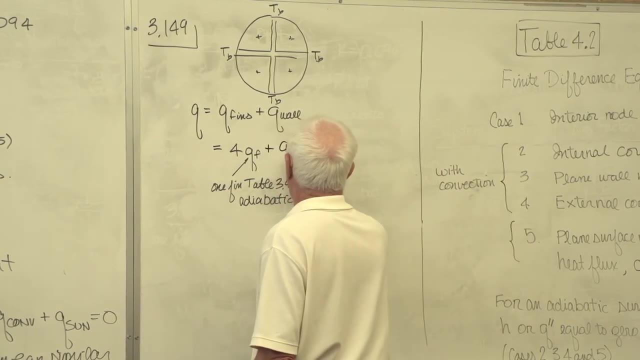 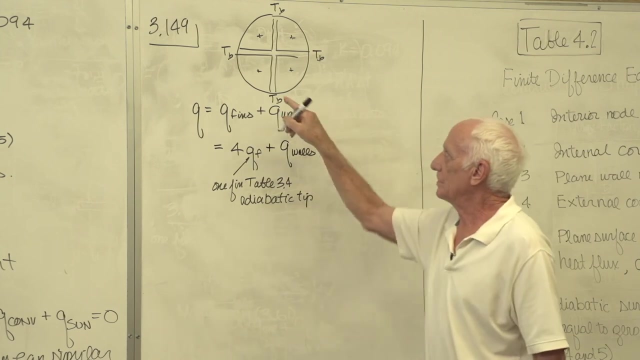 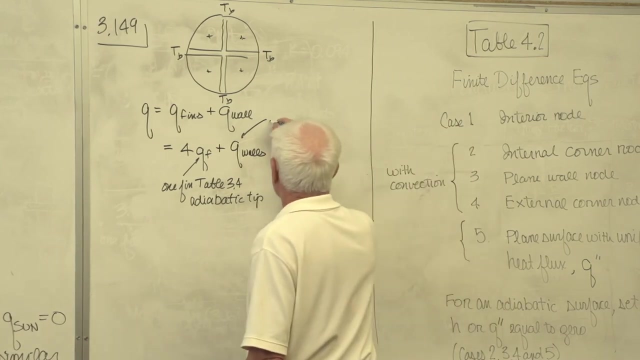 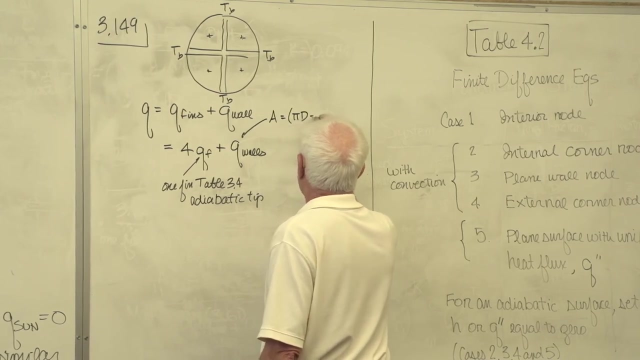 How many fins? Four got it. Table 3-4, Case B plus Q from the walls, Q from the walls: What's the total wall area? The circumference times the length, Circumference pi d. But you have to subtract out four times t. 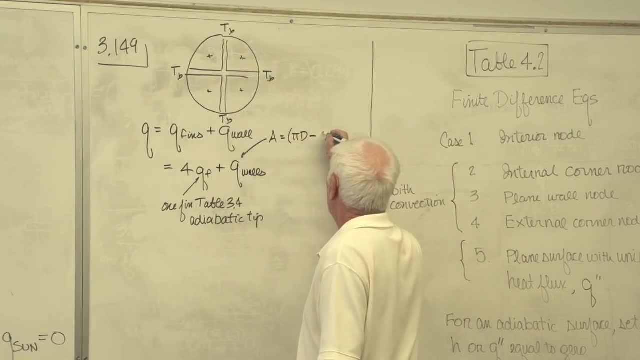 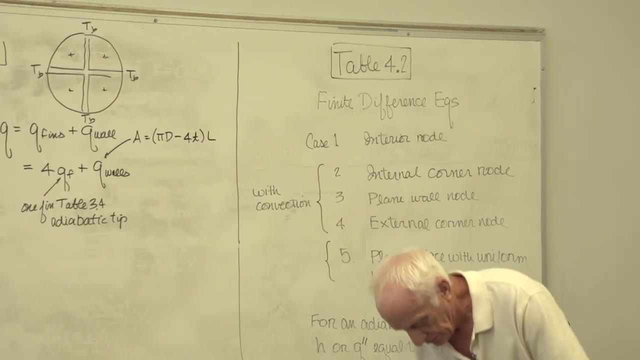 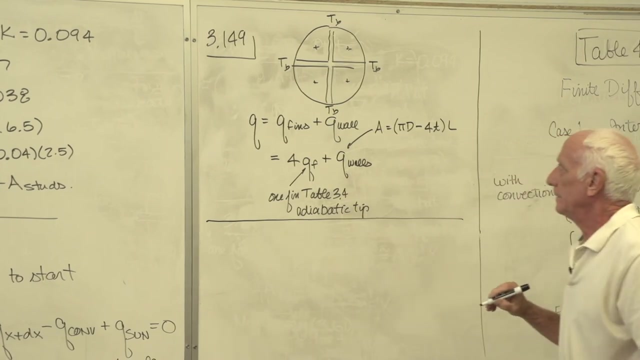 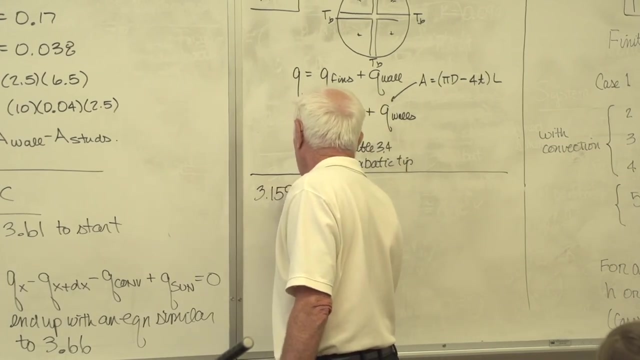 because that's not bare wall. The fins touching the wall there times the length, which is one. We're doing a per meter basis. So that's how you get that guy 3,158.. Any questions on him before I go on? 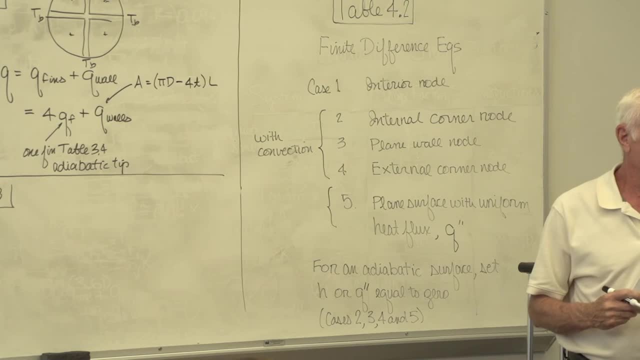 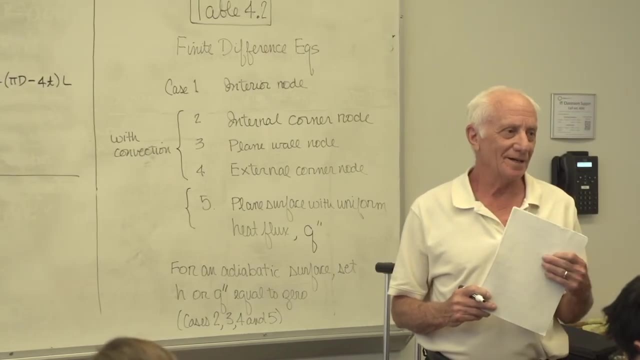 The length of the fins. just do the length of the surface touching the fluid right, not all the way to the center. Yeah, that's right, I would go to that. Yeah, I would go to that. Yeah, Because, like you say, 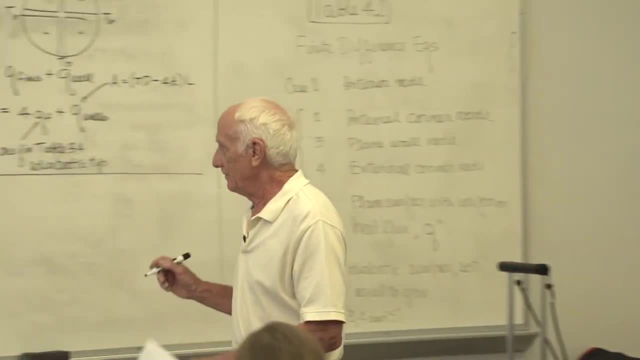 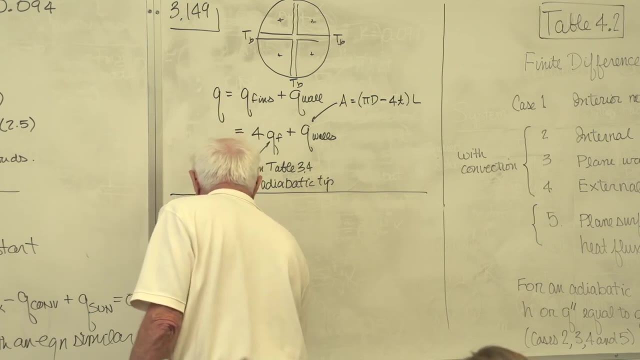 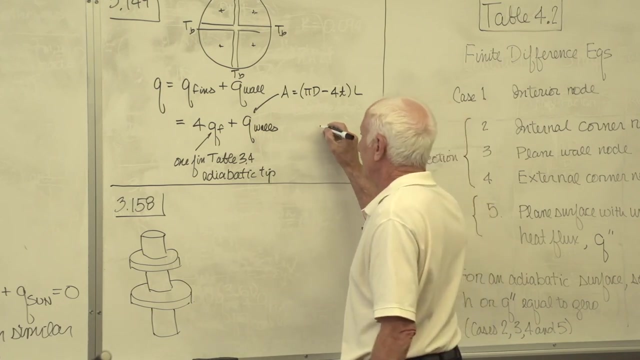 it's not touching the fluid area. 3,158 is this picture? Circumferential fins. Okay, By the way, on this problem here you don't need to find the fin efficiency. That's a waste of time on a timed exam. 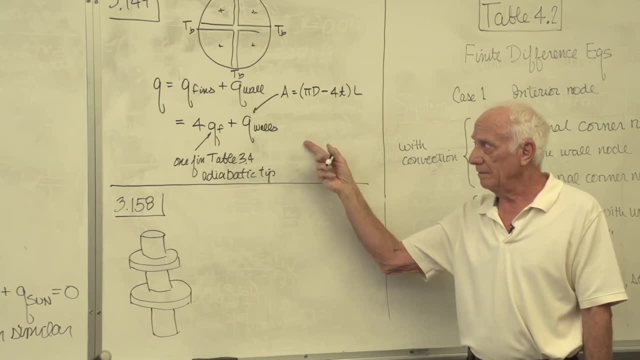 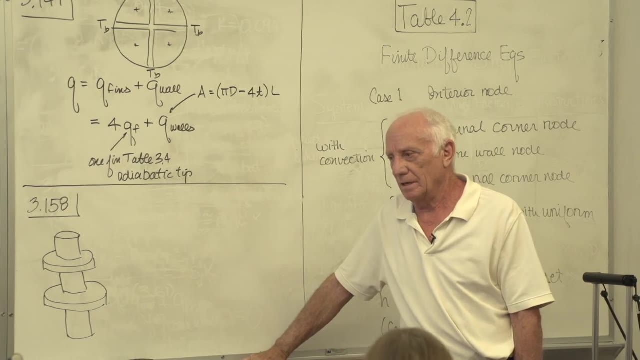 You can If you're asked for it. you sure can. But this is the easy way out because I know what Qf is: Capital M, hyperbolic, tangent, little ml. I get that really quick. But if you want to find the efficiency, 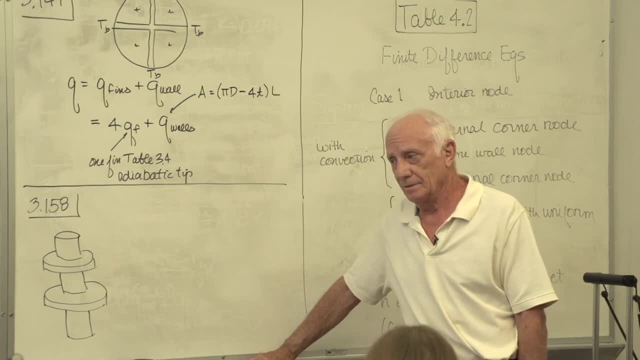 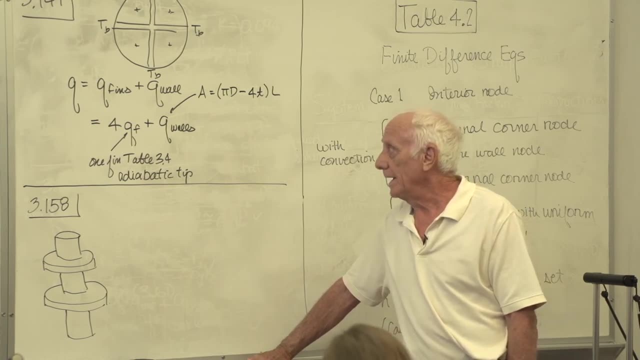 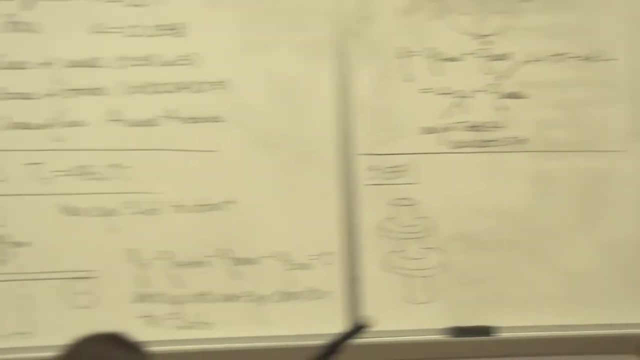 you can do it that way, It just takes more time. So, on this, exam time is valuable, real valuable, Come up Friday. Okay, This guy, Let's check how many fins there are on that That thing 158.. 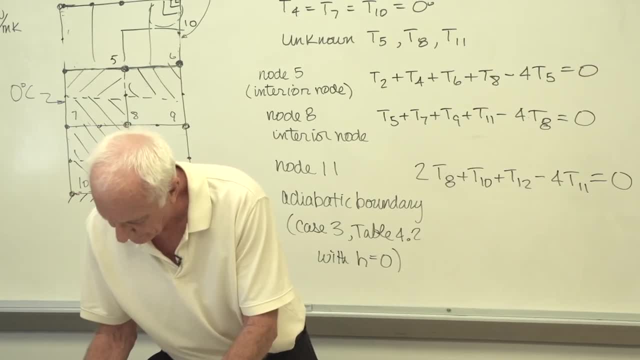 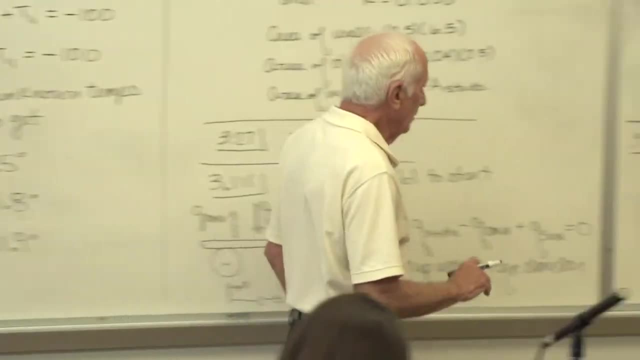 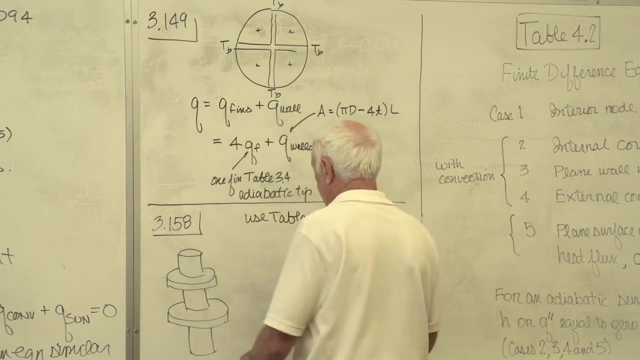 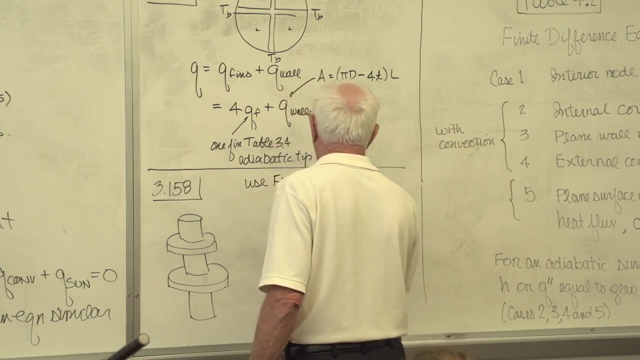 The first part says: find the heat loss by one fin. Okay, Got it. That's part A. Yeah, Heat loss per fin: 200 fins. So I'm going to use table a figure 3,320, to get eta fin. 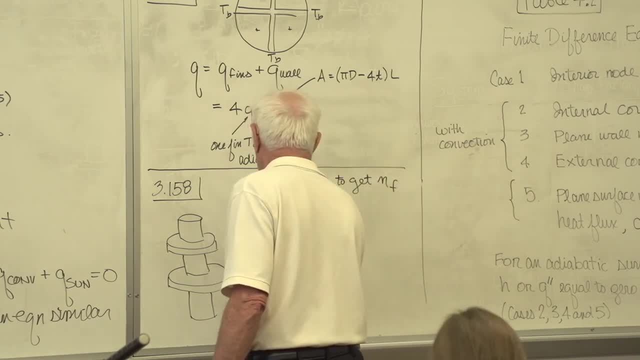 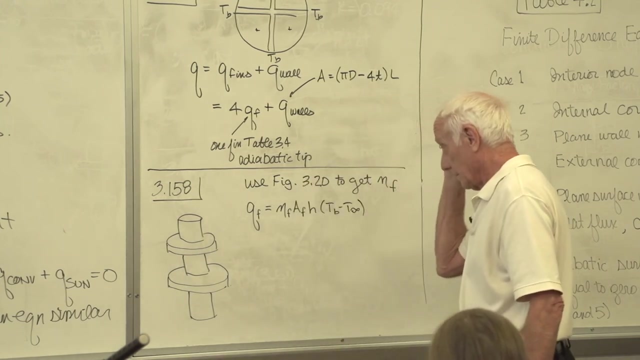 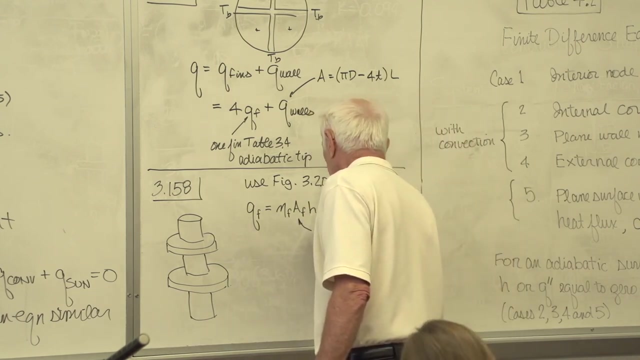 Then Q for one fin is equal to eta. area of the fin times: h, T base minus T infinity. The area of the fin there's top and bottom. So area of the fin is two because there's top and bottom Times, pi r squared minus the inside radius squared. 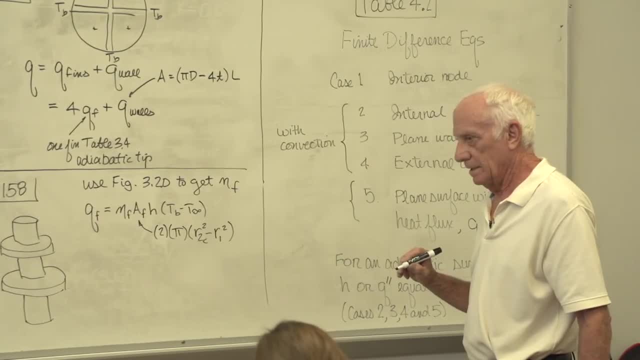 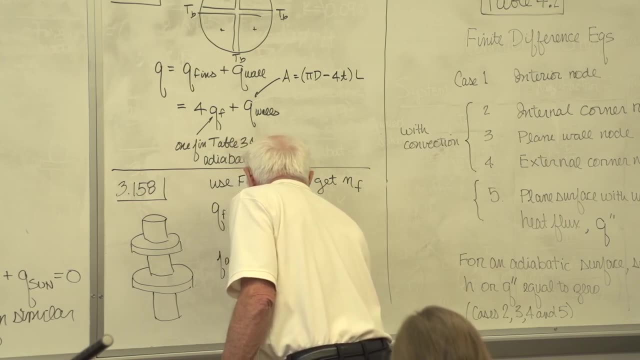 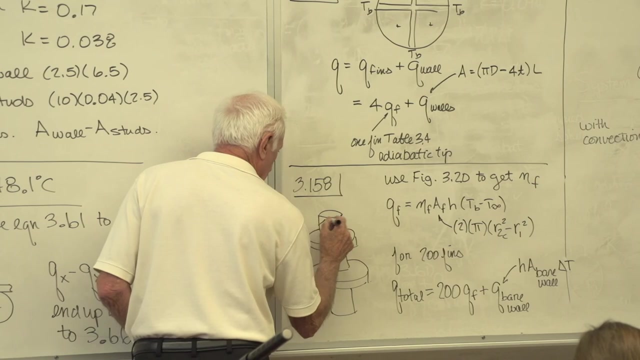 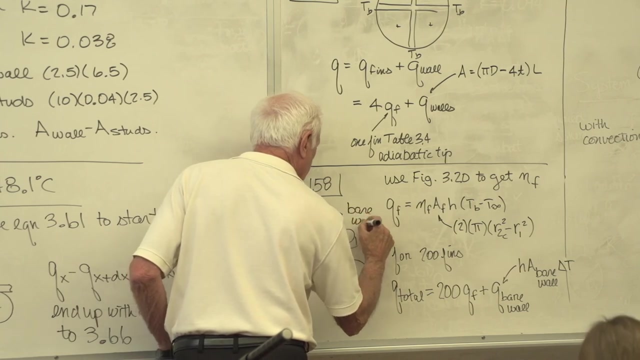 There's your area of the fin. For 200 fins, Q total equal 200 QF plus Q from the bare wall. So there's the bare wall. Now I'll show you the bare wall. Okay, That's the bare wall. 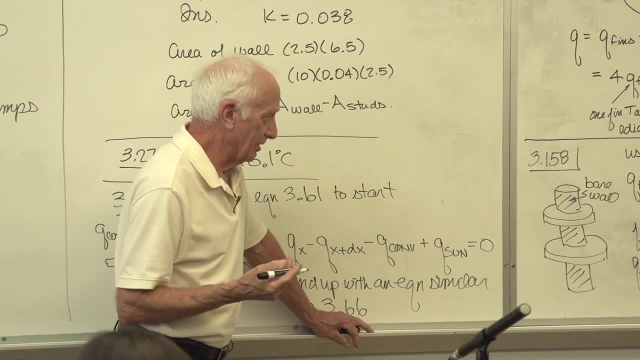 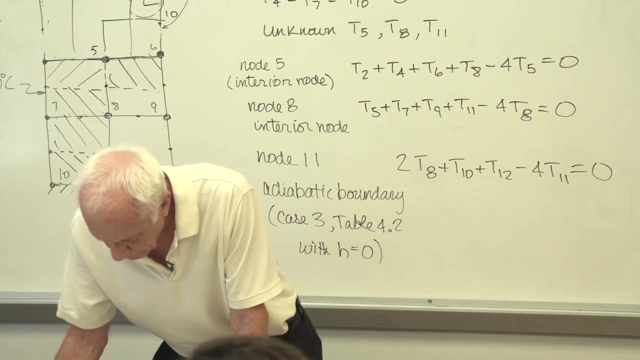 So how many spaces are there between the fins? 199.. If you want to do it that way, it's fine, But be careful. He says the fins are spaced at five millimeter increments. Boy, I told you in this chapter on the fins. 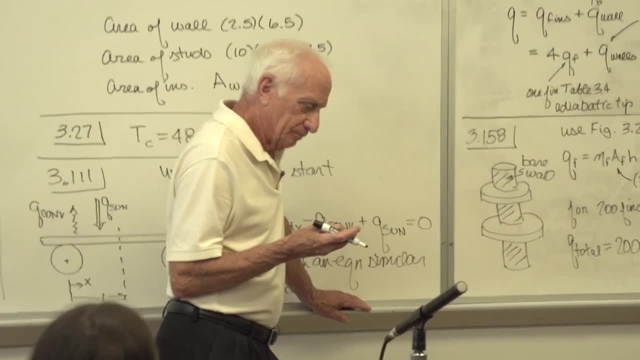 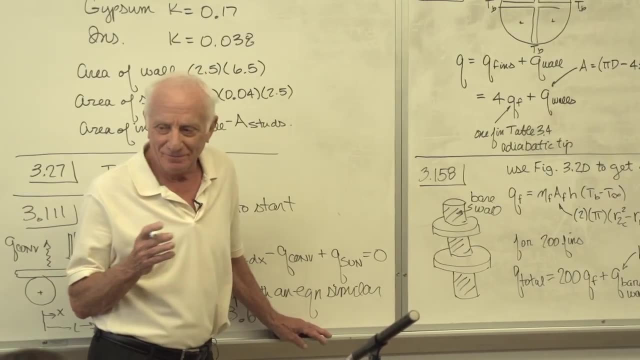 there's so many different areas. There's A sub C, there's A sub P, there's A sub F. You got to know that most people on fins make their mistakes on areas which should be the simplest thing of all, but they make their mistake on the areas. 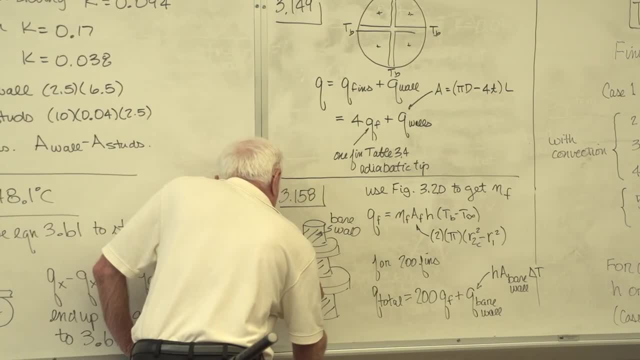 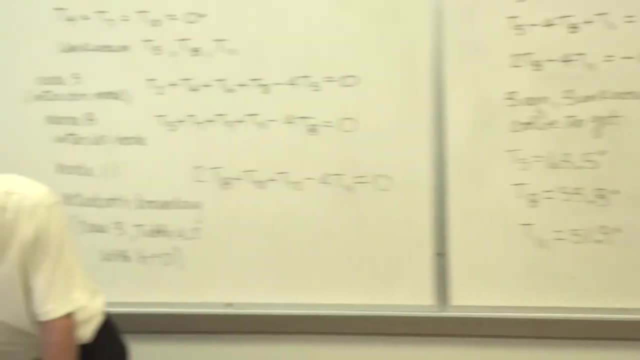 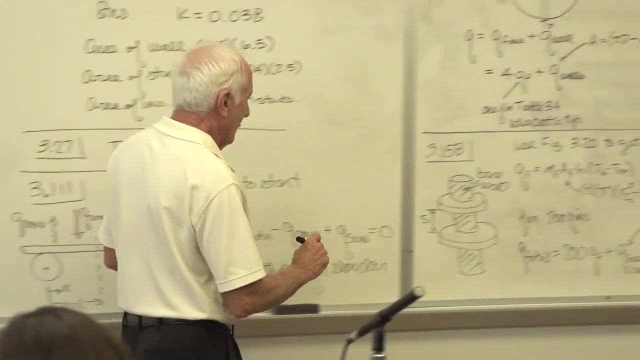 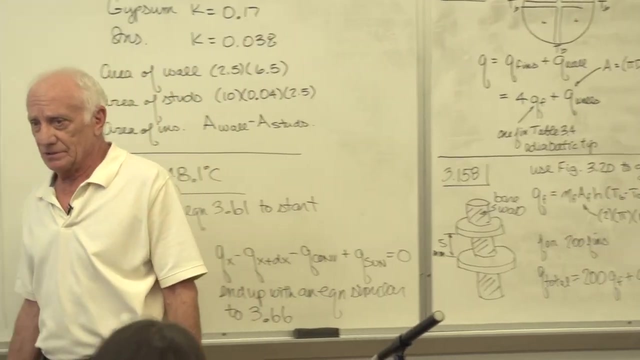 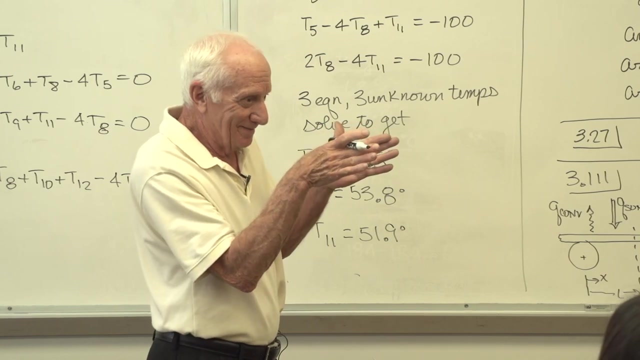 So the spacing of the fins five, Five millimeter increments Wall in your house. Somebody tells you the studs are 16 inches space at 16 inches. Does that mean there's 16 inches between this space and that face of the stud? 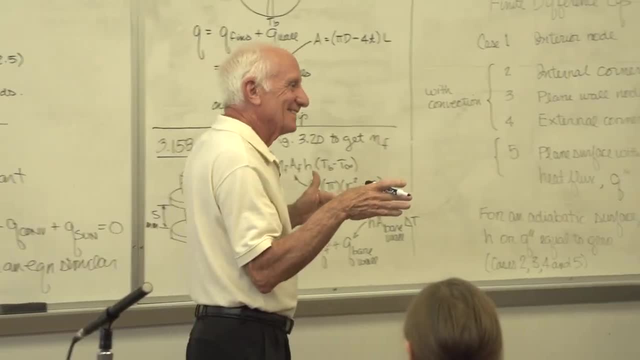 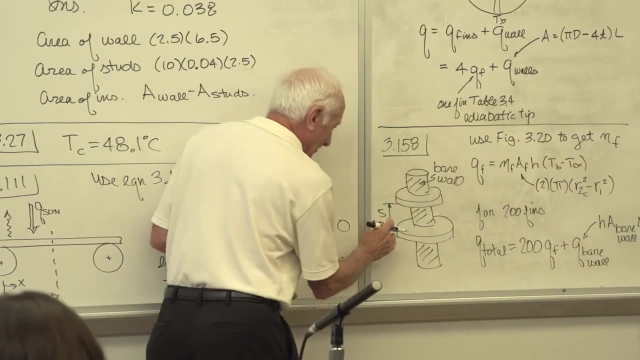 No, What's the correct way to say that? Center to center? right, Yeah, Center to center. So what does this mean? Five millimeters center to center? No, you got it wrong. Your area is wrong. It's from the middle to the middle. 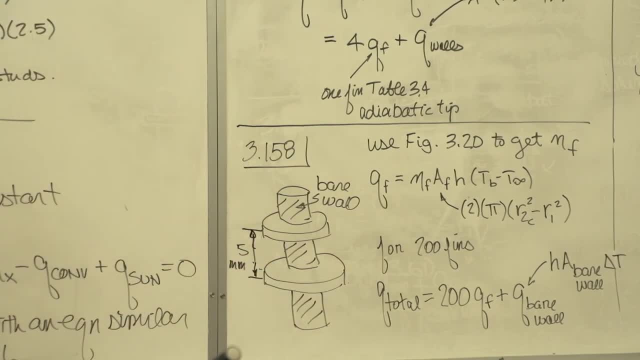 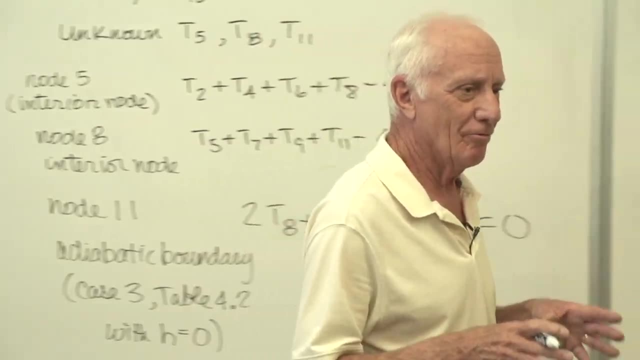 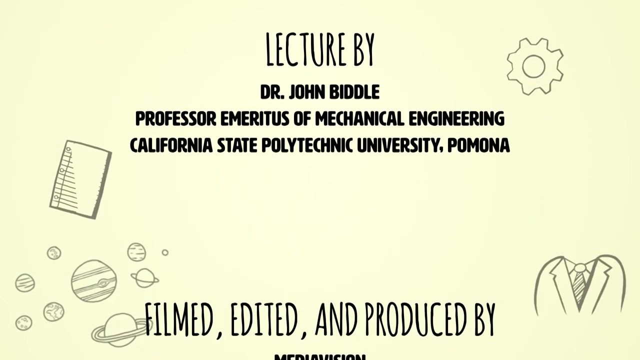 People make mistakes like that, which seems small, but when you multiply it by 199 spaces it becomes rather large. So get the areas correct on problems like that, All right. thanks a lot, Thanks, Thanks.